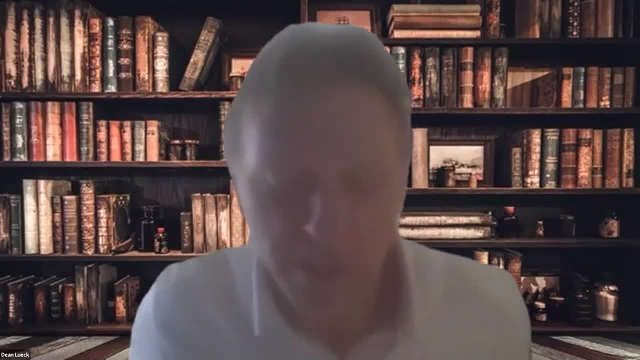 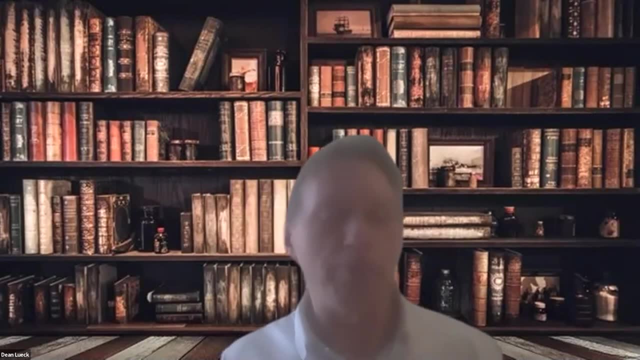 Before we get going, I just want to thank the workshop and staff for the support, especially Alison Sturgeon and David Price who made all the arrangements. We're going to plan for Peter to speak for 45 minutes. I think he's going to pop up some slides. 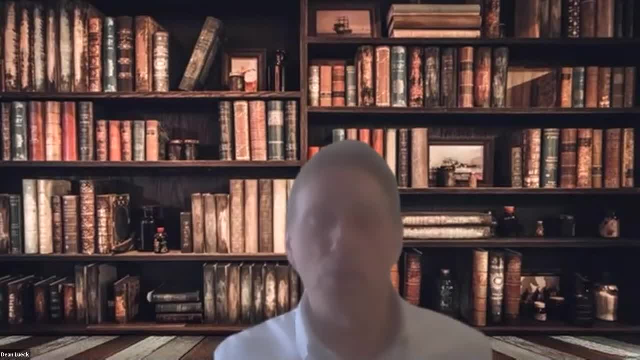 ordinarily we'd have this kind of nice reception, which we're not going to have, unfortunately. we'll keep the. we'll keep the um zoom open for a little bit. afterward. people can visit, uh, to extent that that's possible. um, the lecture is live streamed and it'll be available soon as a podcast. um, so 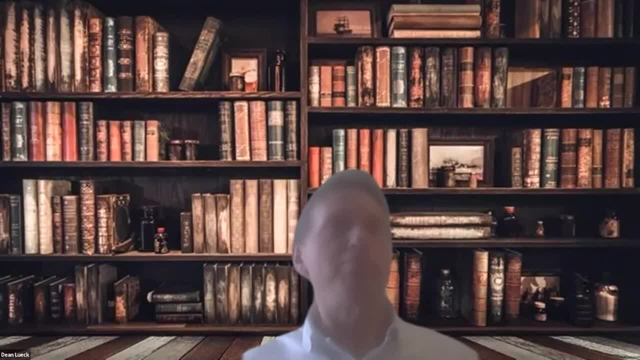 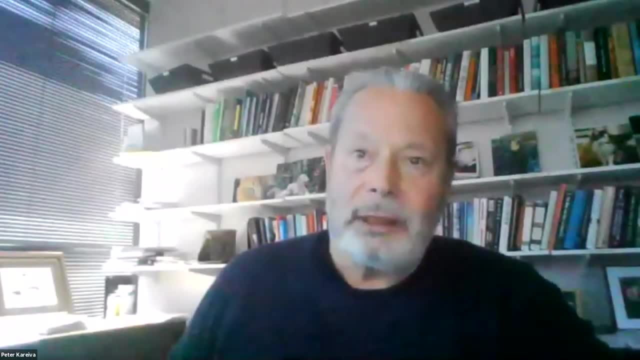 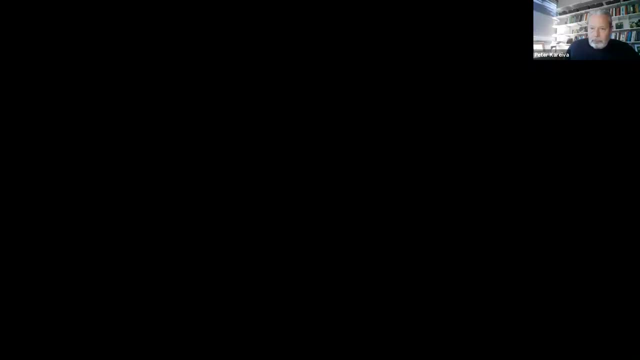 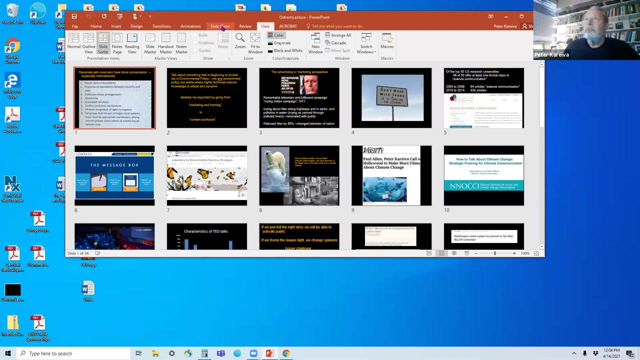 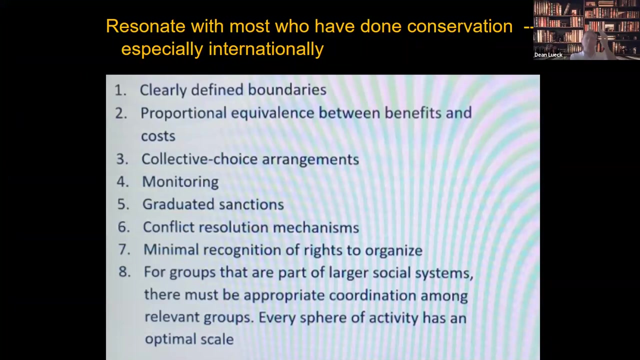 please join me in welcoming professor peter cariva. thank you, and i'm gonna share my screen now see if i can get going here. take the right one. so do you have that? yes, okay, great, well, you know being asked to, uh, you know, you know, you know. 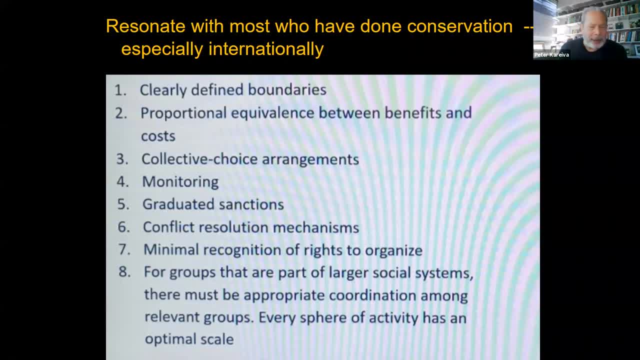 give an ostrom lecture- sort of like being asked to take a michael jordan jump shot or something it's. it's pretty daunting, but to give some perspective. most of my career i've been a sort of a practicing conservation biologist and worked a lot internationally and having done that, you know when ostrom's principles were published and and got attention. 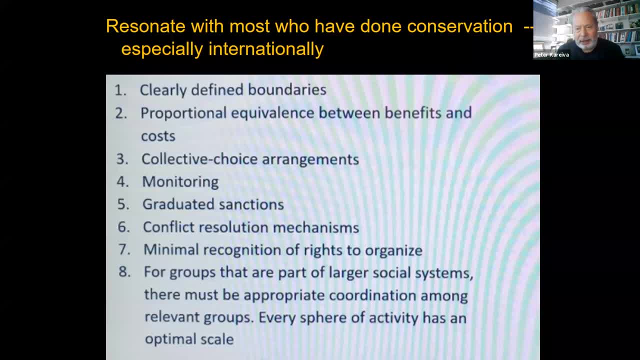 they really resonate with conservation biologists. at the time i was working on marine protected areas and marine conservation and they kind of they made sense. they made sense of just what i had seen in terms of what was what failed and what worked and uh it, you know, it's just. 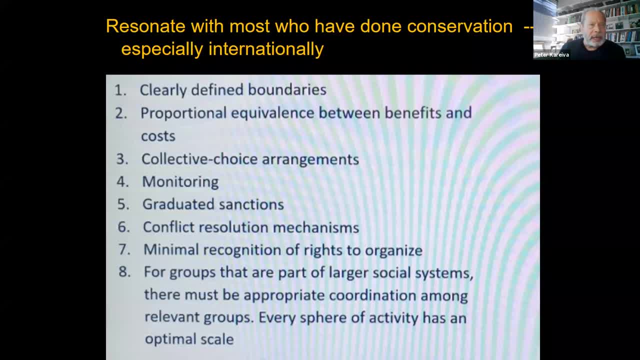 the, the insight into conservation biologists and conservation biologists and conservation biologists, and i think that conservation represented by these a principles is huge and i think, uh, now, most conservation organizations, when they plan projects, actually look to these at the beginning, instead of the way i did and looked to them after the fact. 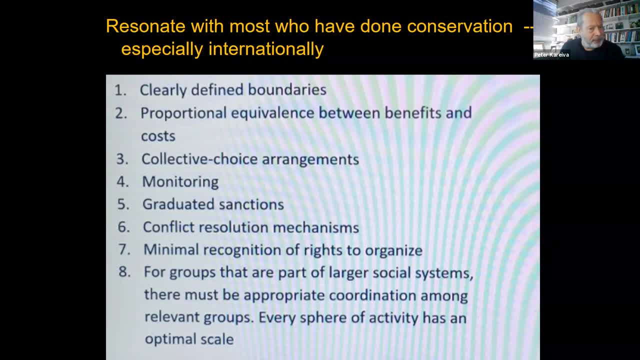 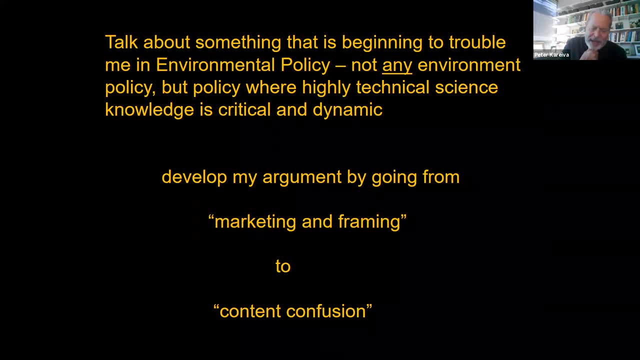 to explain success or failure. now we look to them to try to figure out how to succeed, and so what i, you know, sort of inspired me to look at the current environment to understand how the by that I want to talk about something that's troubling me in environmental policy. 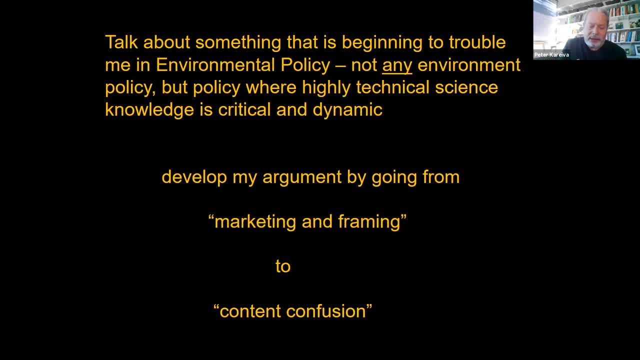 but it's not any environmental policy. I'm going to focus on policy where highly technical science, knowledge, is critical in its dynamic. You might have a policy for poverty alleviation and there could be social science done to collect data on the effectiveness of that policy. That's. 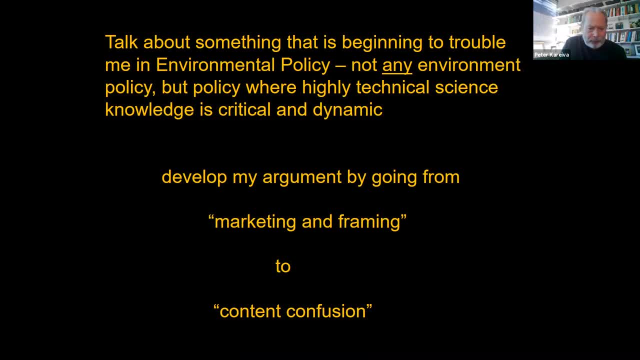 not what I'm speaking about here. I'm speaking about climate policy, geoengineering policy, policy where COVID COVID's a good example, policy where changing science knowledge and what that science knowledge is is critical to getting the policy right. So it's a 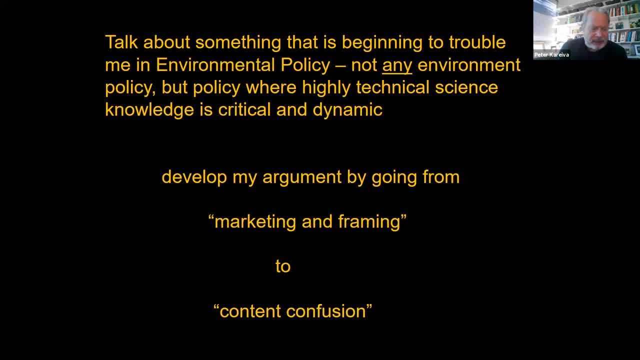 subset of environmental policy, And I'm going to kind of develop my argument or train of thought by starting with what seems kind of trivial and talking about marketing and framing, And I do that to distinguish it from what I want to really talk about, which is content confusion. 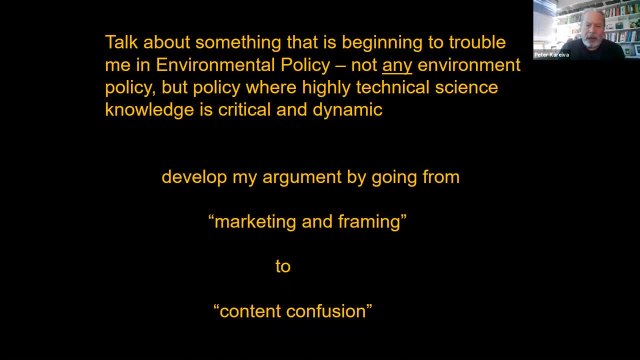 So I'll start with marketing and framing, because that's a form of communication. It's a form of communication about policy and science that I think everybody has contact with these days, And I want to set it apart from what I see as the real problem. 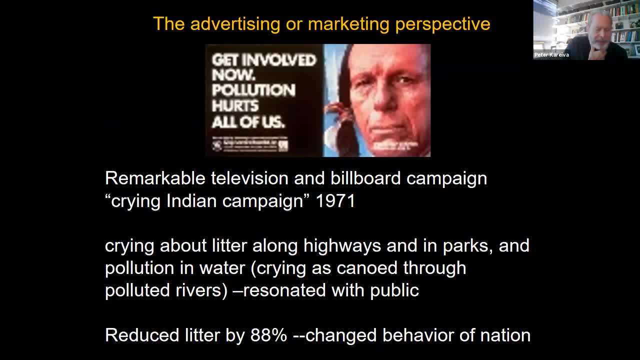 So let's start with sort of some of the most famous advertising and marketing campaigns. you know the environments. I've ever seen This billboard. some people may remember this. I'm old enough I remember it. There was a billboard campaign. 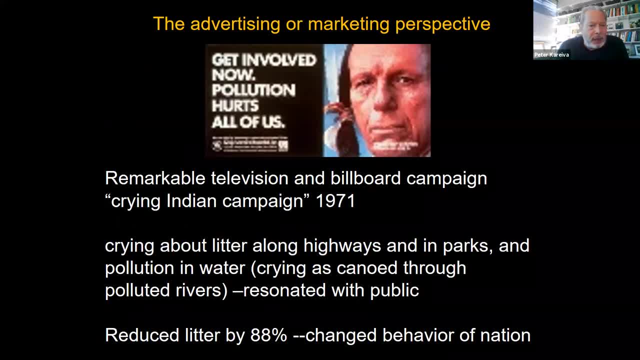 And there were also television commercials And it was, you know, crying Native Americans or a Native American in a canoe with a teardrop, And it was all about litter along the highways. It was astonishingly effective. In less than a year that campaign reduced litter by 88%. 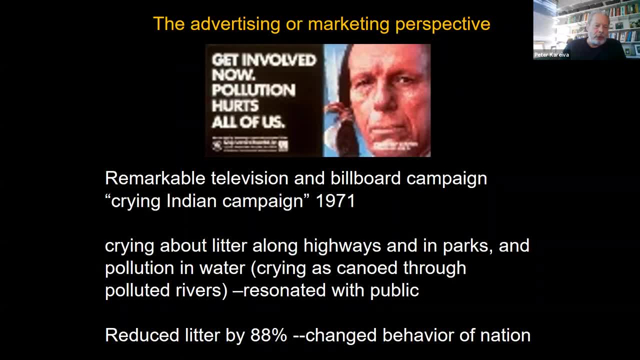 Madison Avenue and advertising agencies just sort of would study that to see like how did that work so well? It was a sort of fascinating marketing campaign to address. you know it's not a big environmental problem, but there used to be a lot of litter And one of the interesting twists on it and lessons. 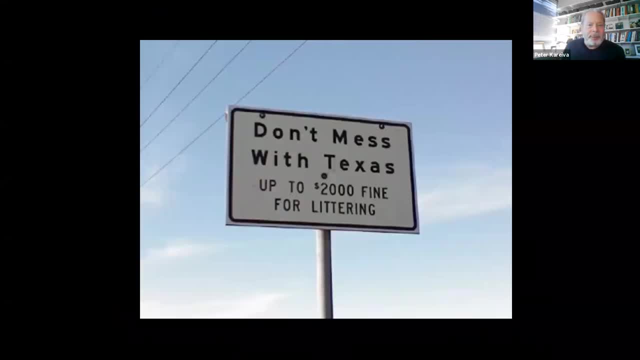 from it was a slight change made for Texas. This was Texas. So instead of you know doing the, you know crying Native American in a canoe. Texas's motto, as it tried to get with the litter, was: don't mess with Texas, which was: 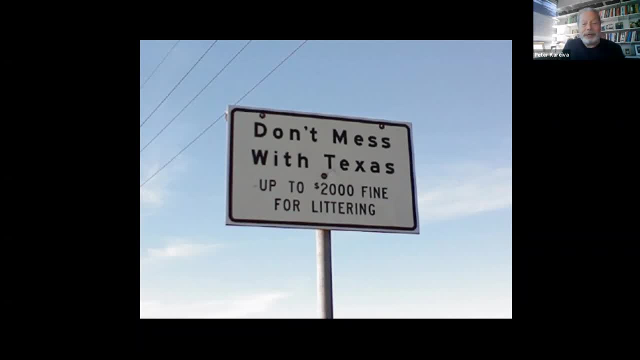 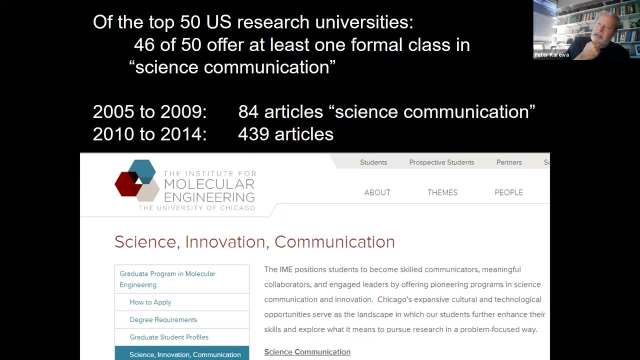 Texan cleverness. So now I may decide. maybe three years ago, but I bet you it's more. I think it's true that most universities now give classes in science communication graduate courses. So I did a search. I got the top ranked 50 US research universities- R1 research universities- and I went through their catalogs to see if they had graduate courses in science communication. 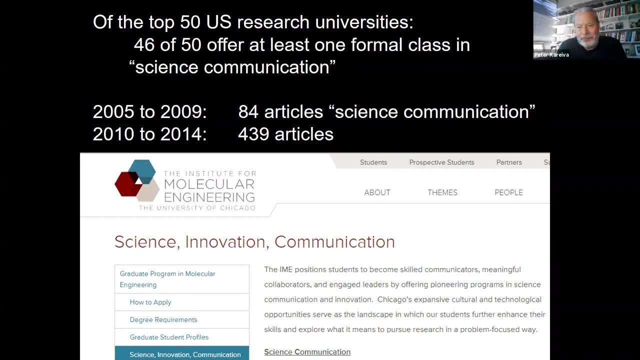 And invariably they did. Most had several courses That did not used to be the case. That is a relatively recent development. That if you're a scientist now you're told you- you know it's not just about publishing, it's not just about discovery. You got to learn how to be a good communicator to the general public and to the press and to media. 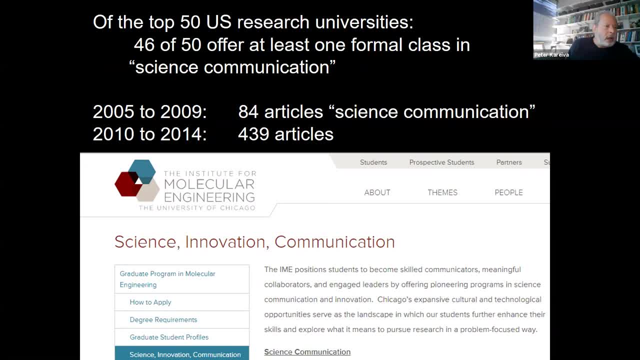 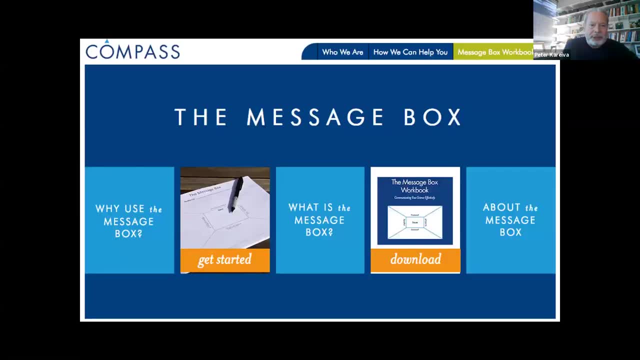 And it's really swept the nation. There's non-NGOs and all sorts of organizations that offer training. You may know. you know Compass Is one of them. in the environmental arena You get taught the message box And this type of communication training is. 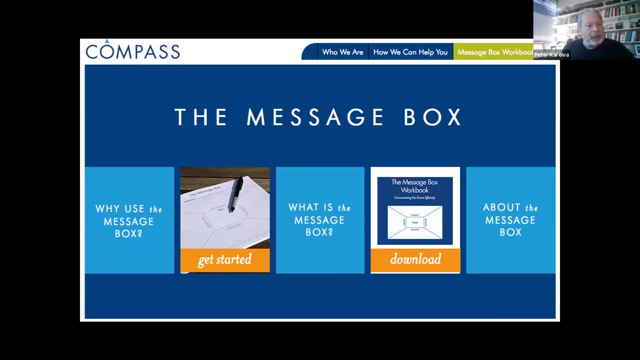 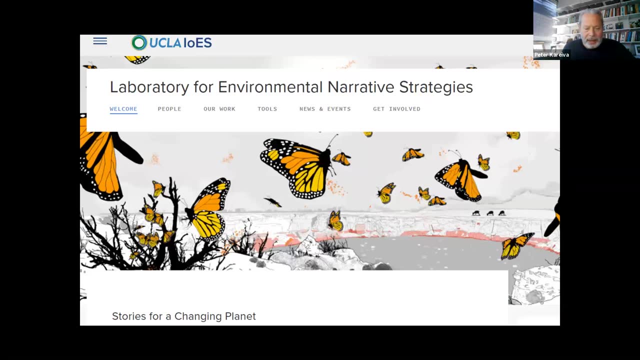 Is the standard now? I think it would be. I think it'd be hard pressed to get a PhD in environmental science or conservation and not go through some sort of formal Science communication training. And in fact when I was at UCLA, we created this thing we call the laboratory for environmental narrative strategies. That's just so we could call it Lens. 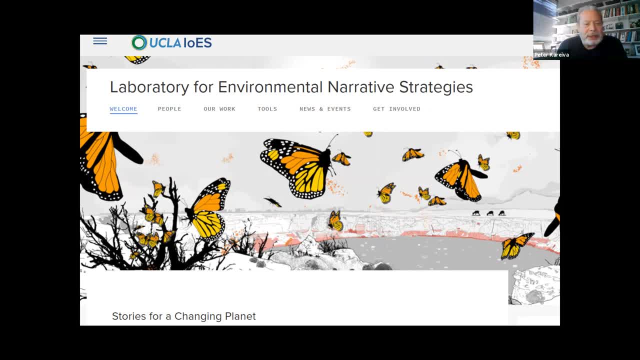 And we raised a lot of money for it. But the idea was clearly, you know, in This notion that somehow, if we told better stories, we would be more effective as scientists dealing with our planetary problems. We would be more effective as scientists dealing with our planetary problems. 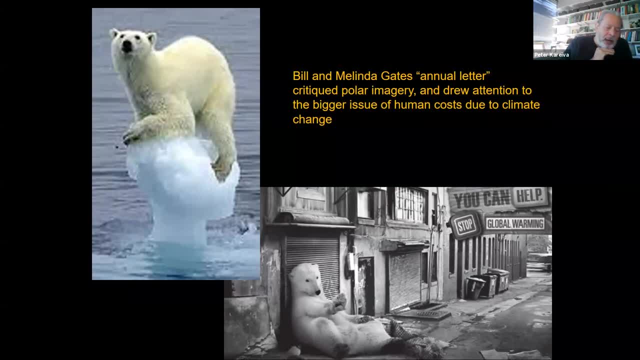 A really influential thing that happened. I don't think academia Noted this, but I was in DC at the time working for the Nature Conservancy and I can tell you WWF- all the major sort of conservation groups- noticed this. You know, Bill and Melinda Gates have an annual letter. Every year they write a letter and they talk about issues. 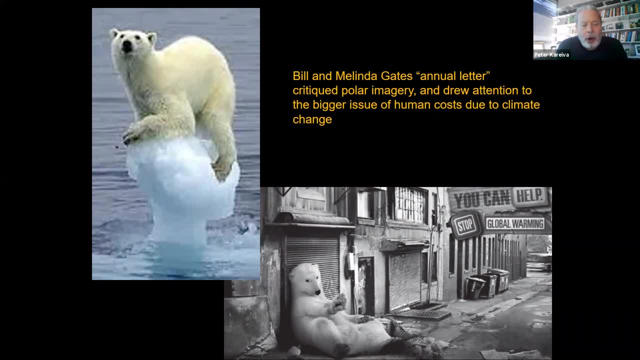 And they had an annual letter that, in an offhand way, it it. it wasn't really a sharp criticism, but it was. it was a mild rebuke of the conservation community for framing Global warming and climate change around polar bears And their point was their real point of the letter was to emphasize the impact of conservation. 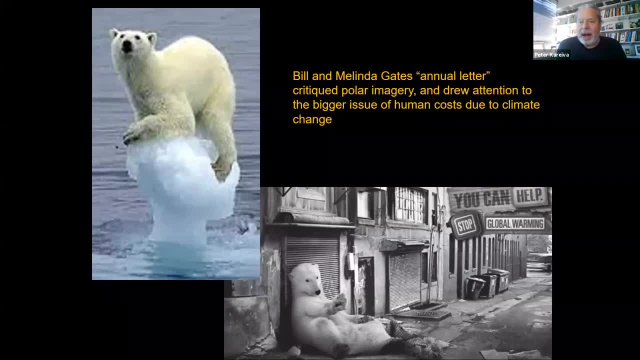 Climate change, on human health and poverty, And so it was really just one sentence About the sort of polar bear thing. But when you work for a nonprofit you pay attention to what the major philanthropists say, And it really struck folks that this went on, And in fact this is interesting. 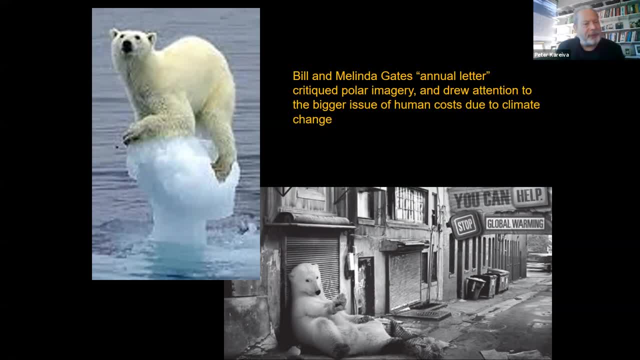 Twist on it. The first photograph up there In the upper left is really common in the environmental literature about global warming After the Melinda and Bill Gates. note the lower right polar bear. you notice what it evokes. It evokes a sense of home. you know homelessness. 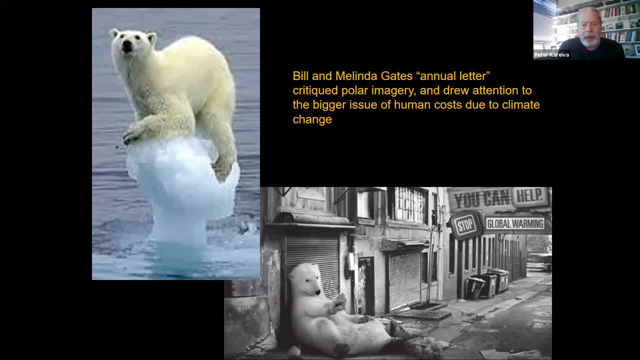 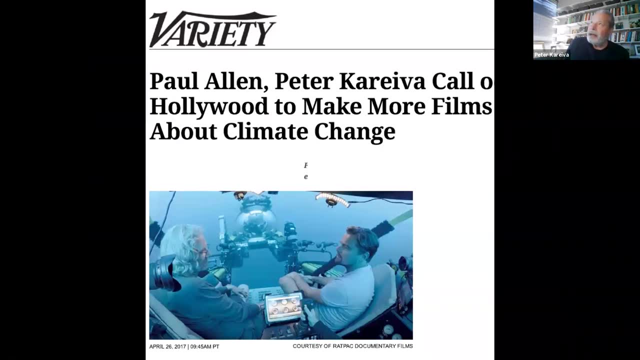 And is trying to strike a different chord. That's a WWF sort of poster about climate change And you know, you can. you see here that you know. believe me, you can be Bryno, because it's a littleètres haven't really been recorded in the United States. 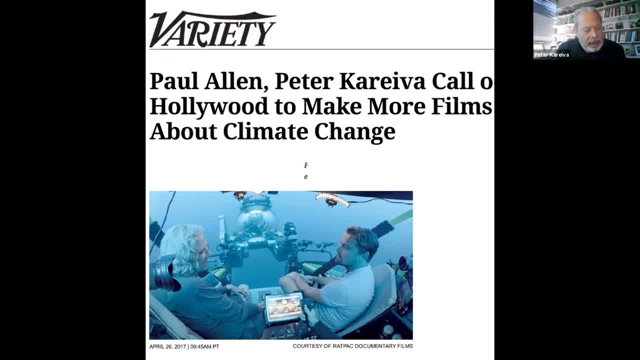 And you can color that history completely here. a little bit more than a thousand years ago- and this is- this is maybe my, you know, Most unusual publication- I wrote a, An editorial with Paul Allen in Variety magazine, And, and we challenge Hollywood. 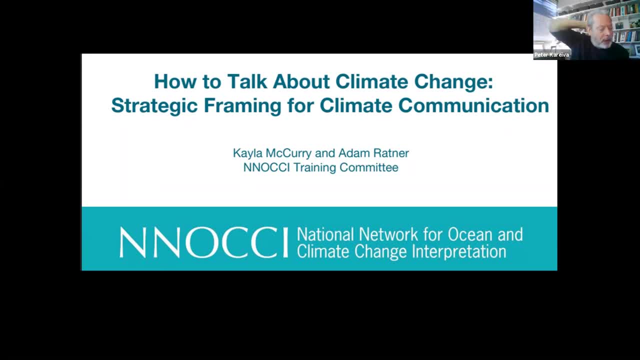 We called on Hollywood to make more films about climate Chief of climate change. become aware of aquariums and zoos. get more visitors than professional sports. You know this aquarium gets 2 million a year, not during COVID- And there are national science foundations funded programs that address the idea of how. 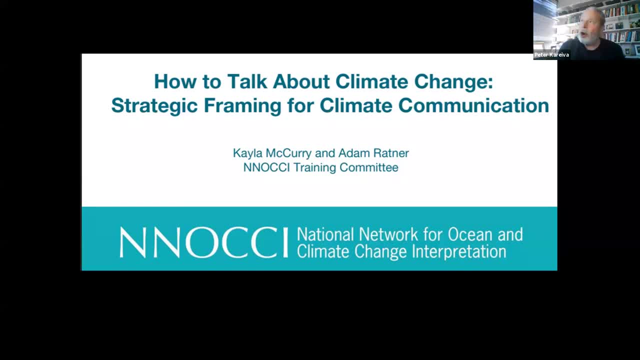 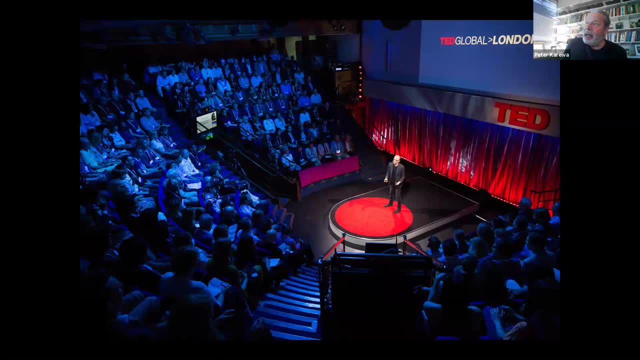 should aquariums and zoos, where they have direct contact with the public, talk about climate change And there's organizations for it? And lastly, we all know about TED Talks and how influential they are, And if you teach, you know your students have watched TED Talks. 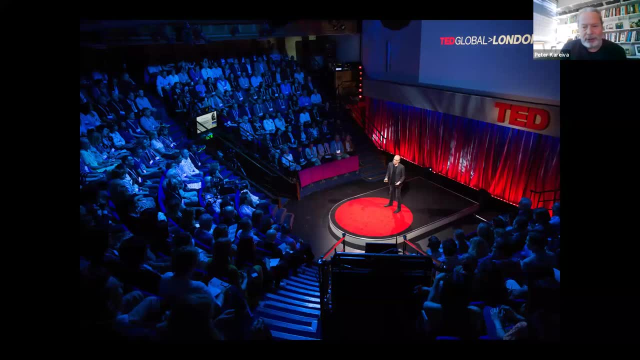 And when you work for a nonprofit, your board members have watched. One of the interesting things about TED Talks is they're one of the ways you know the wealthy and influential. imagine that they keep up with the issues And they're fun and they go to them. 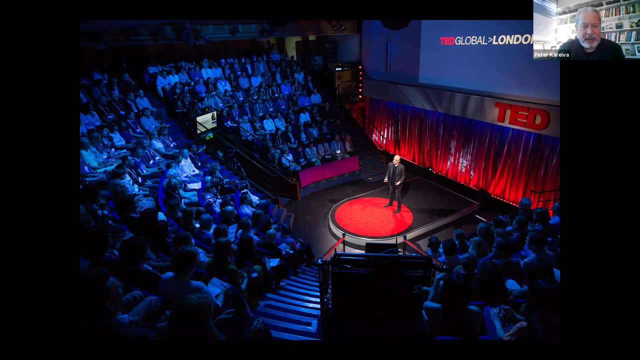 And so many times somebody would come up to me and say: did you see this TED Talk? Is this really a good approach to climate change? Or did you see this TED Talk, And is this really happening in fisheries? It's become a very, very prominent form of communication. 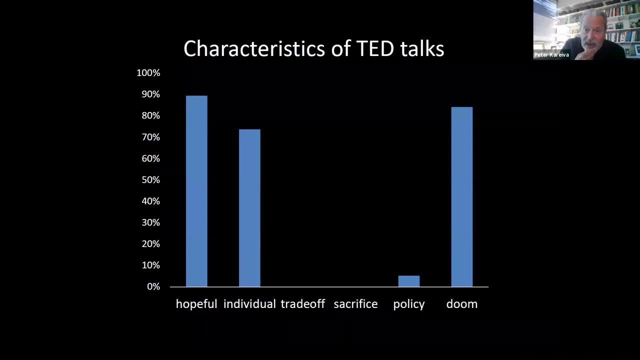 I did this, I became sort of frustrated with TED Talks So I did a little analysis where maybe my filter was wrong. TED Talks are very well curated, So you can search by subject area and then by who gave them, And my criteria was they had to be about environmental problems. 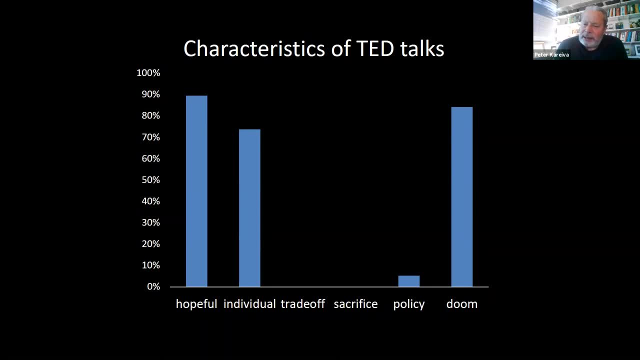 And they had to be about by PhD scientists Because I figured if they were by activists or authors of a popular book. they have different motives, But I thought you know, scientists talking about environmental issues, you know, let's see what they bring up. 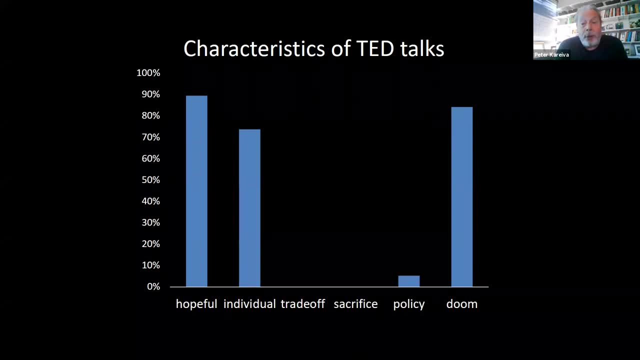 The striking thing about TED Talks is policies almost never discussed By those scientists. Neither are trade-offs or sacrifice. Essentially, the model of a TED Talk if you're a scientist is: oh my God, there's doom on the horizon. 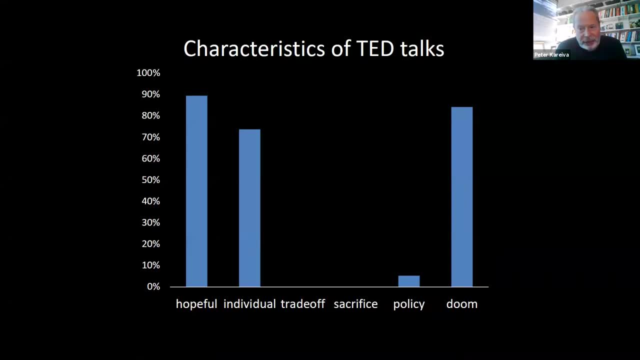 I've discovered something. It could be a technology or it could be composting. I've discovered something And you, the individual, if you get this technology, support it or do composting, can make a difference And you can do it. 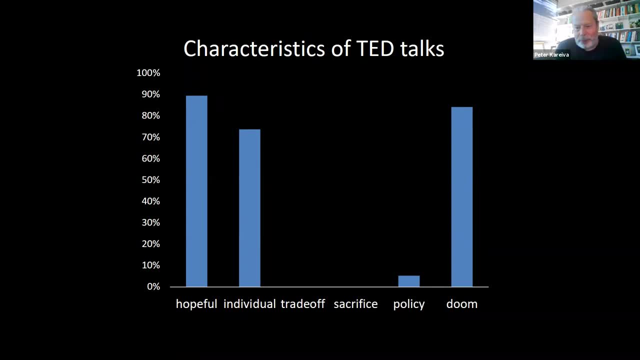 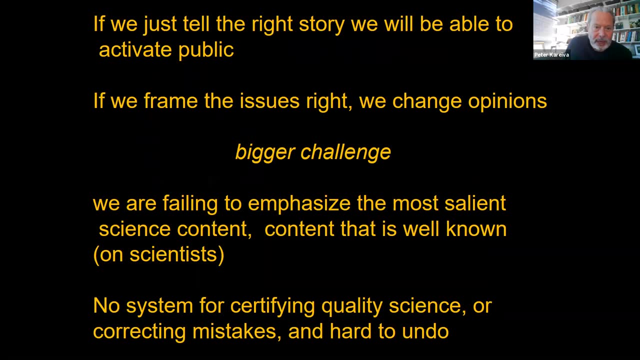 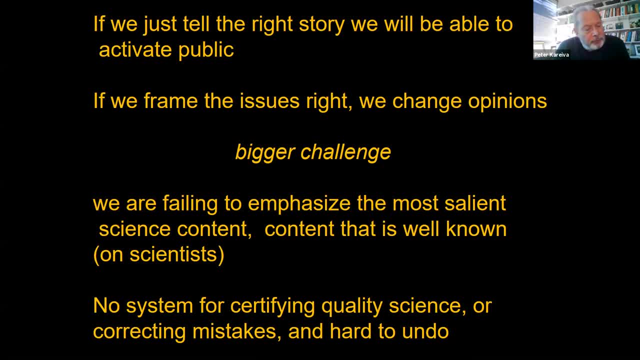 even in NGOs And at research universities related to environmental problems. And it's basically these two ideas. It's like if we just tell the right story we'll be able to activate the public, Or if we frame the issues right, we could change opinions. 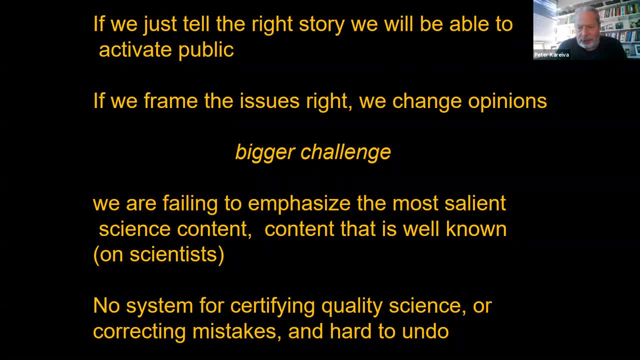 You know, like Lakoff's work out of Berkeley in the Frameworks Institute, Just reframe the problem. But I think the bigger challenge And the real substantive challenge is what I want to really finish talking about. So the right story and framing, I call those style. 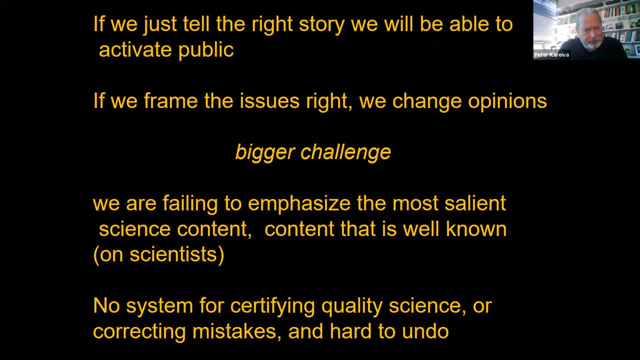 And these bigger challenges I call substance and content, And I think the things that we're failing to address when we talk about science, communication and environmental policy is: are we picking the right science to talk about? I mean, it's not how we talk about the science content. 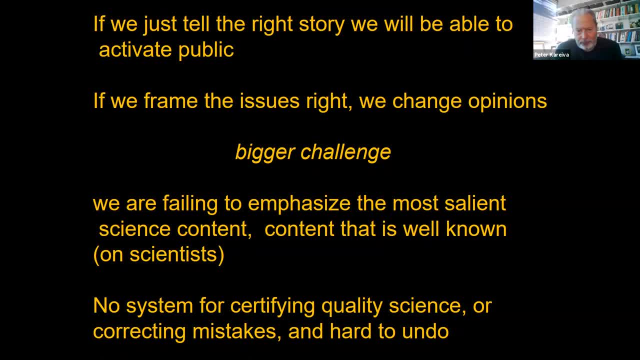 It's: what science content do we talk about? And that decision is really on scientists to get better at. And the second challenge- and this is sort of like some of Eleanor Ostrom's issues of descriptions of what is needed for good resource management- 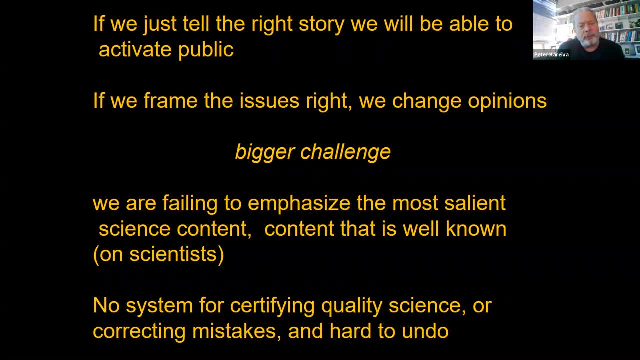 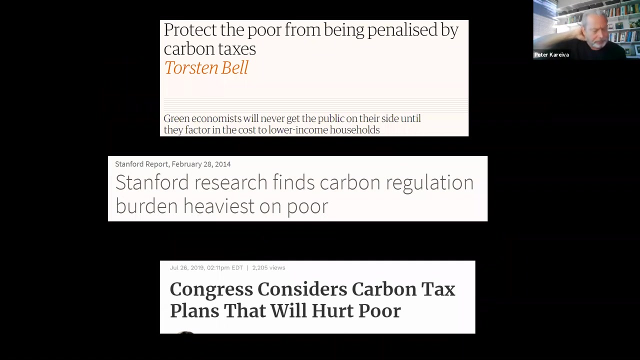 In this arena we have no system for certifying quality science or for correcting mistakes to get published, And once they're out there they're really hard to undo and they have lasting impact. So, as a transition sort of between the content and the messaging, 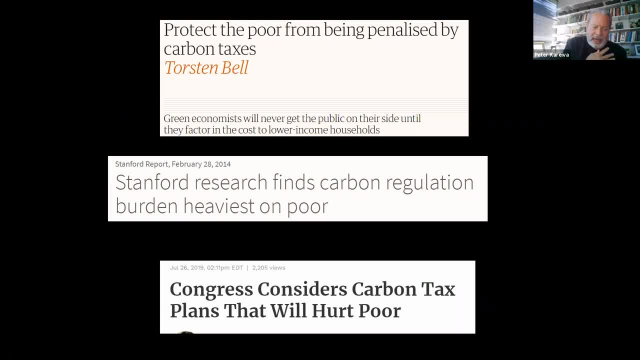 I thought that there's kind of an intermediate example which is discussing carbon tax. So there have been a number of studies and a lot of articles that have talked about carbon taxes from the point of view: will they hurt the poor? There's even been legal suits. 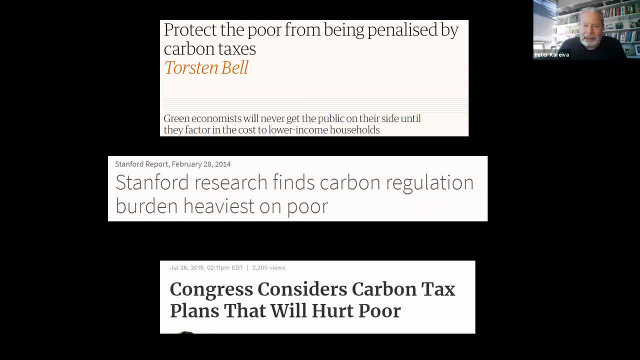 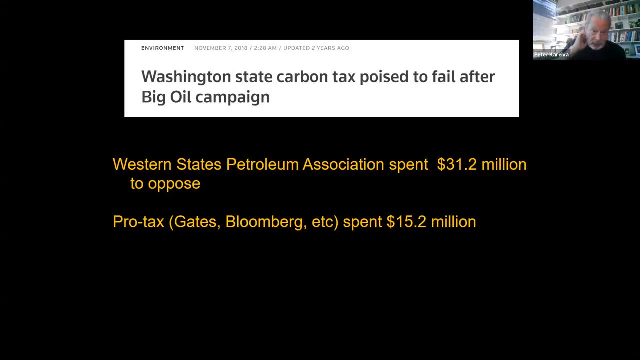 from Miami minority communities that they're biased And in terms of who gets penalized. well, in the most recent state ballot on carbon taxes that was in the Washington state carbon tax ballot measure in 2018, got a lot of national attention. 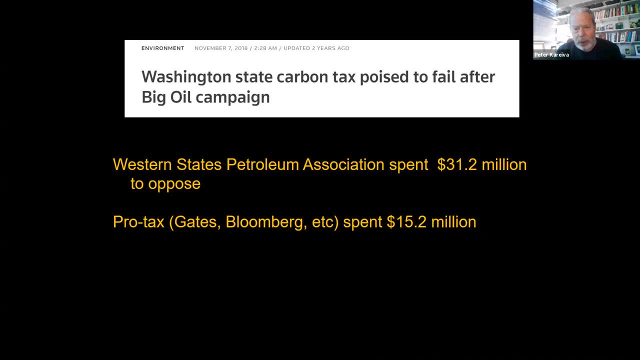 It would have been the first straightforward carbon tax, but it didn't get a lot of attention in the United States And it was a lot of money that was spent on it And a lot of the discussion was about how you deal with underserved communities and the poor. 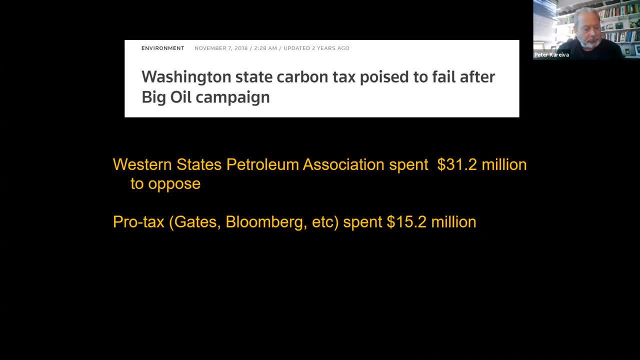 And you basically had the Western State Petroleum Association versus a pro-tax and Bill Gates funded was in favor of the carbon tax. Bloomberg was. a lot of money was spent more by the federal government than by the federal government, And so there was a lot of discussion about how you deal with underserved communities. 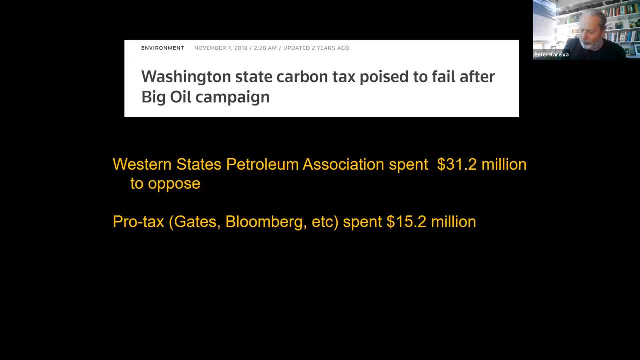 And I think that's a good example of how you deal with underserved communities. And I think that's a good example of how you deal with underserved communities More by the oil. And I might pause here and say: how do you think the votes turned out? 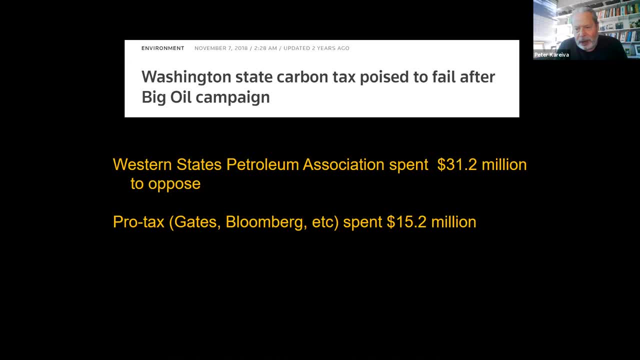 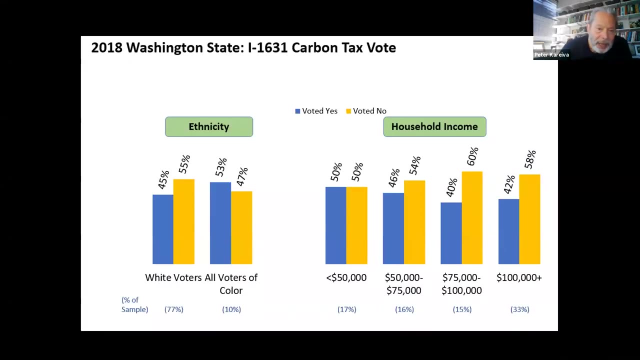 in terms of race or ethnicity, for the carbon tax or income. You might just guess in your head. how do you think the votes turned out? And this was a surprise to people- It turned out that here no is the yellow and yes is the blue. 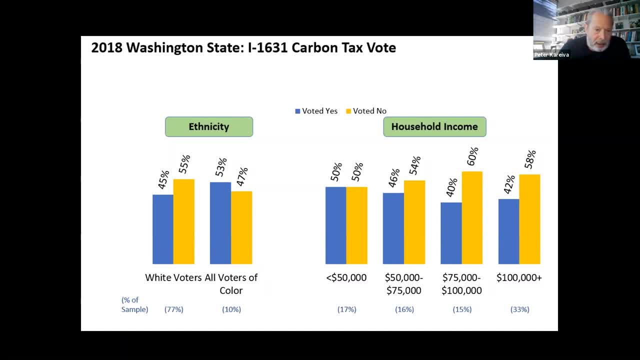 blue And for white voters: 55% voted no, 45% voted yes. For voters of color, it was the reverse And in fact the tendency was the less your income, the more likely you were to vote for the carbon tax. The graph on the right is income And you see, when you get over 100,000, you have. 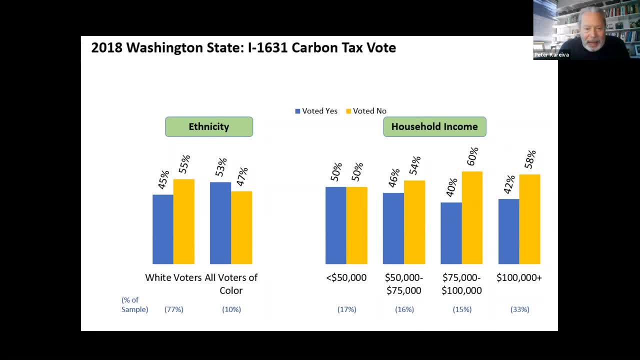 58% voting against it, And when you're less than 50,000, it's a split 50-50.. These data were a shock to people, I mean. they had totally kind of misunderstood that this was a really 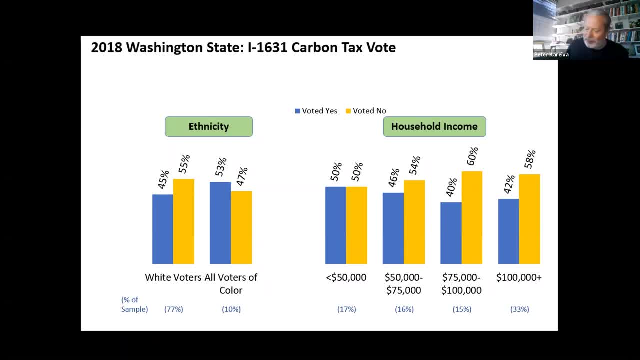 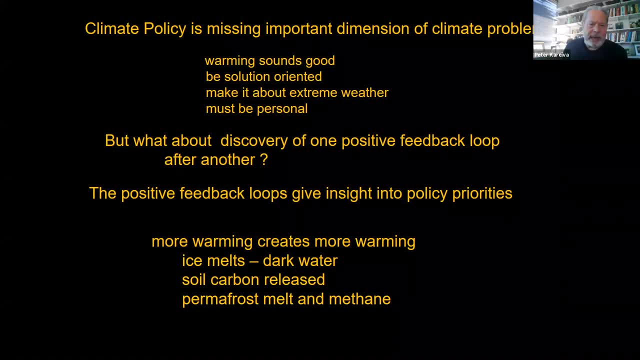 really surprising result for a carbon tax vote, And it's because assumptions were made. Assumptions were made without any data. If anybody wants that data, I'm glad to share it with you. So here's the substantive thing. So I think there are so many papers and studies. 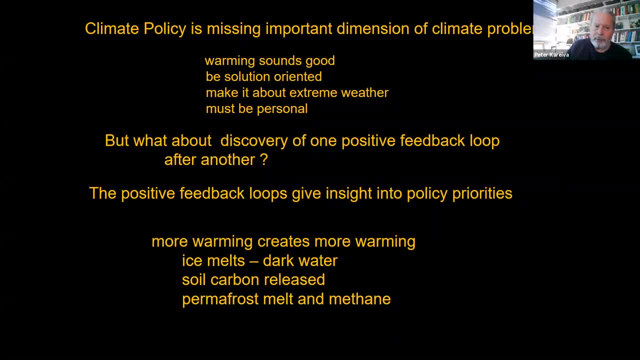 about climate communication, And these are the things that they tell you. They tell you. you know we made a mistake by calling it global warming, because some people think that warming it feels good- Probably feels good to you guys in the winter. 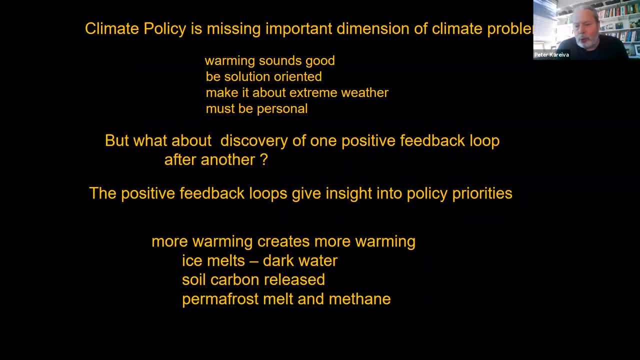 Well, we have to be solution-oriented. We can't be so doom and gloom. Environmentalists are always so doom and gloom. There's a famous quote that you know: if Martin Luther King had been an environmentalist, he wouldn't have given. 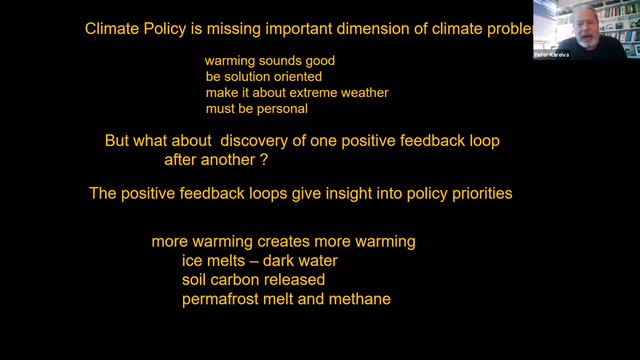 I have a dream speech He would have given. I have a nightmare speech. Oh, we have to make it about extreme weather. Don't talk about global warming. focus on extreme weather, The other thing that there's lots of these articles about. 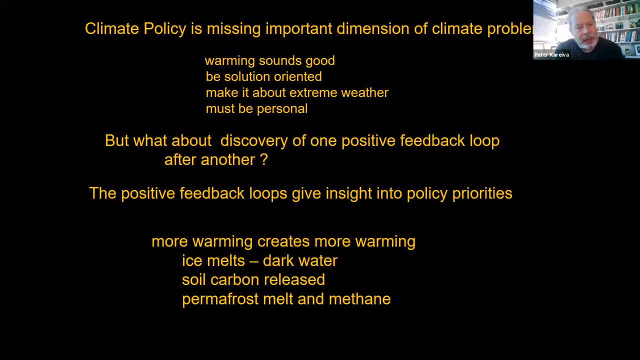 make it personal, You know, identify what's going on in your backyard And you know those are all probably helpful. but I think the whole climate discussion has missed some really important science content And they've failed to connect two dots. The first dot is we're discovering. 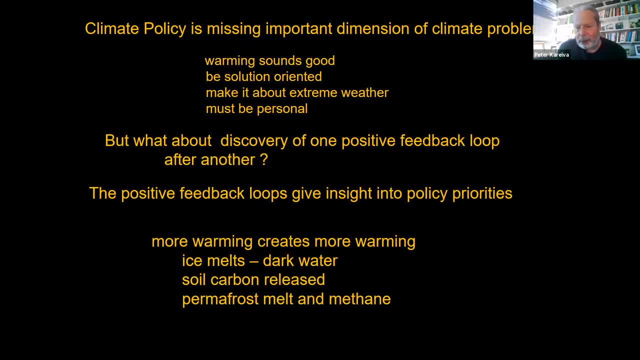 one positive feedback loop after another. Maybe a year ago there was a review article in Nature. I haven't listed them all here- but a positive feedback loop means that you have warming and you get more warming, So ice melts, leaving dark water, which is absorbs heat, which makes it warmer. 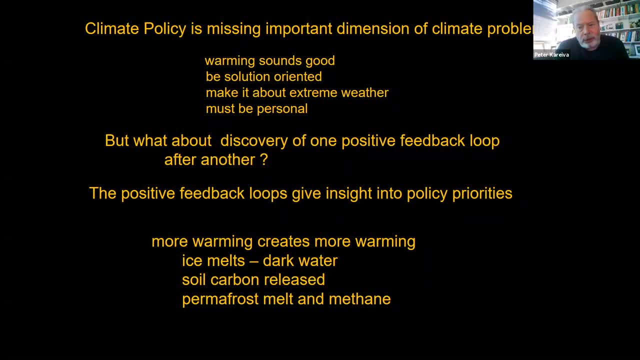 which makes ice melt, more Soil carbon is released, which warms the soil, which and releases CO2, which further warms the soil and releases more CO2.. Permafrost melts releases methane, which causes more warming, which causes more permafrost. 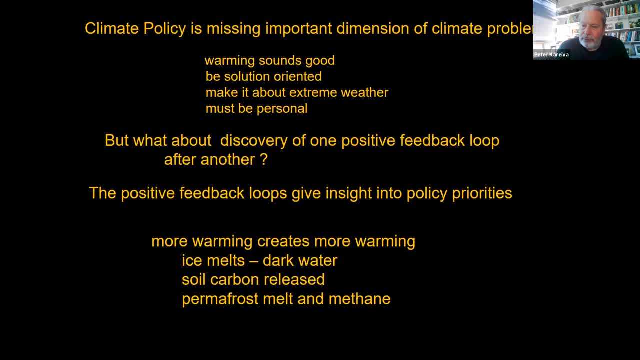 melting and more methane, And I could make a long table of these positive feedback loops. You don't hear these talked about much. I mean, when people think about global warming and CO2, I think too often they think about it like any other pollution, like maybe DDT or mercury. 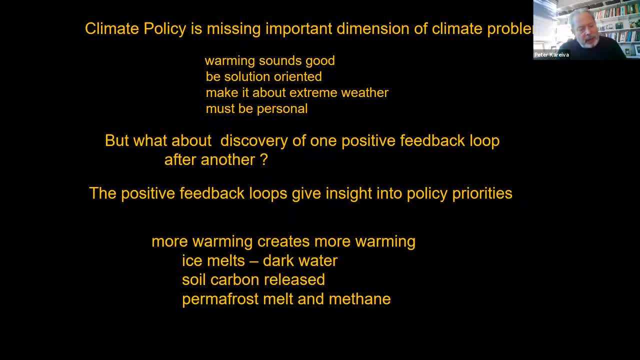 where you add it And yeah, it's added. but the fact that you add it doesn't mean that you inevitably add more in the next time. step. A positive feedback loop is a special kind of phenomenon and it's really important. It's a really significant feature of the climate challenge and it's well known. 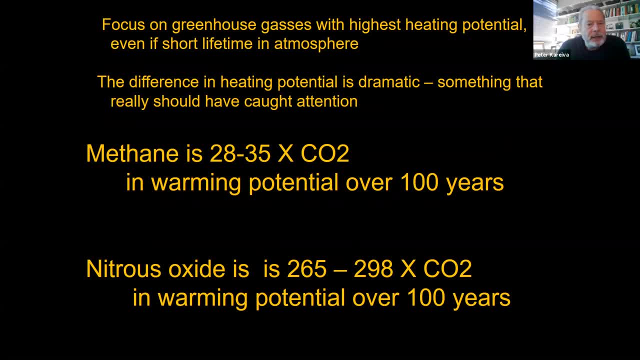 And the other thing that's well known is the different warming potential of different greenhouse gases. So you know it's changing now. I mean it's just changed within the last year or two, But for the longest time we've only talked about CO2.. And the reason is because CO2 stays in the 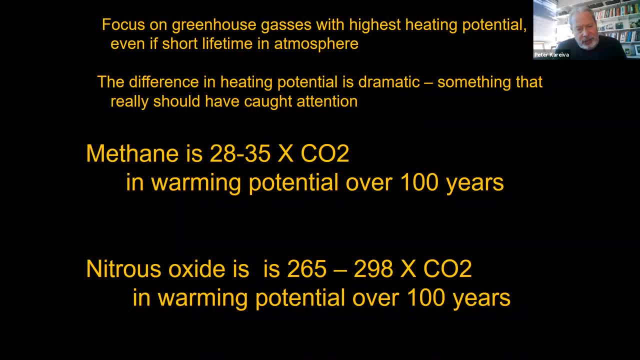 atmosphere for so long and these other greenhouse gases have a short lifespan And there's a standard metric that's used. It's called warming potential over 100 years. So methane per unit methane has 28 to 35 times the warming potential of CO2 over 100 years. 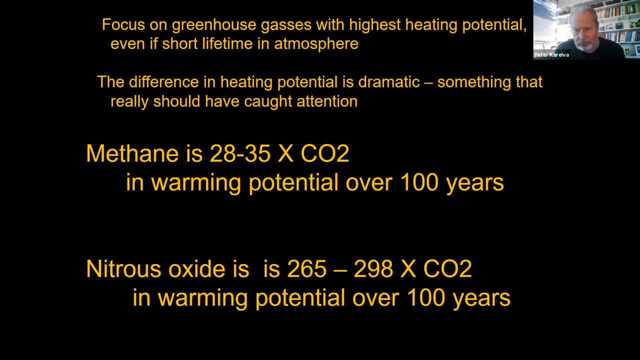 It's just that methane doesn't stay up in the atmosphere that long, whereas CO2 is up there for thousands. Nitrous oxide comes from fertilizer production and a lot of industrial activity. Nitrous oxide it's 265 to 298 times warming potential. 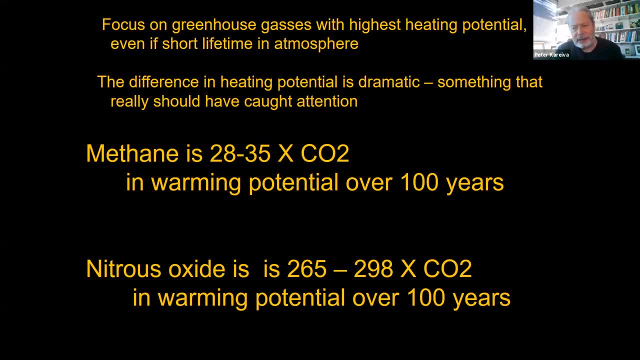 Nitrous oxide, it's 265 to 298 times warming potential of CO2 over 100 years. Now, these two facts- positive feedback loops and enormous warming potential over 100 years- are to me two of the most important science insights or understandings about climate change there are, and somehow it's escaped. 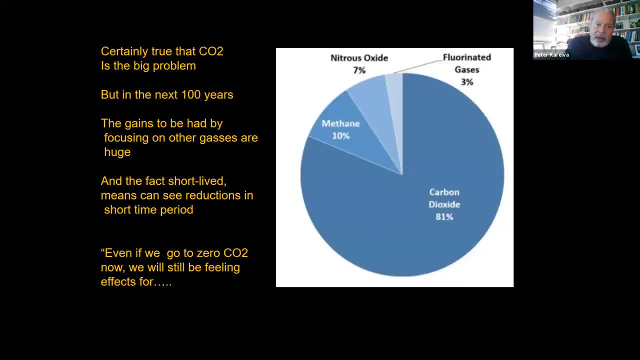 The narrative and it's escaped the policy. And it's certainly CO2 is the big problem, There's no question, And it's because it's the bulk of it. This is the distribution of greenhouse gases in terms of percent, And carbon dioxide's the biggest. But in the next 100 years. 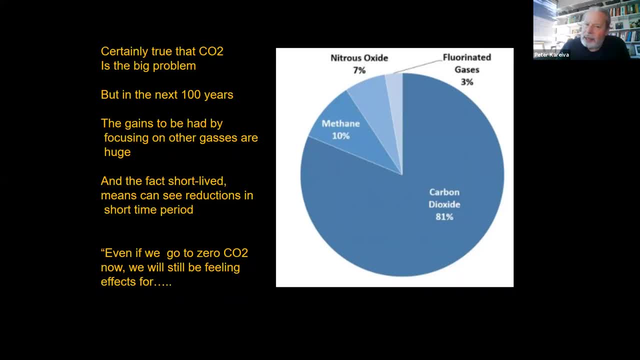 the gains to be had by modest reductions in methane and nitrous oxide are huge. By that time, you know shifting 1% of those is like 10% of carbon dioxide. Because you know shifting 1% of those is like 10% of carbon dioxide. 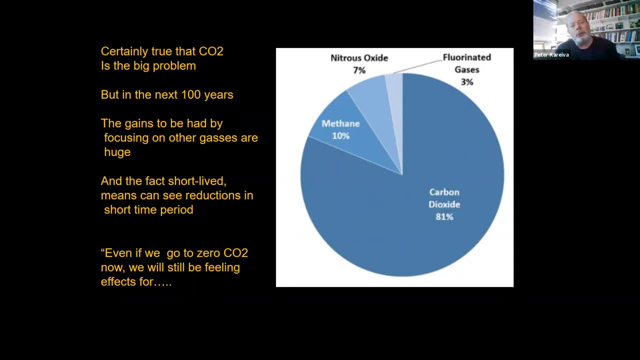 There's another advantage, in terms of the short term, of focusing on those greenhouse gases, and that's is you often hear the narrative about carbon dioxide up. Even if we went to zero carbon emissions right now, it's not going to do any good. we won't even see the results. 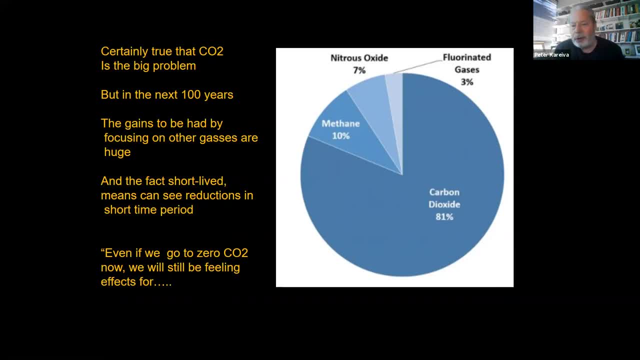 see the effect of that reduction for another 500 years. And that's meant to motivate boy, we really got to get going. But if you shut down nitrous oxide and methane, you could see the effect of those reductions much more rapidly, much, much more rapidly, because they don't stay up. 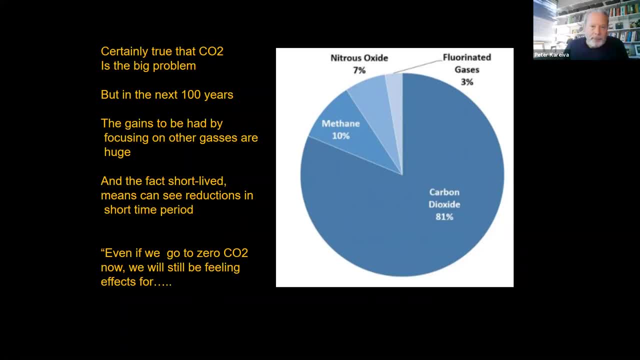 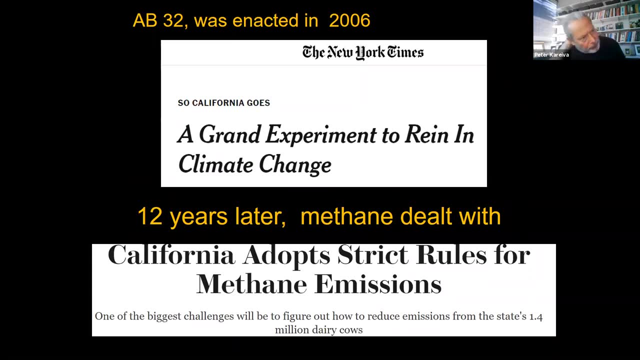 So you shift the balance. So, as an interesting example, you know California, which prides itself on being environmentally progressive and being ahead of everybody. They passed AB 32.. In 2006,, this one in Schwarzenegger, And you know it got headlines. 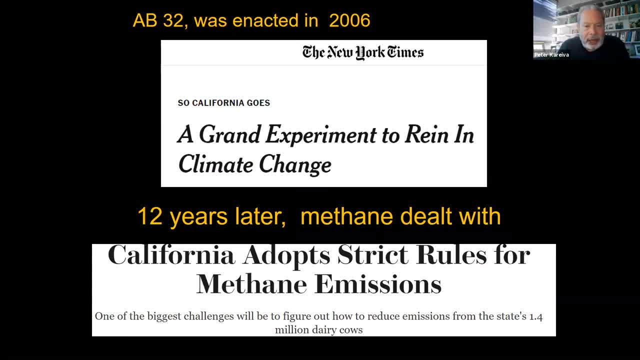 all over the world about a grand experiment to rein in climate change, And this was all about CO2.. It was cap and trade, it was a number of. the whole policy was CO2 in 2006.. Only 12 years later did California deal with methane. 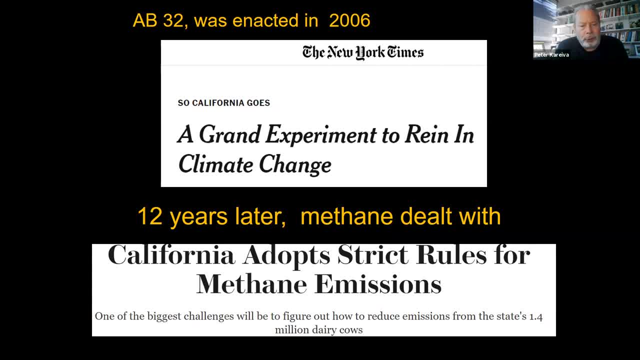 Only 12 years later and it still hasn't caught up. you know, the rules are still. they're basically dairy farms, They're really focusing on dairy farms, And to me this was a case that if you were really thinking about climate change, 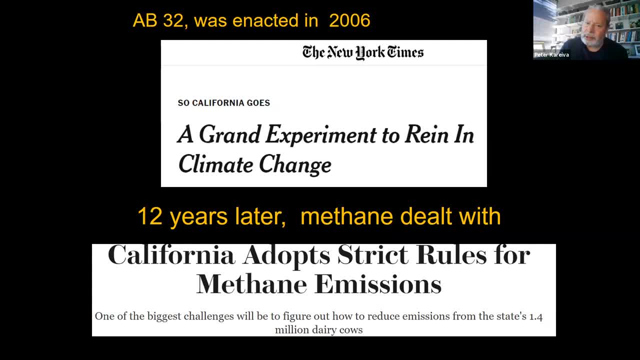 and where you're especially in this case, California- is it's- I think it's- the largest dairy producer in the country. It's not the largest, the second largest- Wisconsin might be more, but but it's huge dairy industry. The opportunity for making a difference with methane. 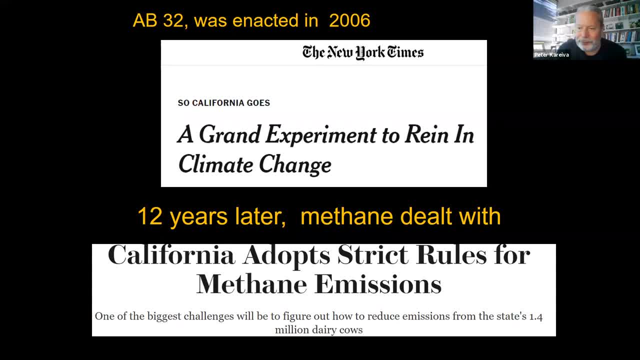 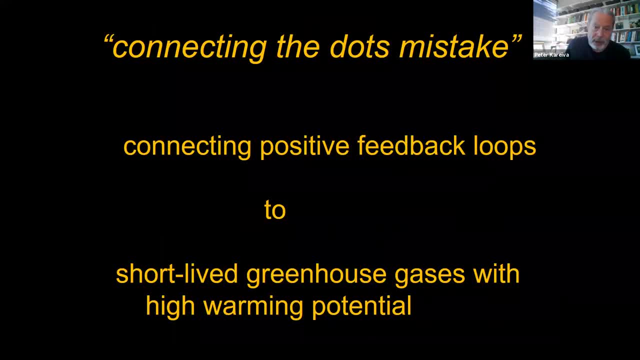 what that was there in 2006,. that was there. All the all the science was known there, but it was missed. So this is what I call connecting the dots mistake: Connecting positive feedback loops to short-lived greenhouse gases with high warming potential. 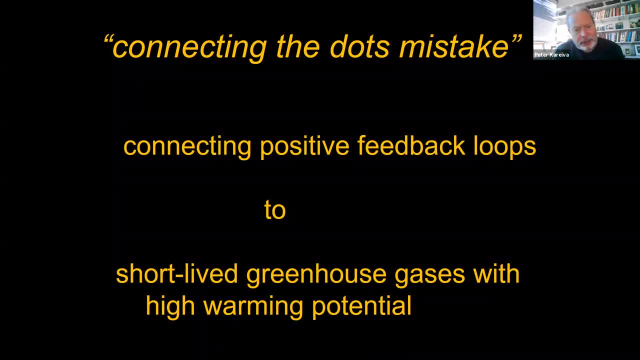 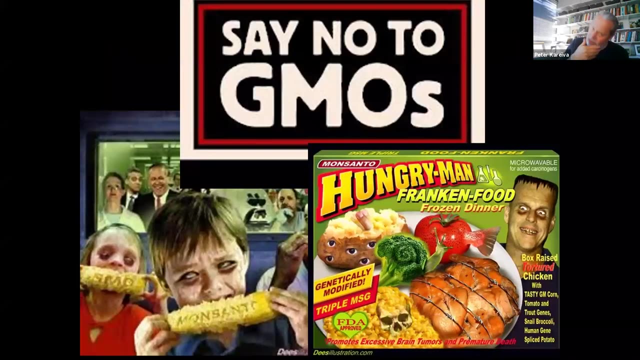 There's the, the positive feedback loops and the warming potential. There's no uncertainty about those two things. This is not about model uncertainty or or or obscure knowledge. It's just failing to connect. It's about the new technology. It's about the way we think about it. 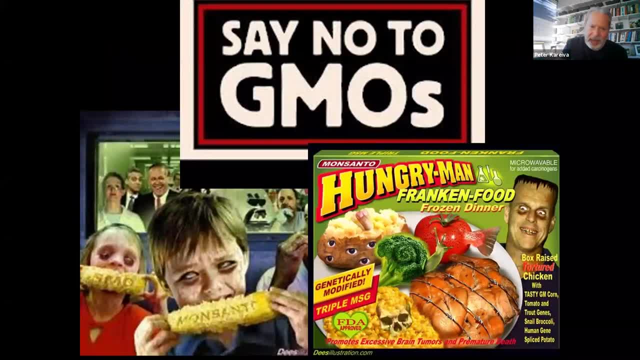 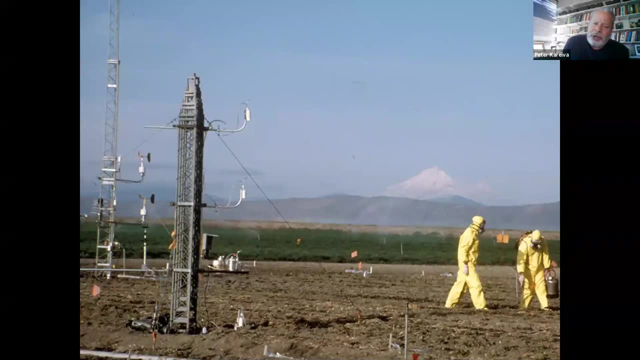 The next one I want to talk about is GMOs, And it's because I have personal involvement with it. This is when GMOs first came out. you know the ads against genetically modified organisms. they had to admire their imagination. I got involved in it because the first GMO was an ice minus bacteria. 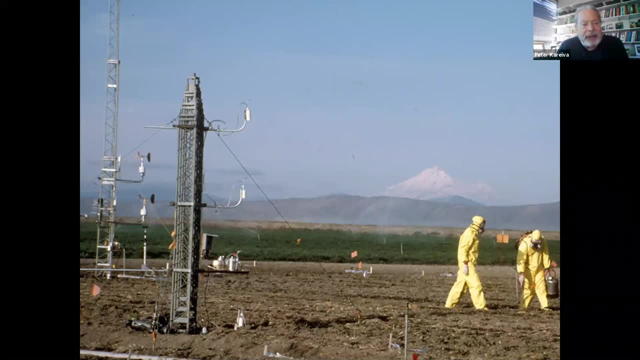 north of Berkeley that was released. It's a bacteria. that actually it's. it's just got a deletion, No addition. It's got a deletion and it doesn't cause frost damage And it was released as an experiment to see if it will be a way to to prevent frost damage in crops. 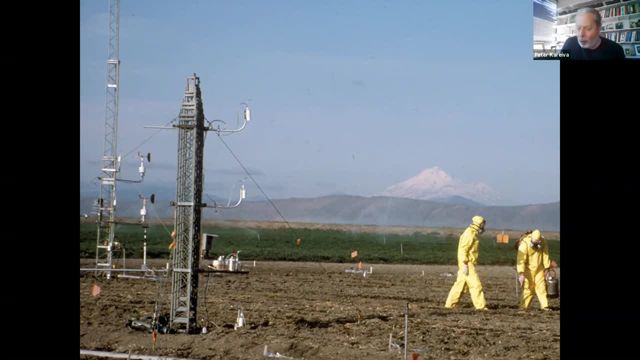 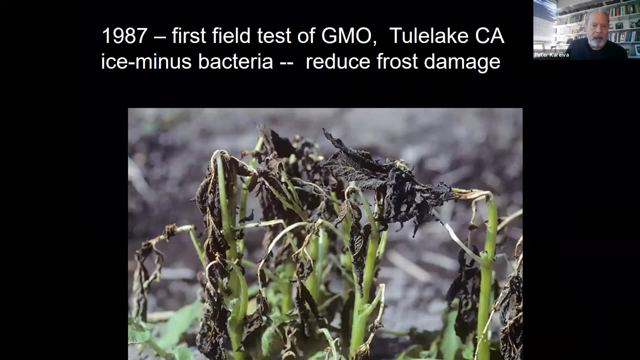 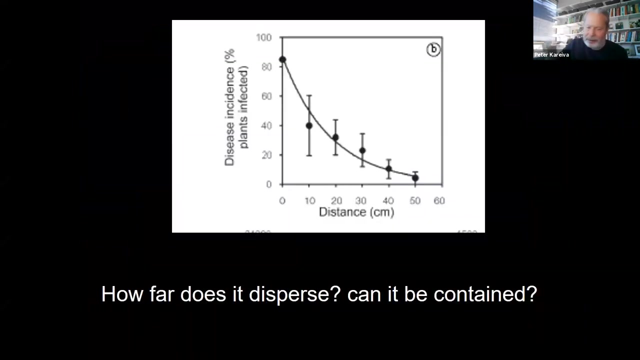 And you could see how in the experiment, how everybody had to walk around in these hazard suits heavily instrumented. this is 1987. And they were looking at I got involved because they wanted to know how far the bacteria spread. But what is interesting is as a follow-up from that, 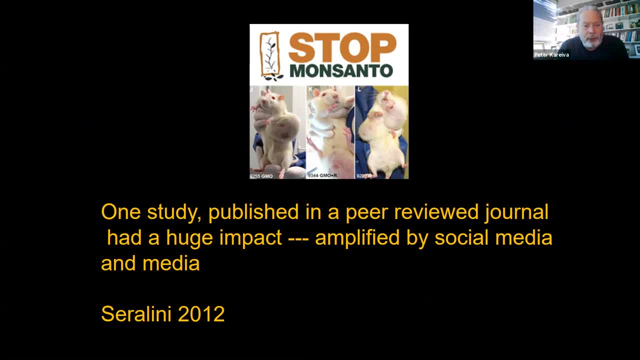 there was a study published in a peer reviewed paper in 2012 that had a huge impact on EU policy And it still has residual impact in trade policy with Africa and so forth. This was the activist sort of ad from it: Stop Monsanto. 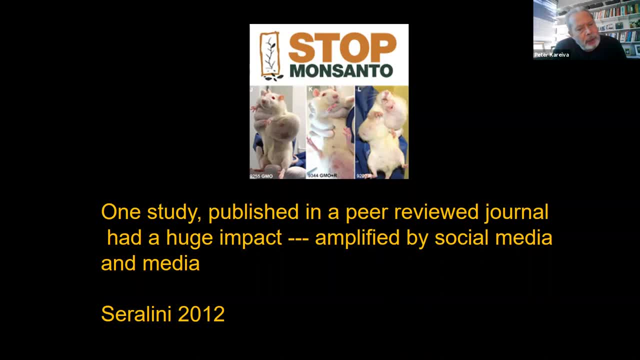 So it was a peer reviewed journal by Seralini And the what got the reason it was so significant it was it was one of the first studies to say: you know, everything else is short-term, All the other research is short-term. 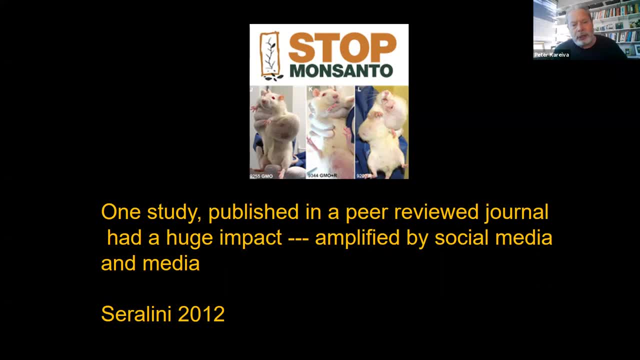 We're going to do a multi-generation study with- with rats We're going to. we have a long-term exposure- not you know, a week or two weeks or not, with insects. Long-term exposure in in in these lab mice. 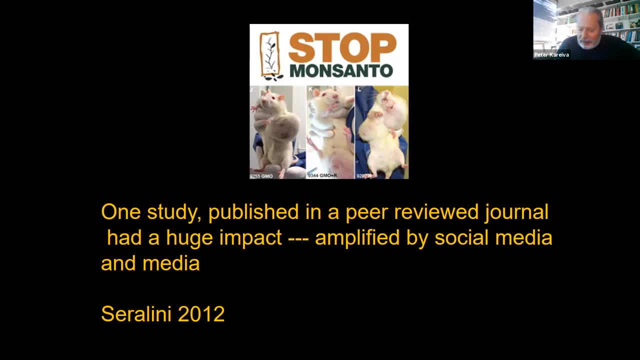 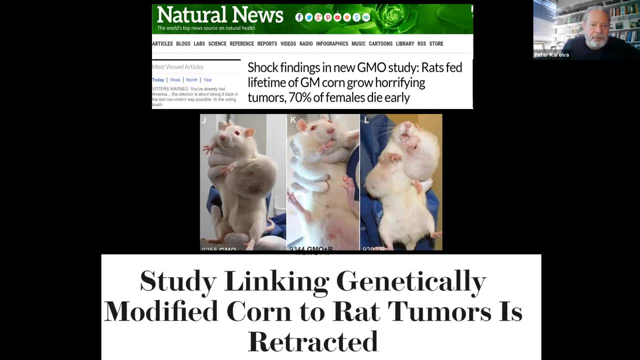 And we're going to look at tumors, And so this was the paper. This is actually the- you know the news release about the paper. Shocking findings in new GMO study: Rats fed lifetime of GM corn grow horrifying tumors. 70% of females die early. 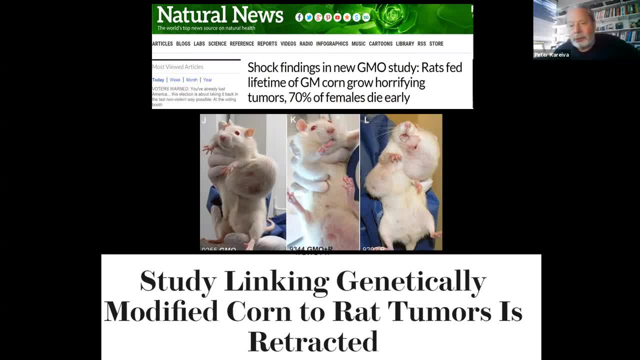 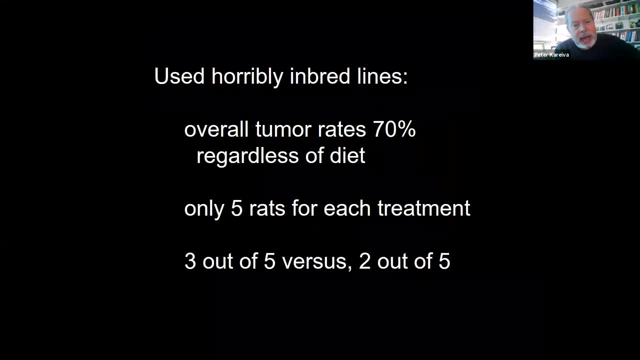 And these are the pictures published in it. That paper was since retracted. Scientists looked at it And it was retracted as really bad science. This was not. they used horribly inbred lines So that, regardless of the diet, 70% of the rats got tumors. 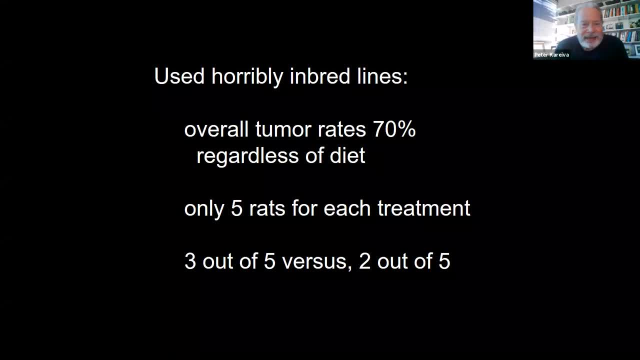 Regardless of the diet. they had such high inbred lines. 70% got tumors. They had five rats for each treatment And it was basically three out of five versus two out of five. I think you could see that. You could see why it got retracted. 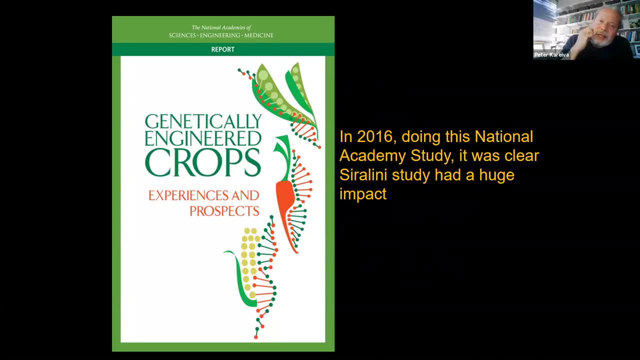 Well, I was on a committee in 2016 to review genetically engineered crops: experiences and prospects. And when you do these things, you, you talk to nonprofits and all the groups That study lives on. That study is cited over and over again. 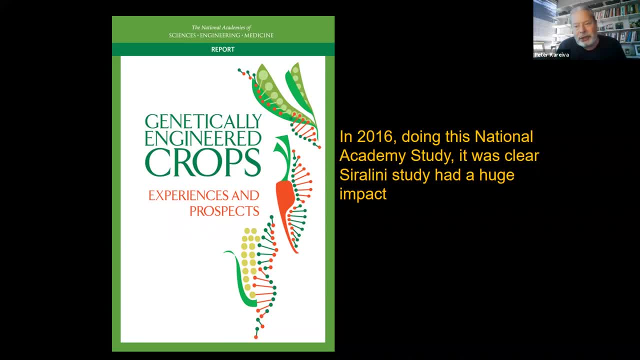 And the interpretation of its retraction was that industry pressured. you know the interpretation is sort of a conspiracy. So the study was good in the sense it it was longer term than anything else. That was a real contribution, you know, to recognize the need for that kind of study. 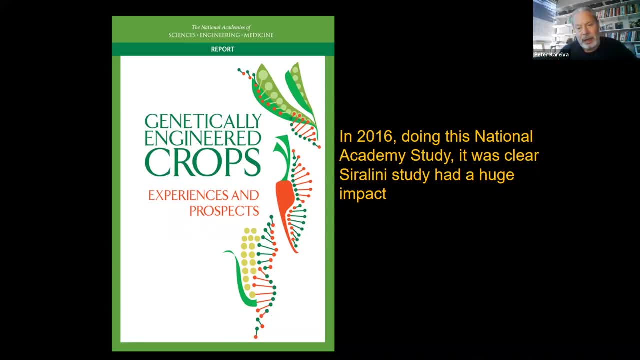 But it was so poorly done And this is still with us. You could go talk to people and they'll bring this up. Much the same with vaccines. you know the retracted studies with vaccines and autism. It's just. it's hard to undo this. 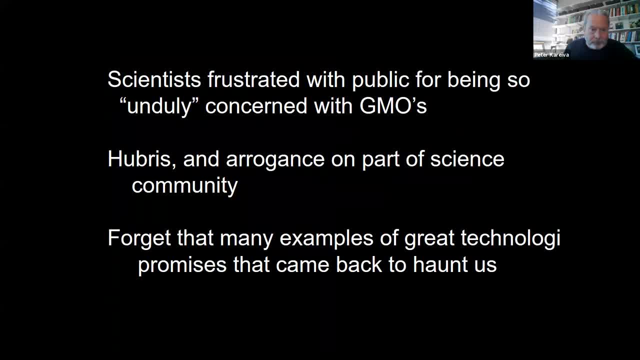 It's really hard to undo it. You know I have to put some of the blame on this on the industry and science for this, And that's because in the early going the scientists were really frustrated with the public for being so unduly concerned. 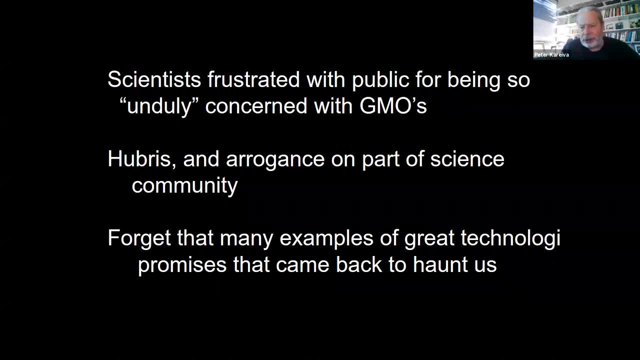 And you would hear them say things like: well, the public just doesn't understand, And that really, uh, uh, uh, uh, that was sort of it was just so arrogant and so foolish. And what the scientists didn't realize is the public. 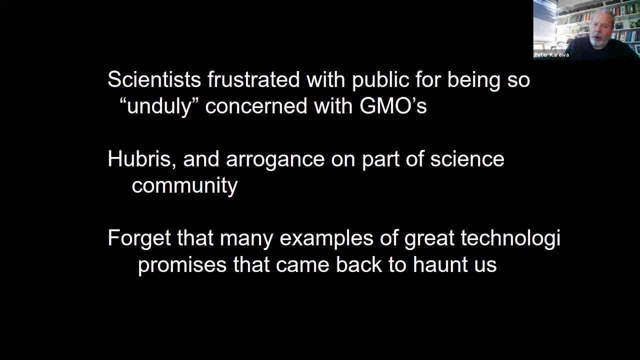 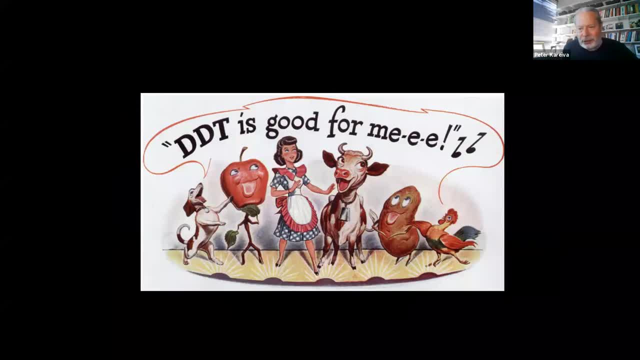 you know the public has a relationship with technology. that has a long memory And the memory included. you know thalidomide, babies and DDT. This is a from a Time Magazine article about DDT. It was an advertiser. 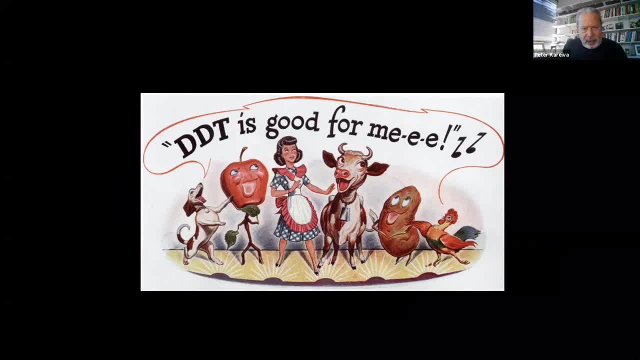 DDT is good for me, So the public has that memory. So don't criticize the public for having concerns about technology. Recognize those concerns and deal with them seriously. If the industry had done that, um studies like the tumor study might not have gotten so much traction. 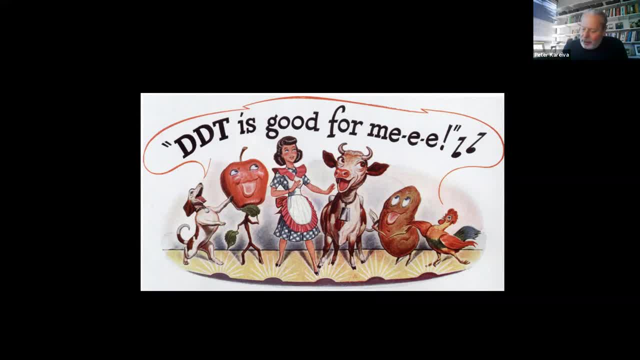 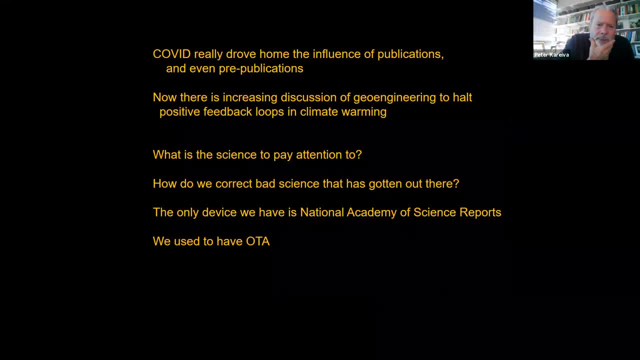 So some of the responsibility is on industry. but still it was a hard thing to crack. So I'm coming to a certain conclusion, I'm sort of wrapping it up for discussion. So I started thinking about this really because I think COVID really drove home the influence of publications and even pre-publications. 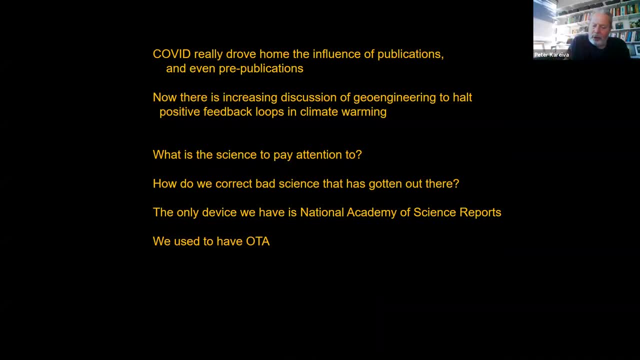 I mean a lot of us. I think we're reading, you know, during COVID we're reading everything we could scientifically, especially if we had an administrative position or we had decision making. You were reading everything, even in the pre-publication stage. 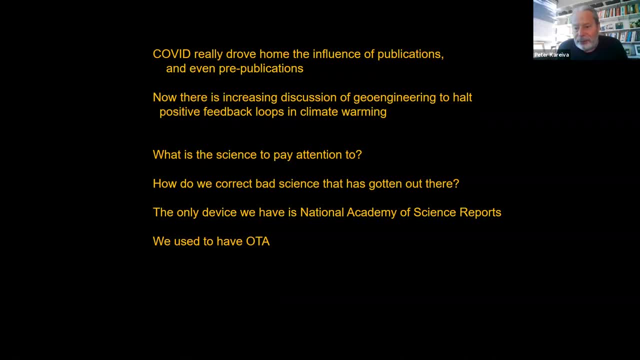 And there was like no referees. There was no referee, There was no sort of way of making sense of it, And that's unfortunate. And now you're going to see geoengineering, which used to be a science fiction kind of notion. Geoengineering is talked about seriously in policy because it does make the link to positive feedback loops. 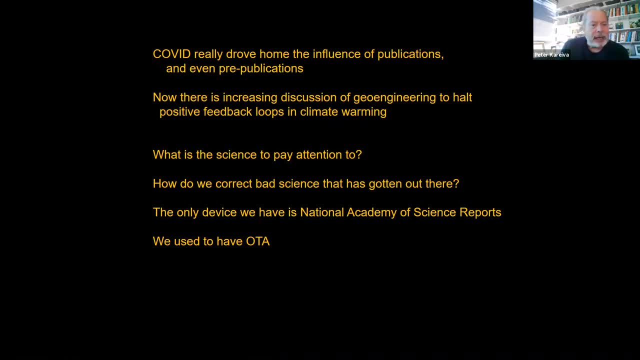 So the whole justification for geoengineering is that to shut down the positive feedback loop until we, our technology, catches up and we could deal with the CO2 problem. It's unfortunate that you know, 15 years ago we didn't focus on methane and nitrous oxides, by the same reason. 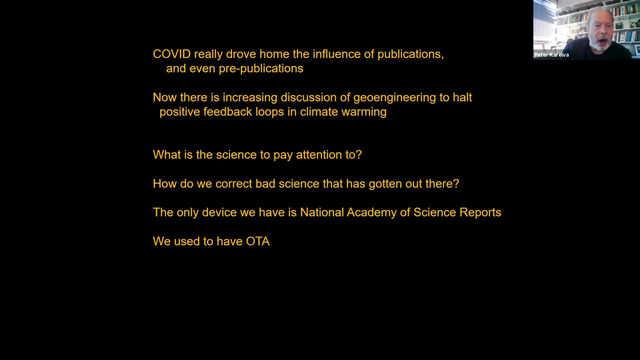 So the sort of challenge is: are: what is that? I want to? that I want to emphasize for environmental policy, where science knowledge is critical, is: what is the science to pay attention to? That's on the scientists, That's the missing. 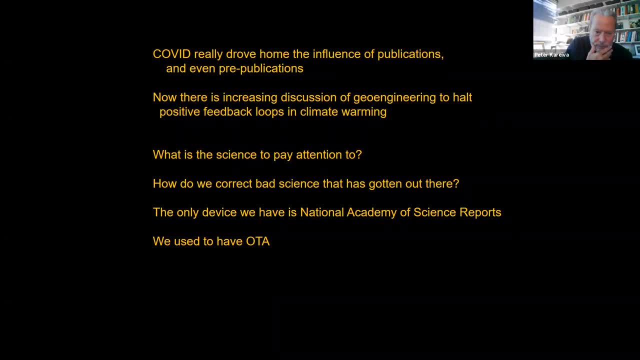 the connecting dots of positive feedback loops and global warming. The other one is: is how do we correct bad science that has gotten out there? It's been published in peer reviewed journals. The- I mean the methods we have are basically the National Academy of Science. 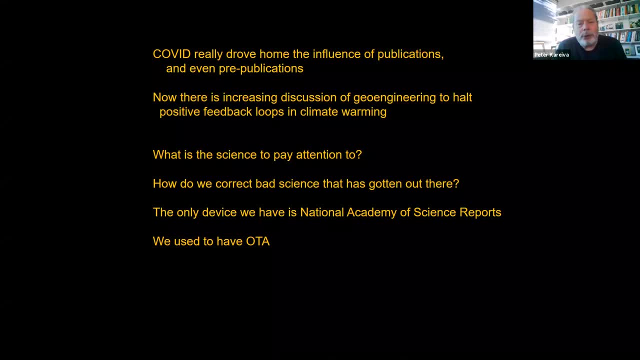 but that takes three or four years. You have to, you have to propose the study, you have to find the funding, you recruit the committee and then it issues the report. So the cycle by which our National Academy can deal with these big science policy. 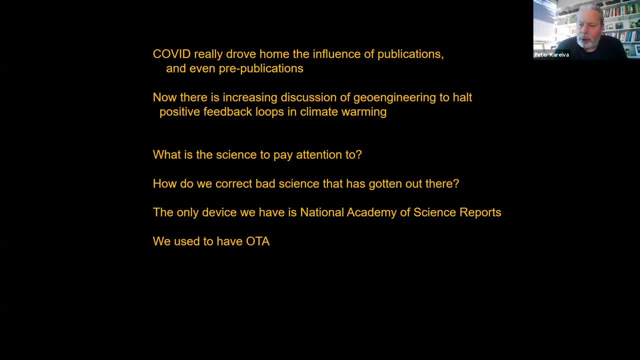 the nexus of science policy is just way too long. It's just way too slow for the modern world. We used to have OTA- I don't know if you that was- Office of Technology Assessment, which answered questions for Congress. That was much faster. 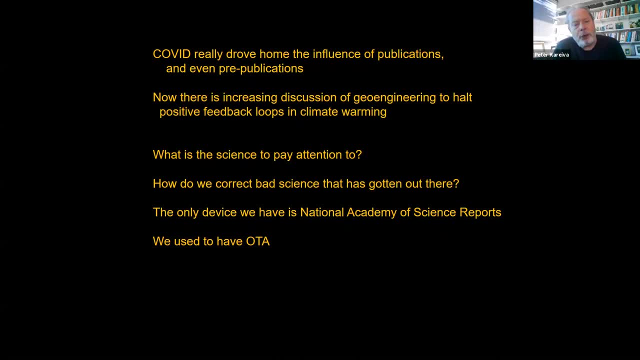 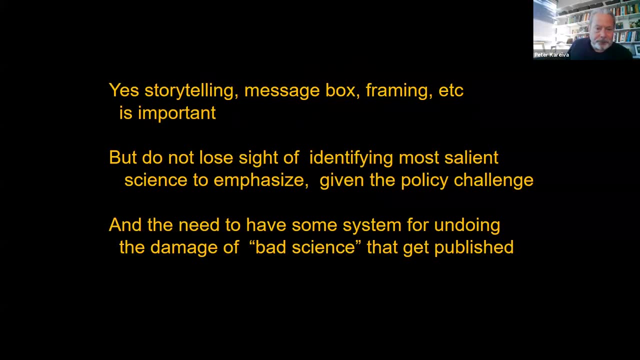 but we don't have it anymore. Now you could get an OTA report on a controversial topic out in a year, but we just don't have the system. So where I want to sort of end is saying that we've you know. 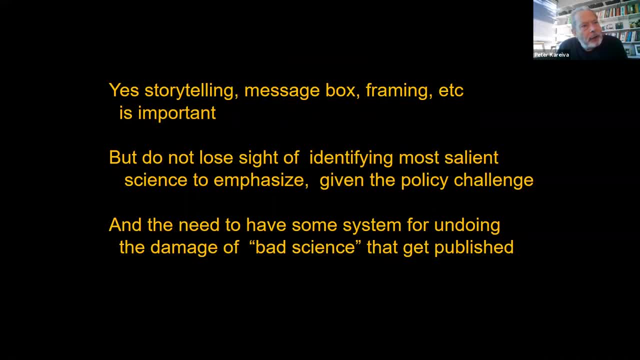 science. communication is at the forefront of all conservation. environmental scientists now I mean, they think about it, They take courses in it And storytelling and message box and framing is important. But I think the things that we're not teaching or we're not even having graduate seminars in. 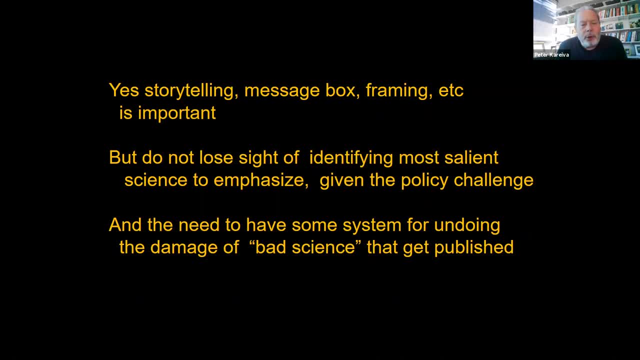 are the importance of identifying the most salient science to emphasize, given the policy challenge. so I think the climate science community missed out on an opportunity, And this is more like something that Eleanor Rostam, our promoter, talked about. What? 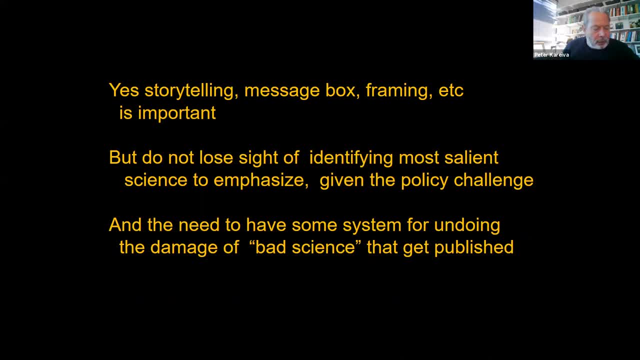 I mean, what are the? who decides what's credible? How do we control and, especially in this age of social media, how do we correct for the phenomena and the damage that bad science can do that gets published and then is amplified and can't be undone? 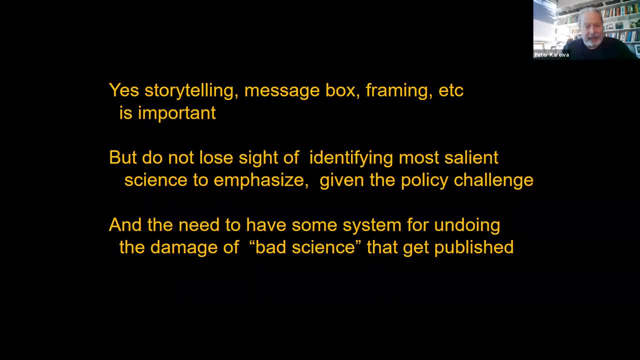 And you know, we see that with GMOs, we see it with vaccines and we'll see it over and over again. And I think it it we need to have some system, some rapid, we need to have some system in place to deal with it. 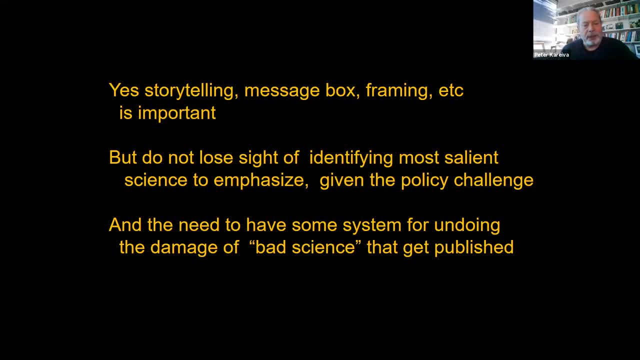 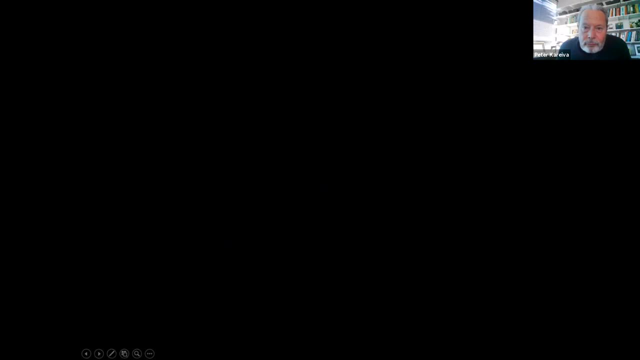 because so many policy substance depends on science substance, So where I end it there and take questions. Thank you, Peter. Why don't you go ahead and we'll save the applause for the very end? I'll try to keep track of chats. 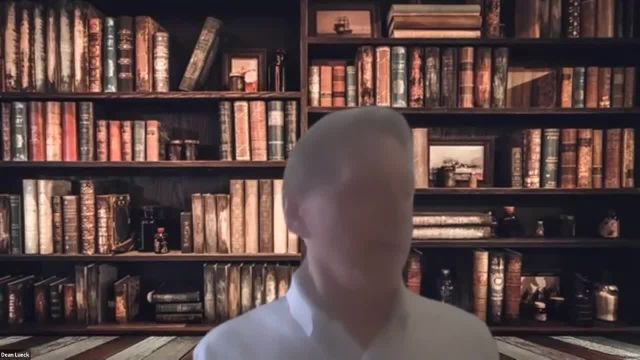 If there's a lull and you want to ask a question, go for it. I'm going to take my prerogative as moderator here to ask a question. So a lot, of, a lot of fascinating things to talk about and think about in terms of. 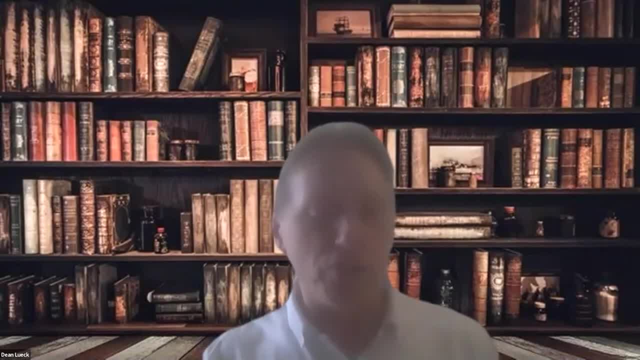 of policy, And one was science community communication. I want to ask you a couple things. One, where do the incentives to distort science fit in here? And if we're thinking about policy, we're thinking about political economy. Ultimately, we're thinking about interest groups, And you talk about conflicts among environmental groups. 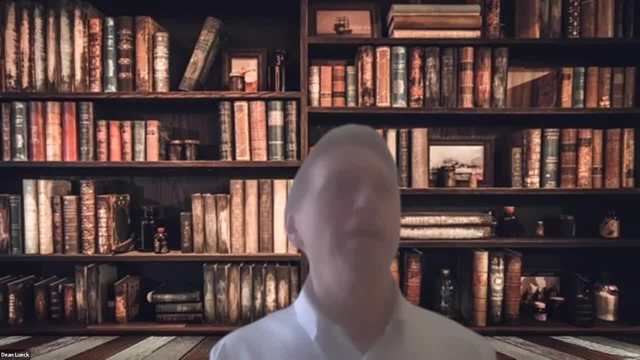 even you've got industry groups, you've got other groups. You know what kind of governance structure in terms of our political institutions- assuming you have sort of the right science and the right science communicator, you know what is going to generate some optimal. 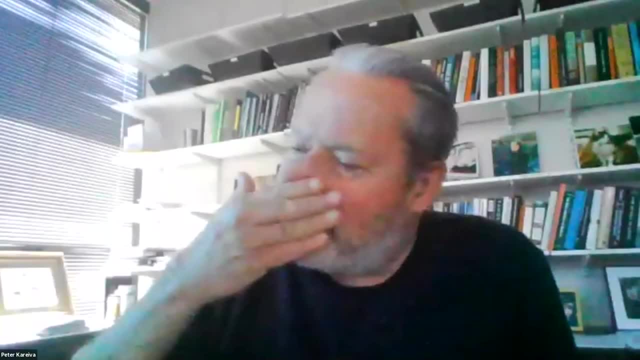 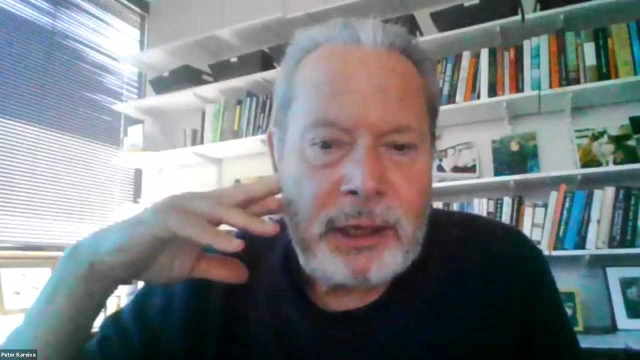 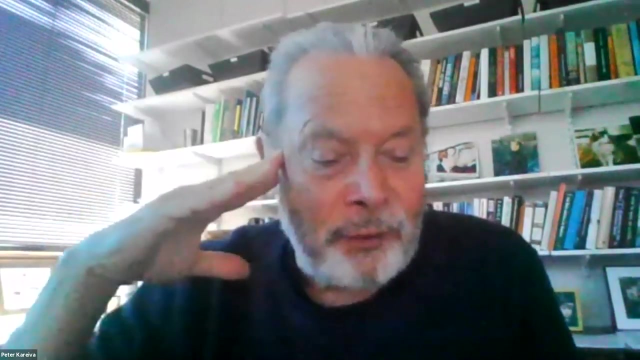 policy outcomes if you would. So you know there are incentives for sure for exaggerating science to certain sets, even by well-intended institutions. I was involved with salmon and the Snake River dams and I remember going out for beer and I won't give the name of the environmental 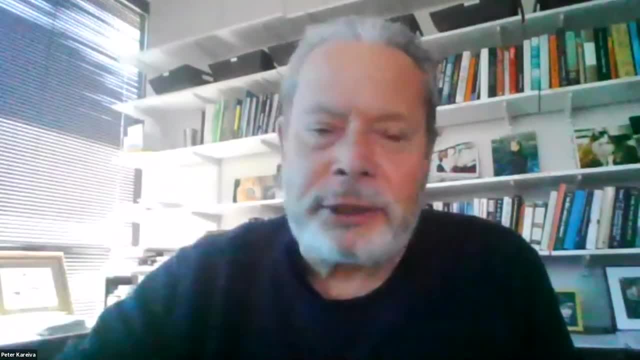 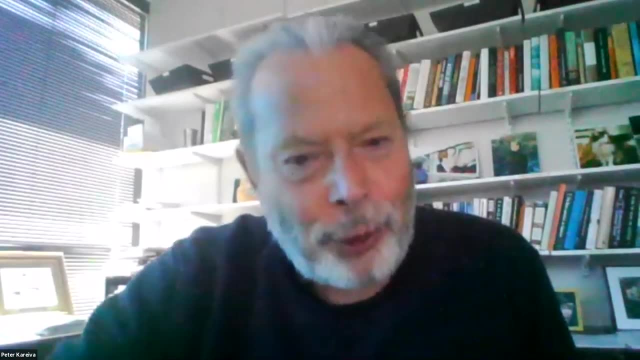 group. but they basically said: I said: how can you say this? The pit tanks tell you something otherwise. And the answer was it was our best fundraising. That's a little bit cynical, but So there, if you're an activist. 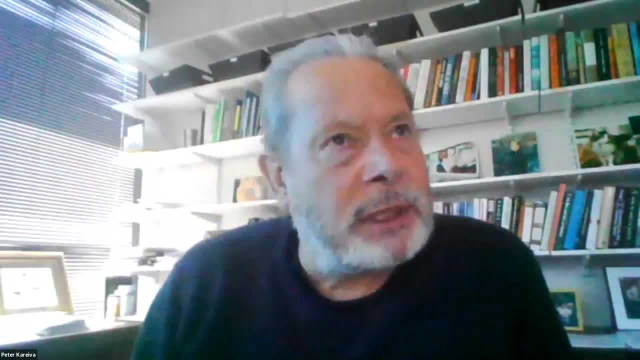 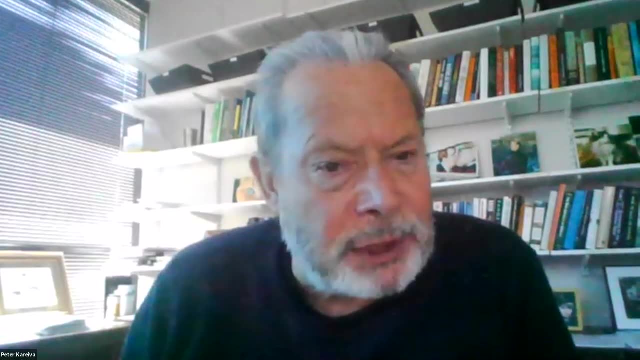 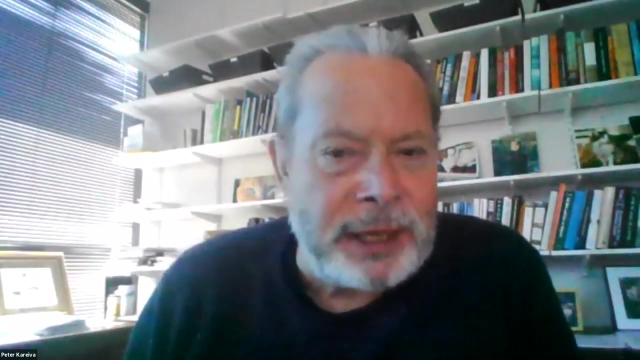 environmental NGO organization. there is some incentive for you know kind of biasing things and exaggerating things for fundraising purposes In the media. there's a movie that was in the top 10 of Netflix: Seaspiracy. Some of you may have seen it. 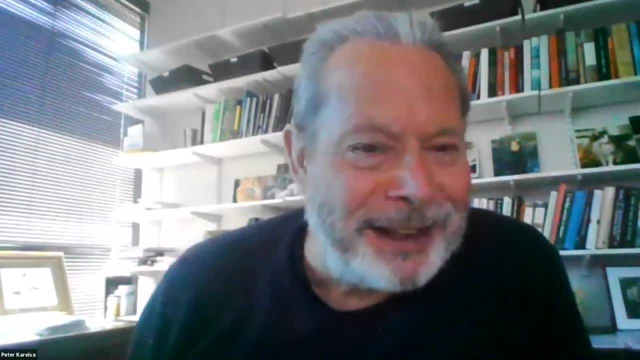 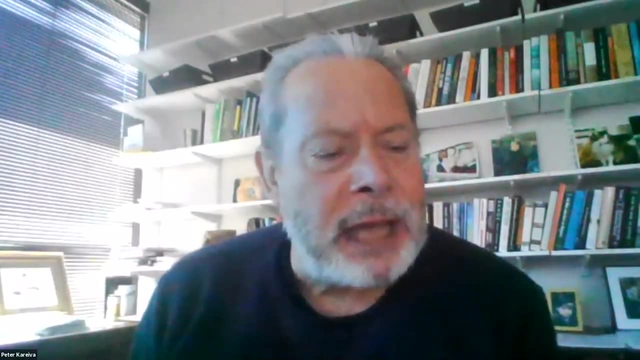 It's basically got everything wrong And but it did very well on Netflix. So there's those incentives, But I also think what is lacking is is that if you even for the honest person who wants to approach an environmental problem- and they happen to be very risk averse- 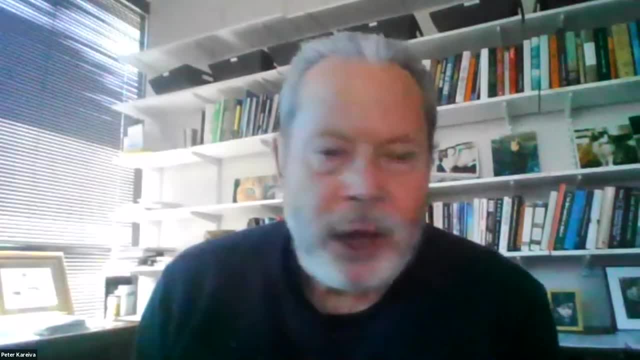 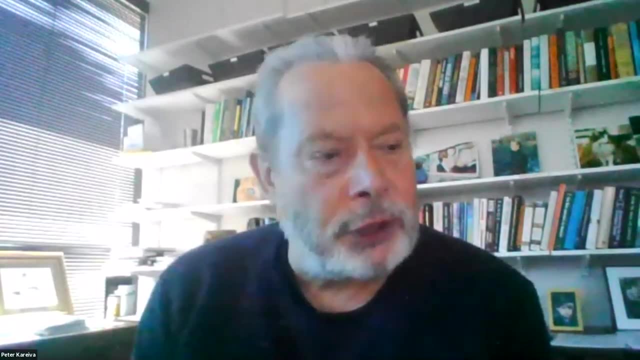 so some people are risk prone and some are risk averse. you're risk averse and you're asking questions about an environmental challenge and you're confronted with this literature, you're naturally, without distorting it, going to be drawn to the scary data. 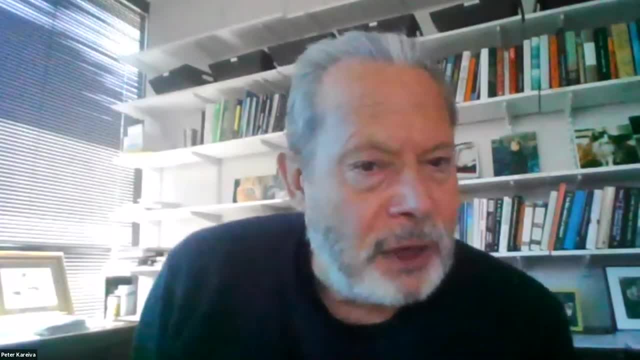 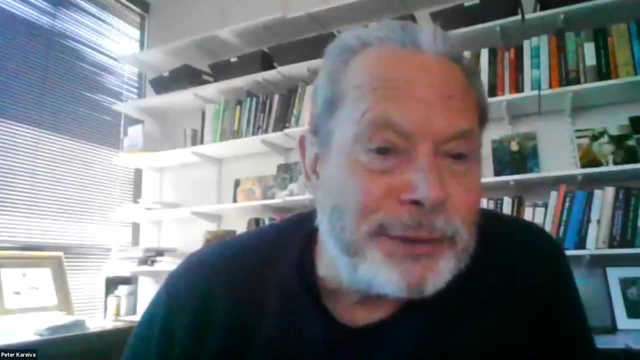 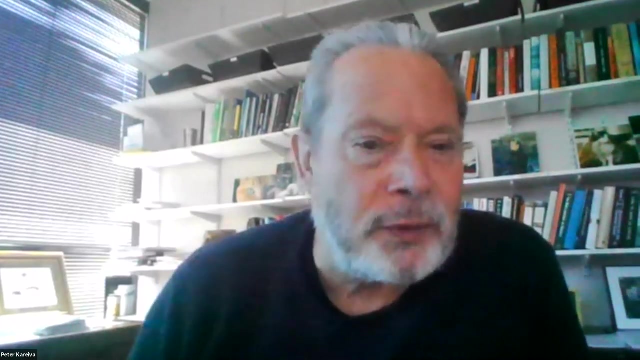 And and and. that's okay, But when we in the only structure we have right now really is the National Academy of Science, That that's what we use. We use the National Academy on all sorts of these controversies. 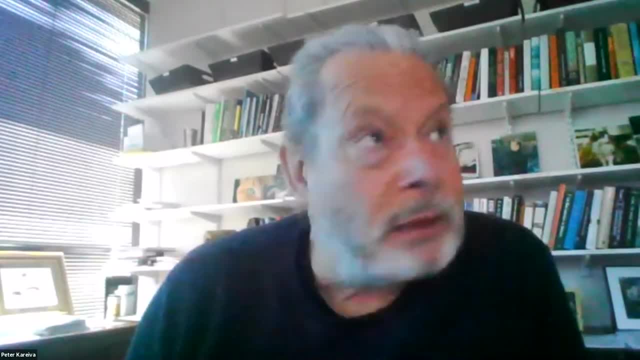 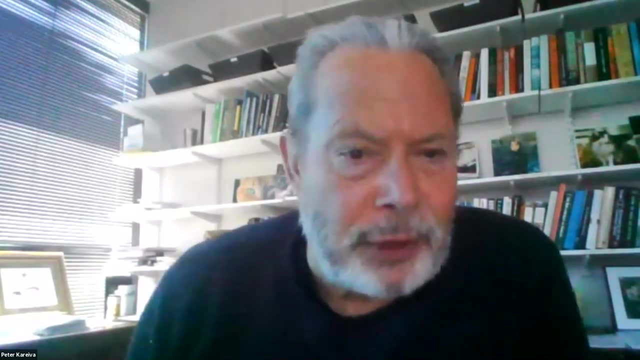 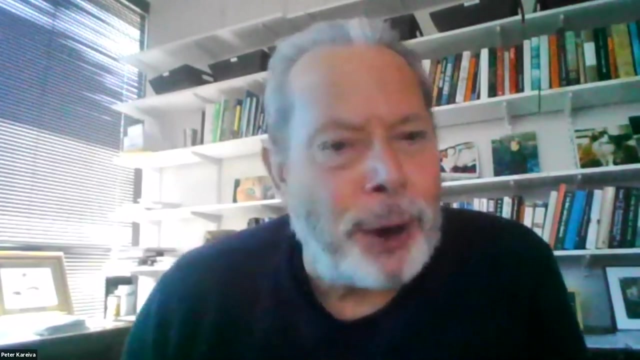 You know climate change: hunting wolves in Alaska, aquaculture off the coast of California, even local. We use the National Academy to do it. It's slow and it's ponderous. We need something that functions, like the National Academy. that's fast. That's my argument. 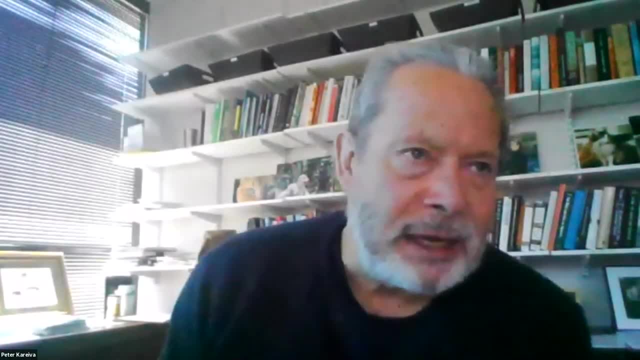 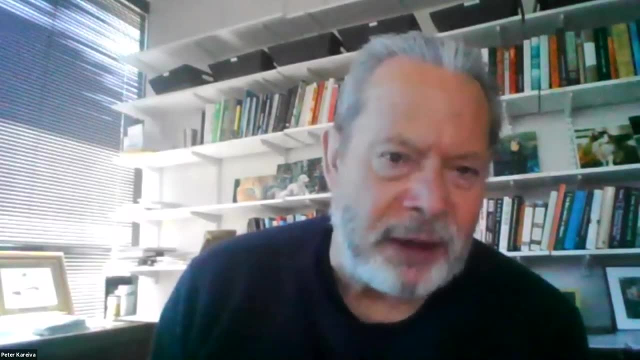 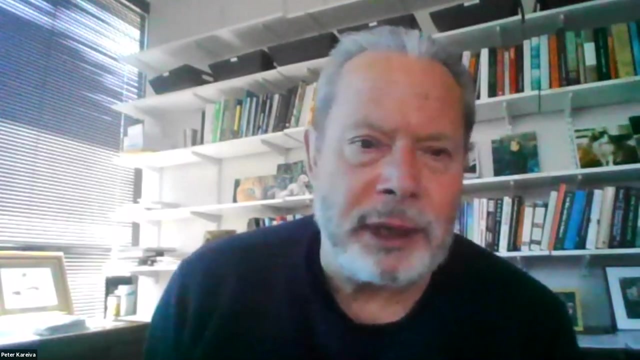 There just isn't anything To to do it, And I, to me it became clear because of COVID, But I think it also applies. I think it's going to apply to geoengineering, and geoengineering is going to be a discussion that's going to become more and more important. 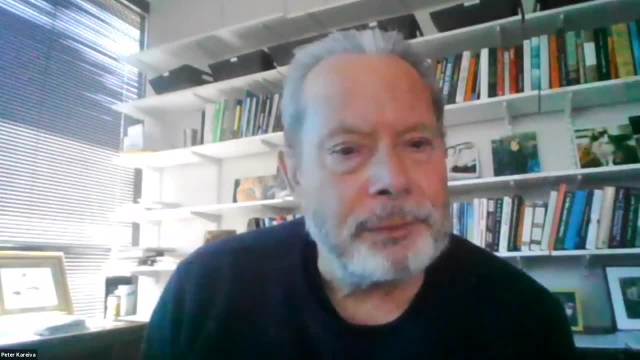 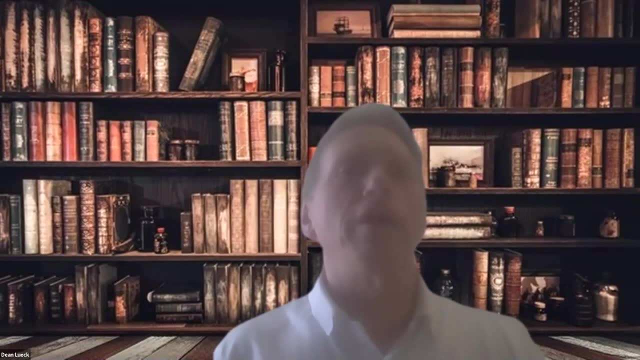 in the environmental arena. Okay, thanks. Yeah, that's, we may come back circle around to this. We have people coming in the chat. I'm just going to. I prefer you ask me a question. I'm going to ask you a question. I'm going to ask you a question. 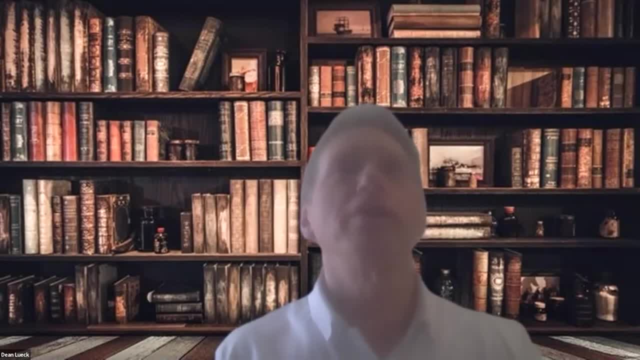 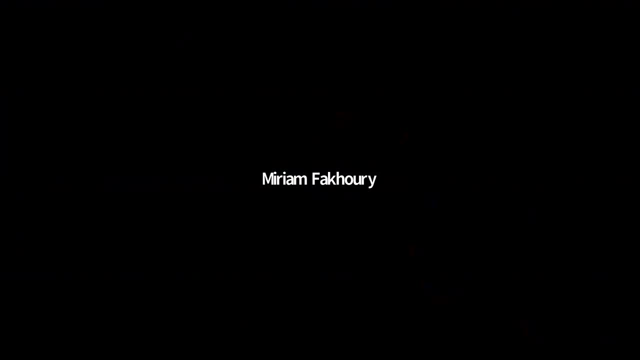 So, Miriam, please feel free to ask your question. Yeah, I'm just wondering what your perspective is on, like what the role of the scientist or researcher like themselves is when it comes to communicating to the public, especially a public that doesn't really understand, like, how science works or what, how to interpret data. Because I'm 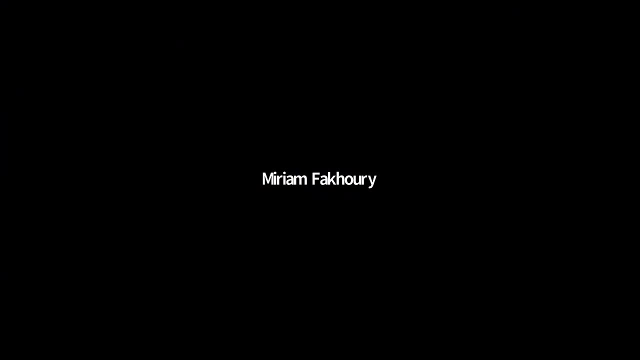 taking an environmental communication class right now. actually, and we've talked about this and that you know a lot of times the people who are gathering the data like don't have the time and energy and resources to communicate the data. you know they're trained in in whatever it is that they're studying. 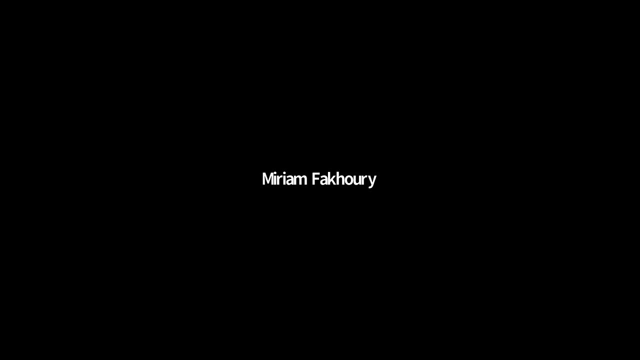 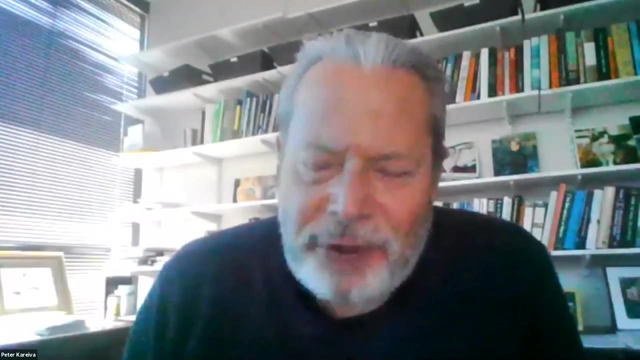 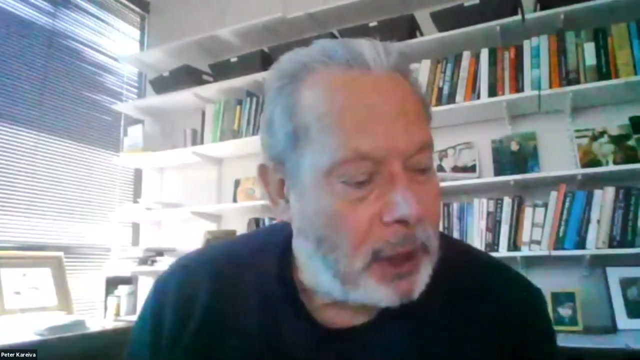 not necessarily teaching or communicating, But, as you said, that is kind of changing. So yeah, I just want to know, like, what your perspective is on that. You know that's a I bet you have some good debates about that, because I, because I've had it with grad students. So one perspective is: 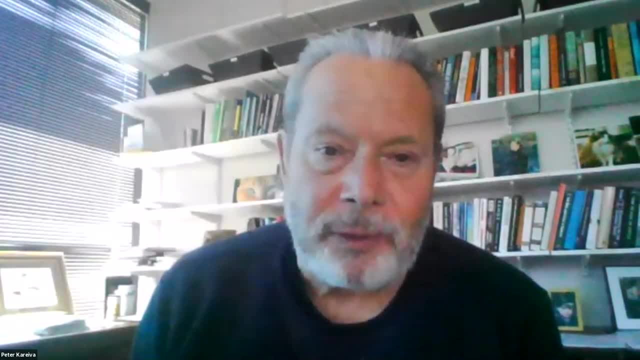 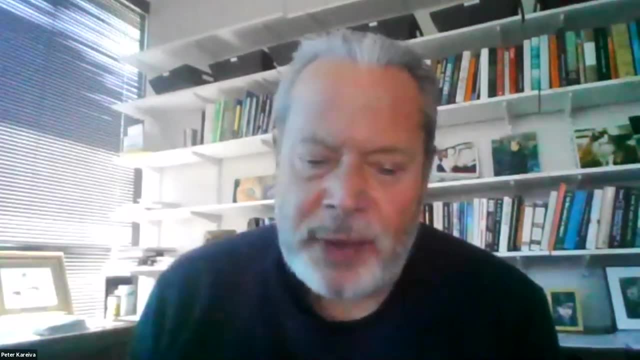 you'll see, actually, even as an editor handling papers, you will see sometimes reviewers of papers offer critical comments of a paper, saying, well, this is good, but it could be misinterpreted to mean blank, and I'm really worried about that. 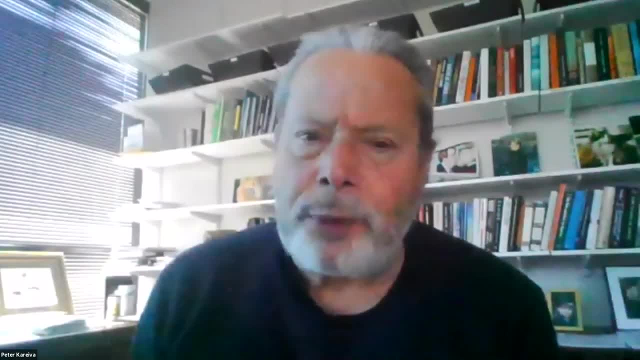 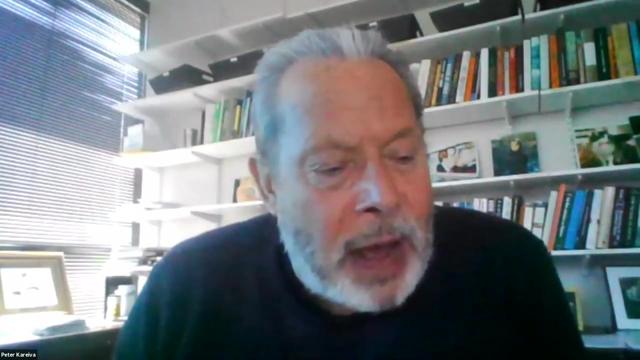 And then they, they, the reviewers, could get pretty heavy handed about it. So you could see, in the review process, even of peer reviewed papers, that pops up. You know, I want to respect the public's intelligence and I would just do my best to. 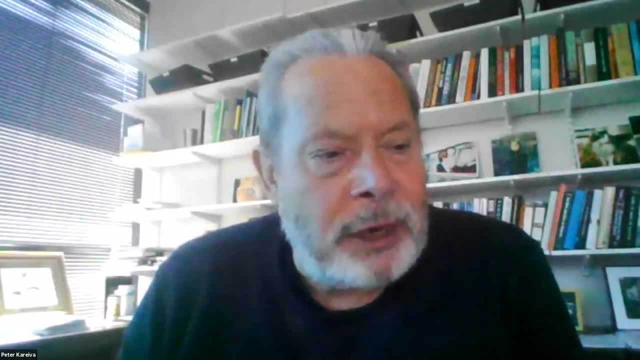 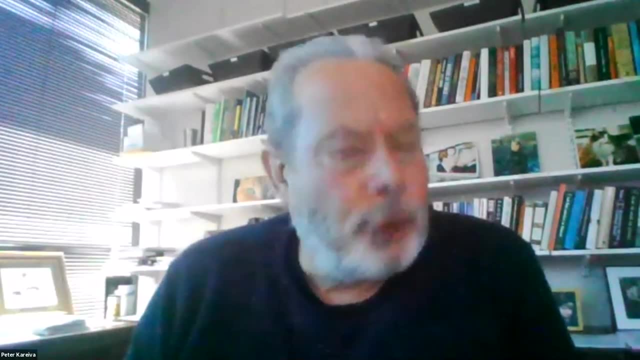 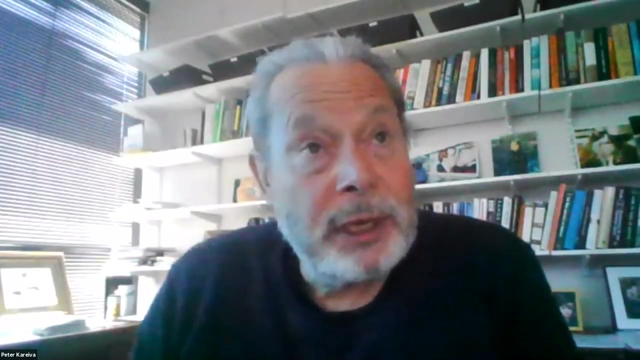 not try to you know, to not shy away from some data because you're afraid of how it might be interpreted, to instead do your best job of interpreting it straightforwardly. There is a tendency to shy away from saying certain things because of how they might be interpreted. 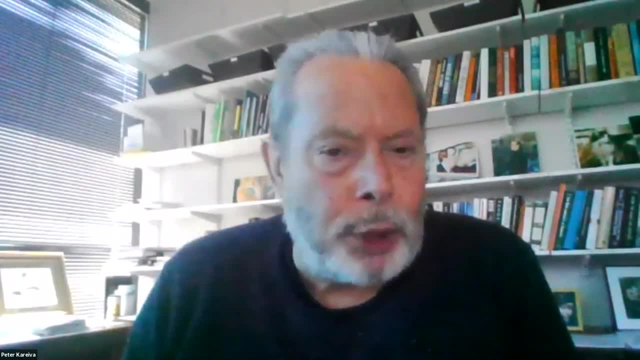 My first exposure to that was North American migratory bird declines and a very famous study that reanalyzed the data from North American migratory bird declines and found there was no evidence of declines. Statistically, some species are going up and some species are going down, But I think there's a tendency to shy away from saying certain things. 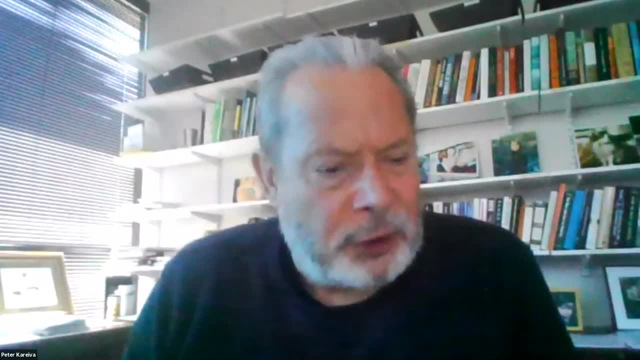 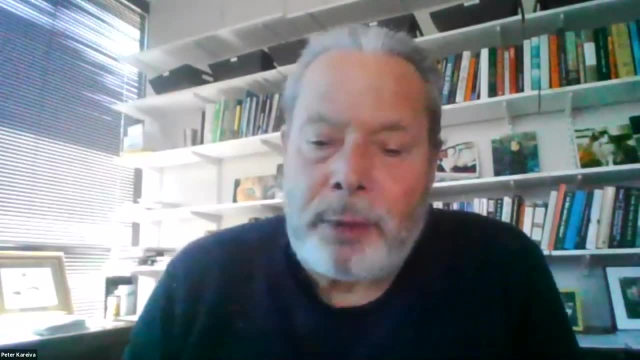 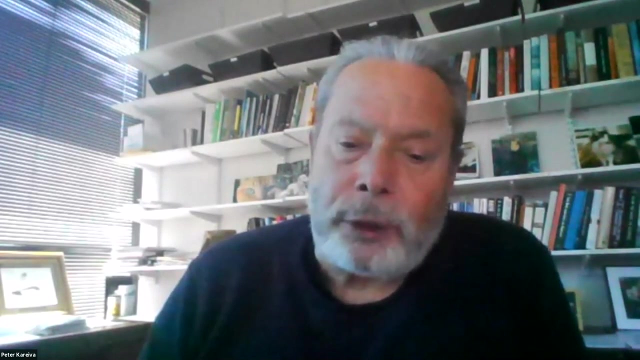 were going down and the species that were going down could be linked to some particular causes. The reviews of that. there was a big concern about that paper being published because North American migratory bird declines had been used to argue for. don't deforest the. 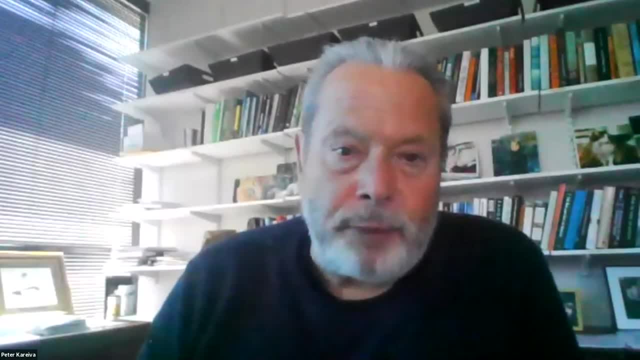 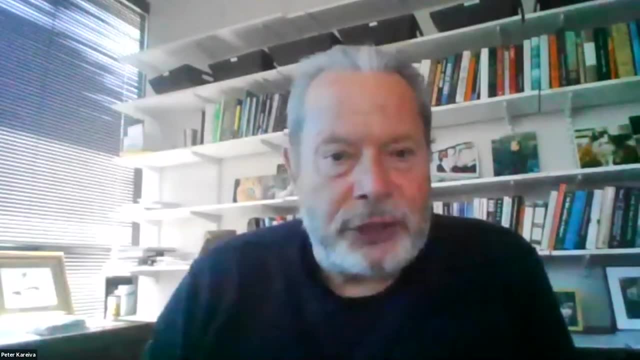 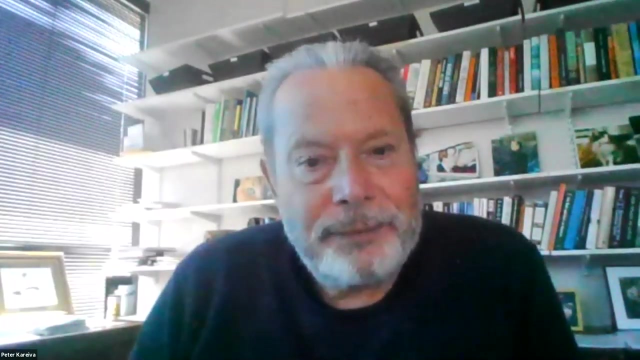 tropics And therefore be worried about publishing this paper because it could undermine this story, The story we've told about deforestation and warblers. I was an editor on that paper, So it was, But so I think you can't do that. 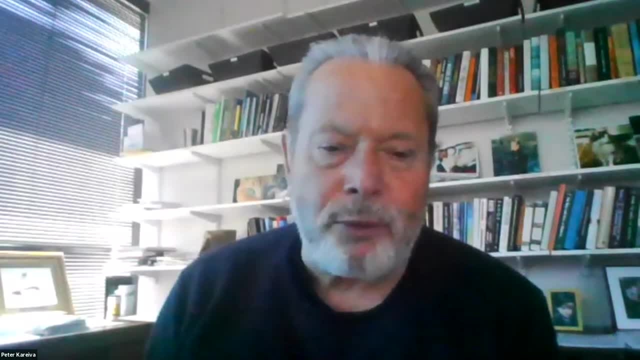 You can't worry about the as this, you can't worry about the implications, because you think the implications might not align with what you want to happen. You just have to be as clear as possible. You have to be as clear as possible. 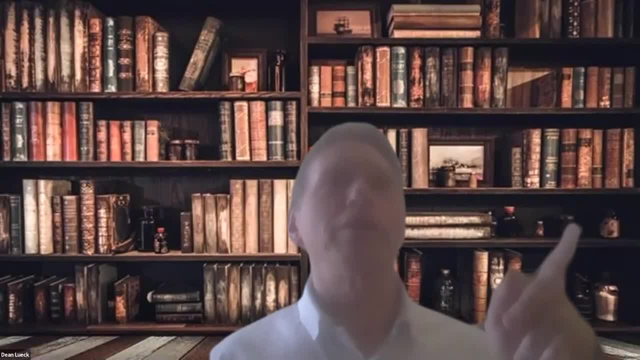 Okay, I'm asking people now to put their hands up, And I know we have at least one. And and why don't you do that? It's easy for me to see: I'm not a great zoo administrator, I'm learning. So, Jessica Steinberg, please. 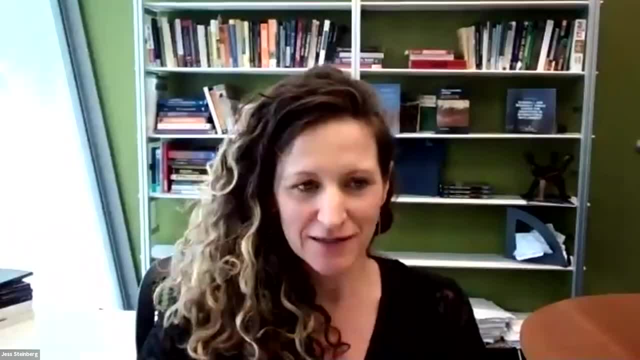 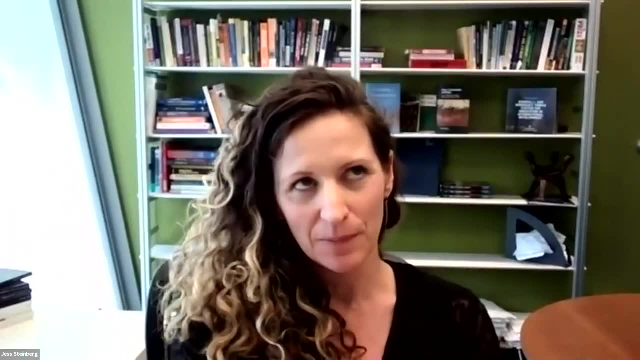 Thanks, Dean And thanks B. That was a really fascinating. I'm a political scientist way outside my wheelhouse and I learned a lot. I guess my question is for us about this sort of point before the last question, but also relates to it, which is: 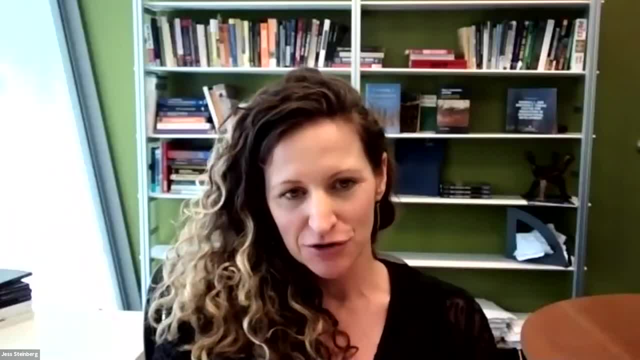 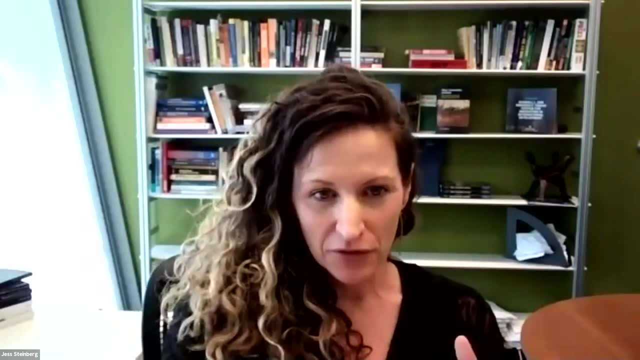 is: what is the benefit of thinking about an international body of the sort that you are talking about over improving the peer review process itself, right? So it seems like the problem, right, is that the studies get through. we find out later that they were problematic in. 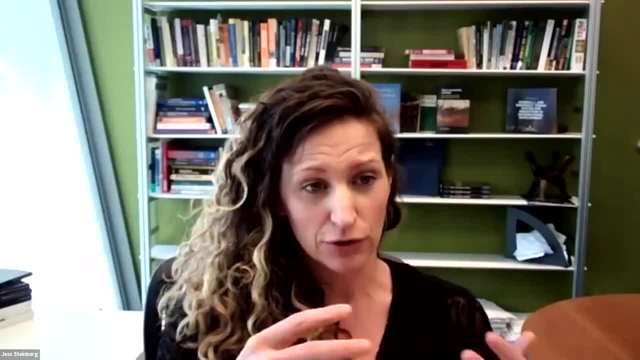 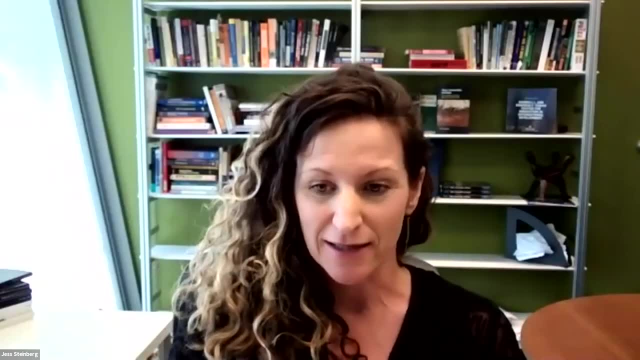 some really fundamental way and therefore should be not only retracted but publicly undermined in some way, such that they don't continue to carry the weight that some of them have right. So I guess one question is: it seems like it would be more efficient to improve the 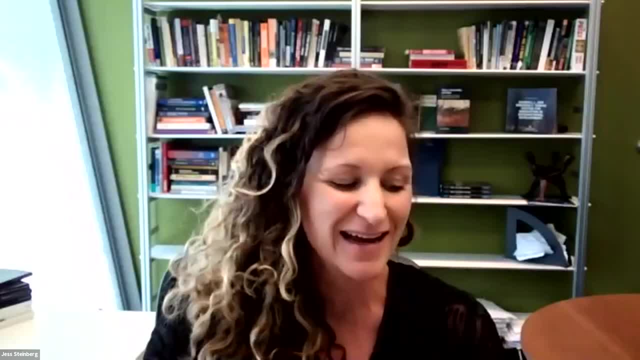 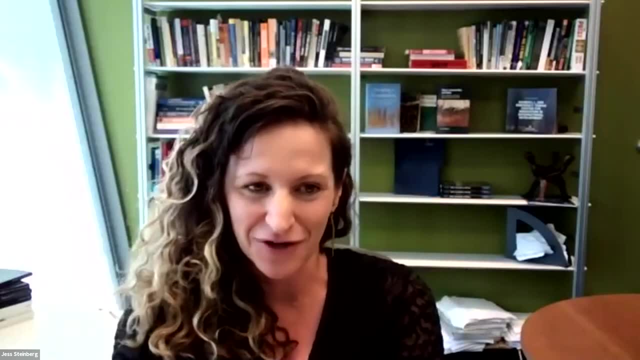 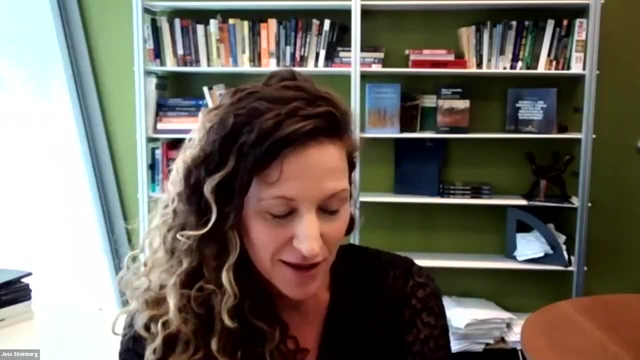 peer review process itself, and as many of us, I'm sure, could attest to it, is by no means perfect. It may be the best of a set of flawed institutions to evaluate at least the first kind of scientific research, but I'm curious as to whether you A have any thoughts on. 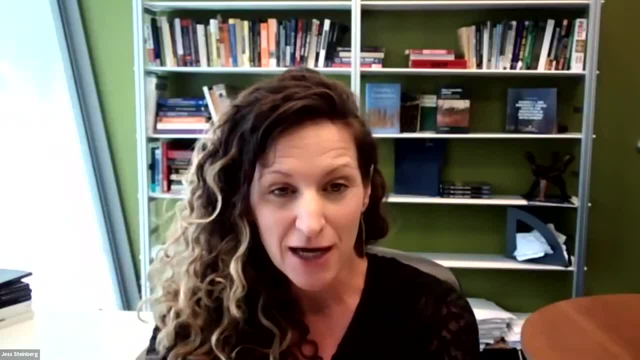 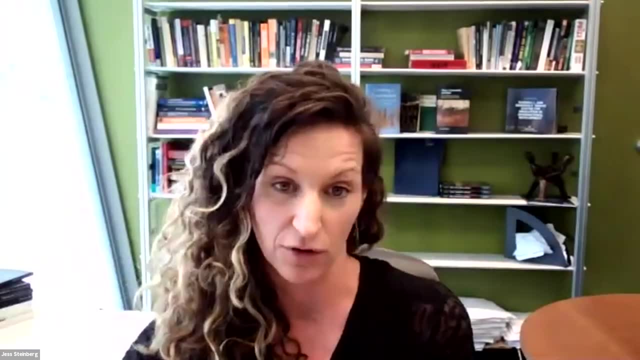 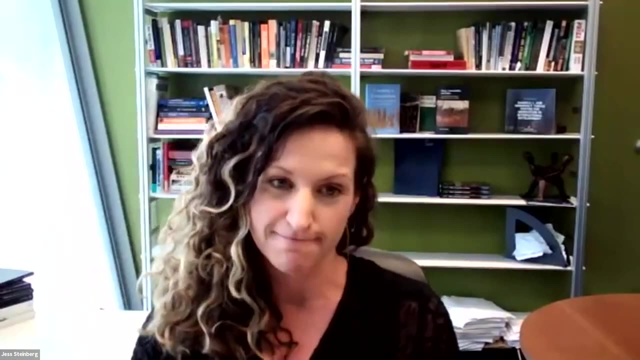 whether or how we might go about doing that as members of the scientific community. and, B, whether you think that this sort of second level of creating some sort of additional body that is faster, for instance, as you point out, than the National Academy to sort of keep tabs. 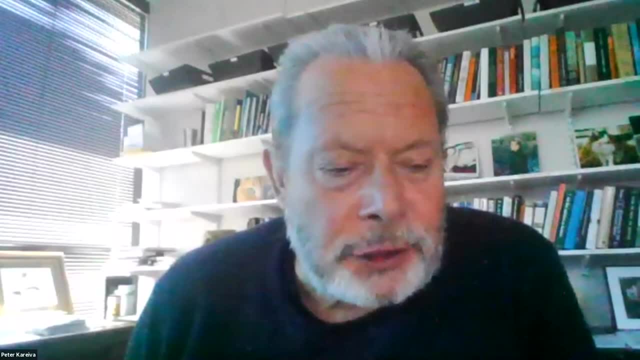 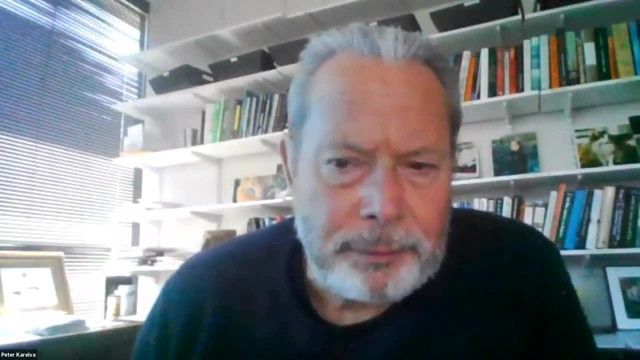 on this sort of thing. So you know, for the Cirellini study that was so obviously flawed, just a good peer review process would have caught it. I agree with that. But I think for more complicated issues like geoengineering is going to be. 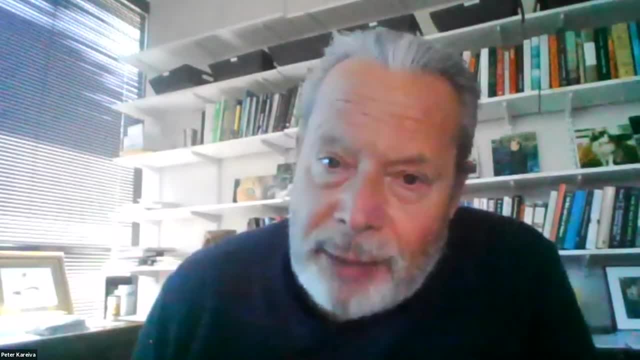 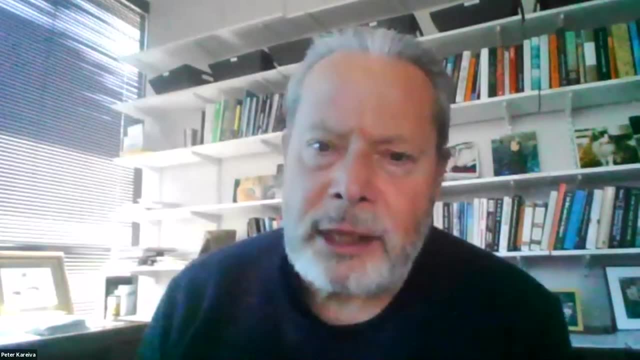 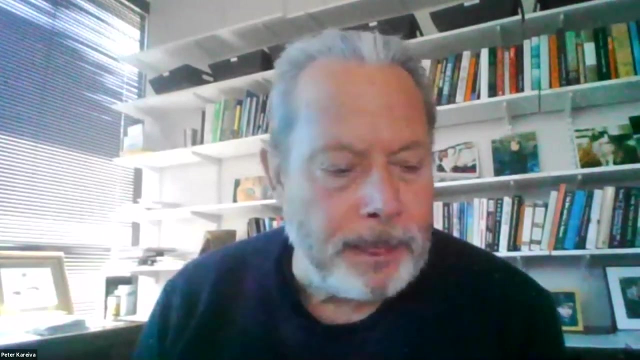 it's going to be very and like COVID for that matter. it's not so obvious. It's really hard to adjudicate, It's not clear what the right metrics are. I think the essentially, I think the public needs some assistance and help in sorting through competing interpretations and 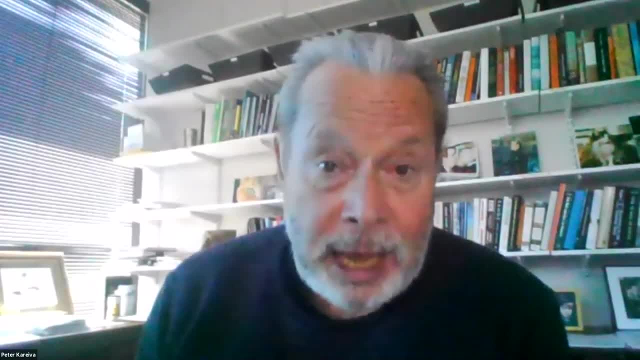 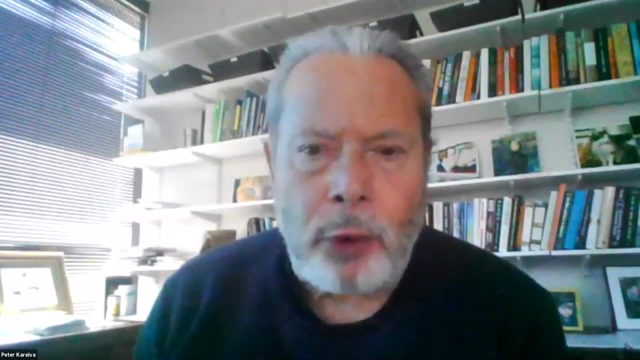 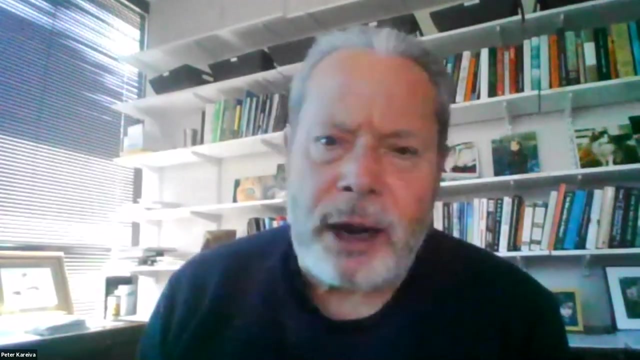 inferences, which is what the Academy does, And it gives you a fairly. you know it works pretty well, but it just works too slow, too slowly, And I don't think it would be that hard to generate. you know you essentially. 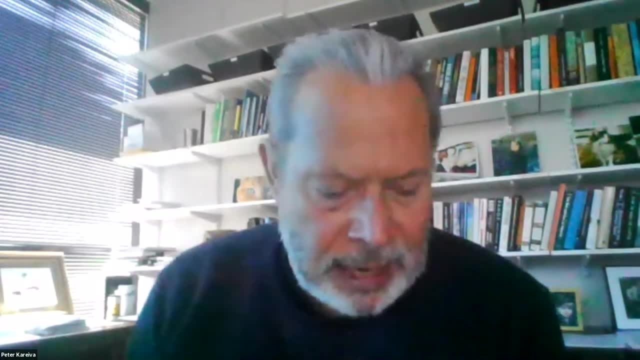 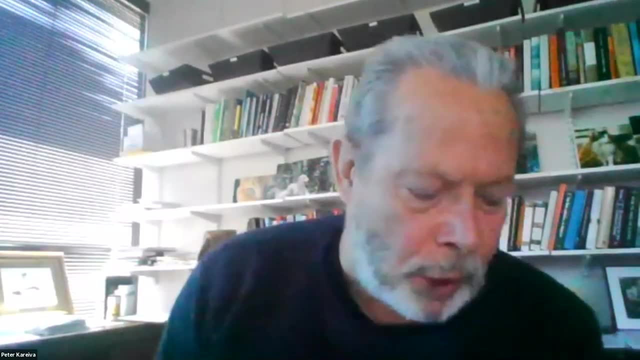 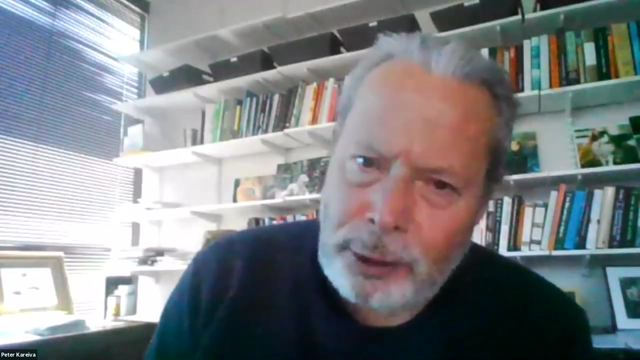 set up a nonprofit or something and you create incentives. You have a. the reason the National Academy works is because you have 20 different science scientists evaluating. It's not one. They come from different fields and have different perspectives. That's why it works. It's slow, but it works, because it's not one or two. 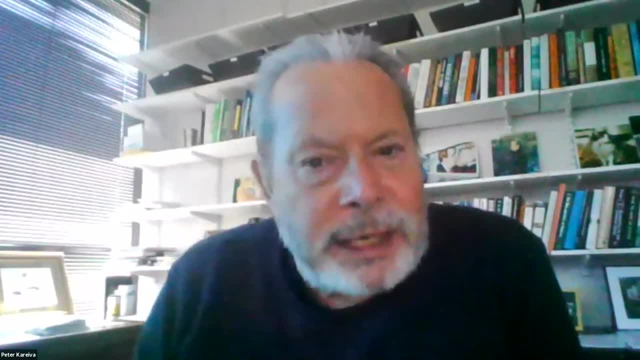 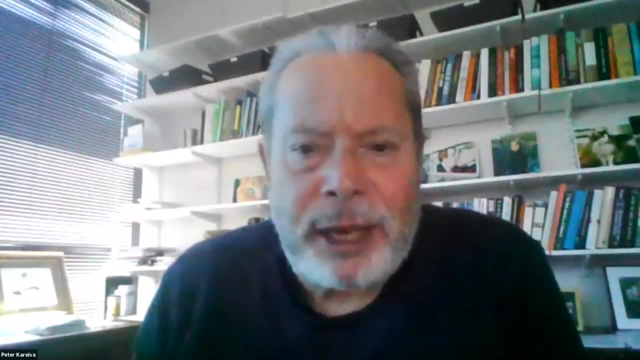 It's a collection. There's no reason you couldn't have 20 different scientists helping resolve an issue on a fast timescale. It would be more narrowly defined- I mean the Academy tends to be broadly defined- things like genericism, It's. 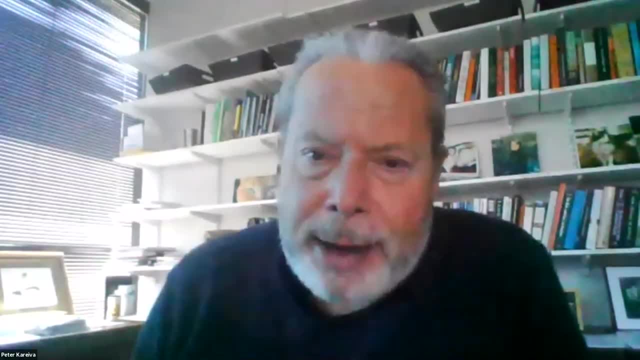 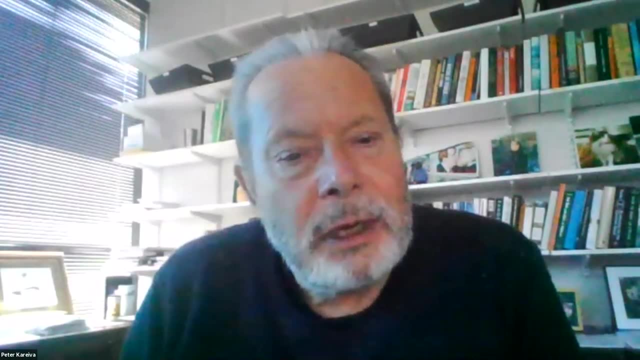 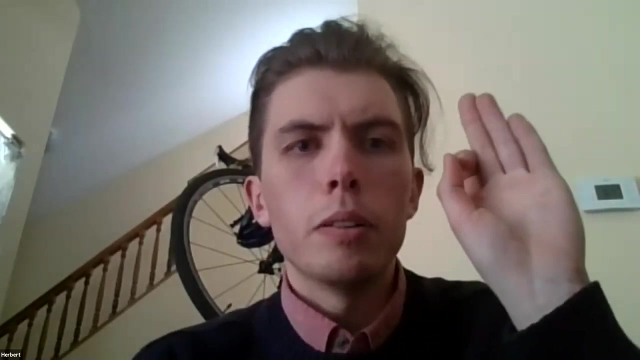 Genetically engineered crops, but on a short time scale, it could be Pollen in Mal and in Monarch decline, which was an issue, by the way, And that that's the type of thing that a system could address really quickly. What's the strength of evidence? How good is that? 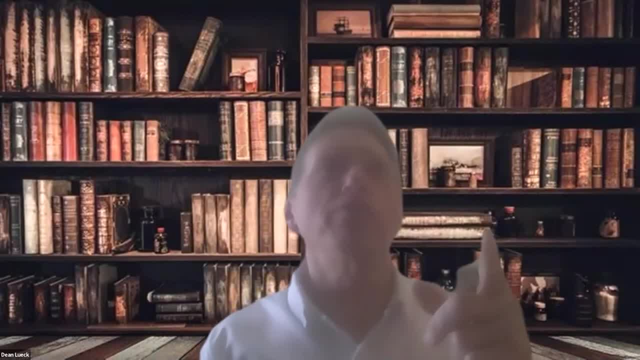 Yeah, Thank you, but we've got three. we've got three of the key. I'm gonna try to keep things moving. We have saying: first then Brian, then Herbert, Thank you. so, zhang, please are you there? his hands up? but yeah, i'm here. let's go to brian. i know he's there, i see him. 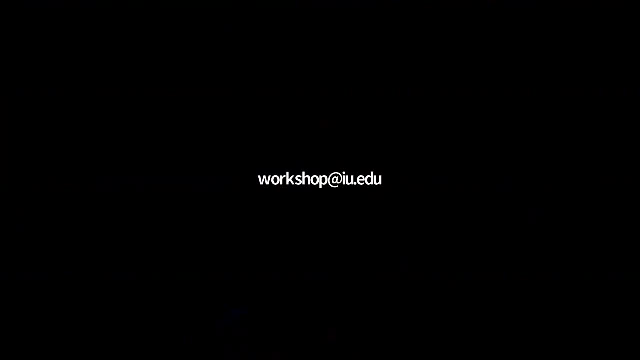 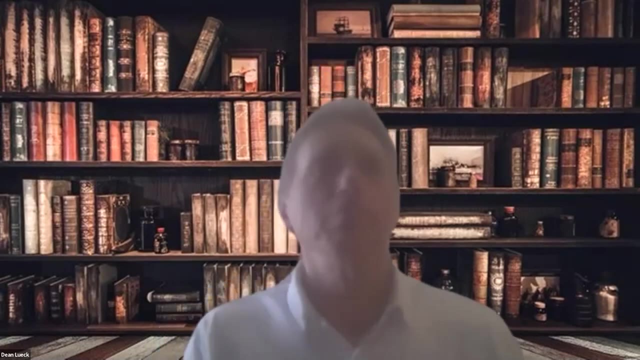 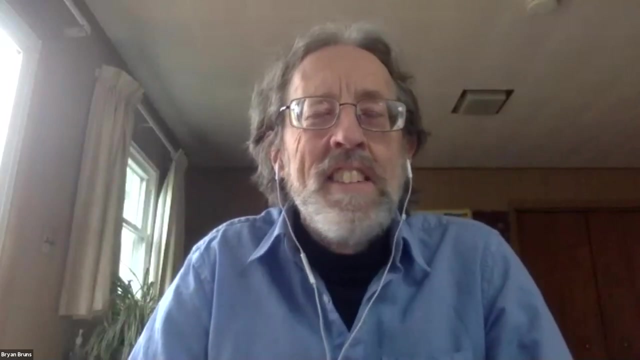 so go, brian, then zhang will come back to you. oh, he has a message in the chat. his microphone isn't working, okay. well, brian, go ahead, then i'll dig out the chat information. okay, um, in terms of a desire to have this, it sounds great. um, i'm going to say, since this is the 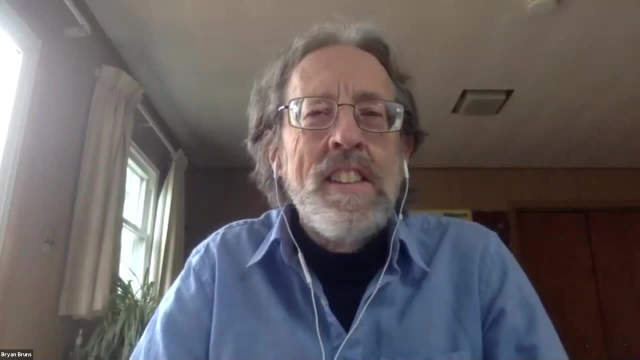 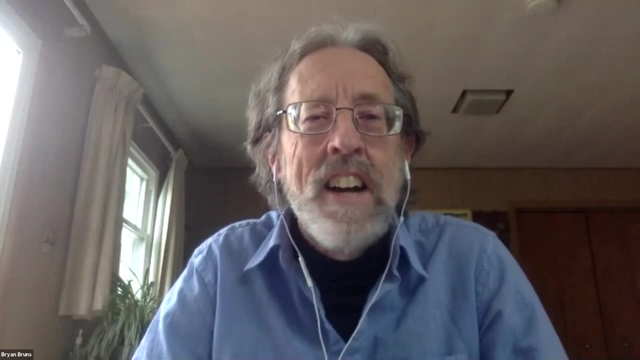 austrum lecture whether you have any comments about, in a sense, the other path, the hard, hard way of doing it, which you know. in a sense, harden's tragedy of the commons was an example of bad science, especially if you look at harden's personal beliefs and some of the stuff that 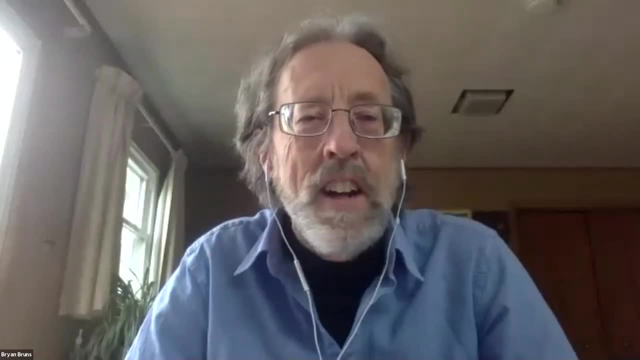 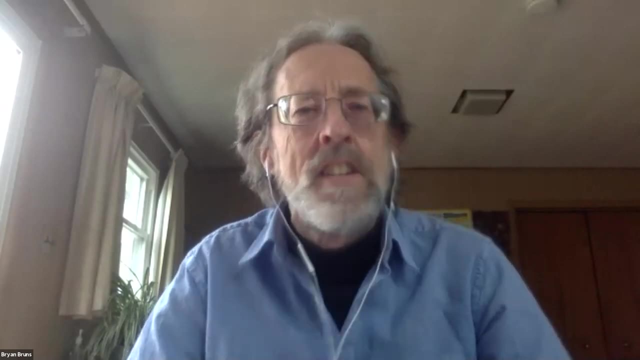 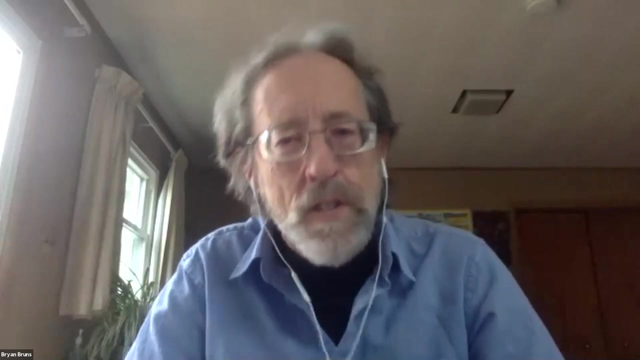 and what you had is lynn and a bunch of colleagues you know spent literally decades building up the counter evidence and reframing the issue. and just so it's not only lynn. another example is amory lovins, who looked at the implications of energy efficiency first. 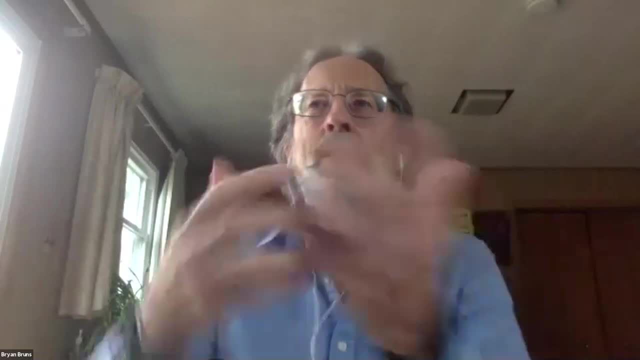 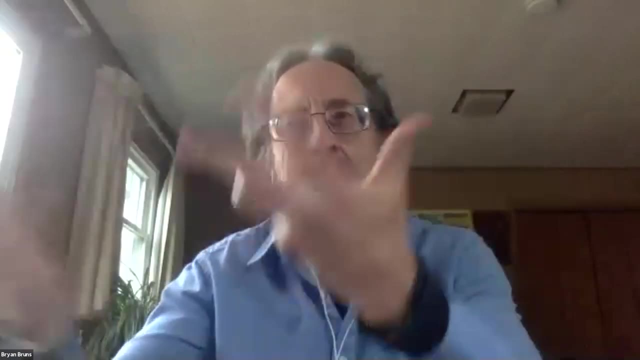 for energy and more recently for climate change. you know the side of things people were neglecting, so i guess there's a question: how do you combine the kind of hard, slow slogging strategy with what you're hoping for of some quick way to come up with authoritative 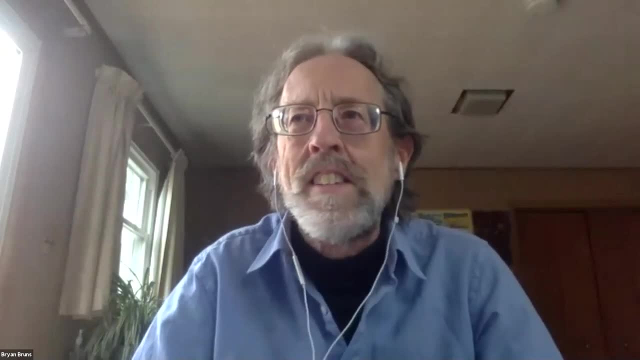 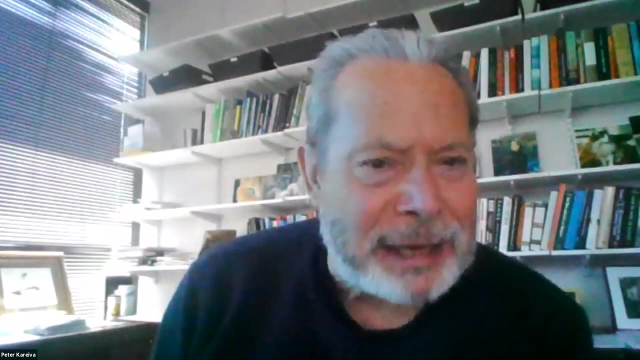 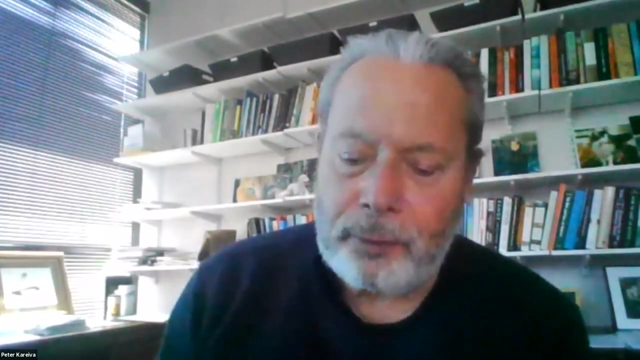 you conclusions about some of these things, you know. so the the hard, slow, slow slogging strategy does work for sure. i mean in it, in it's, it's. it's, it's why we're scientists and it's why scientists respect it. it does work. um, i think what you would do is you would, maybe you would have. 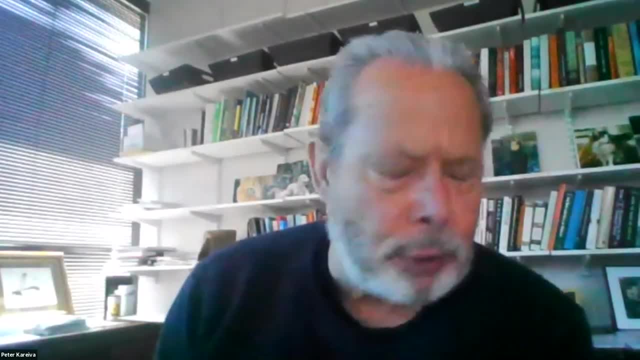 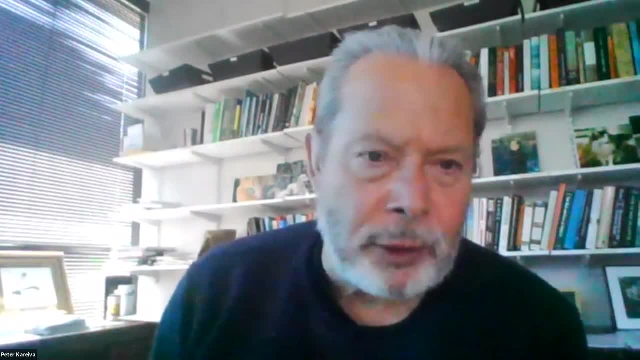 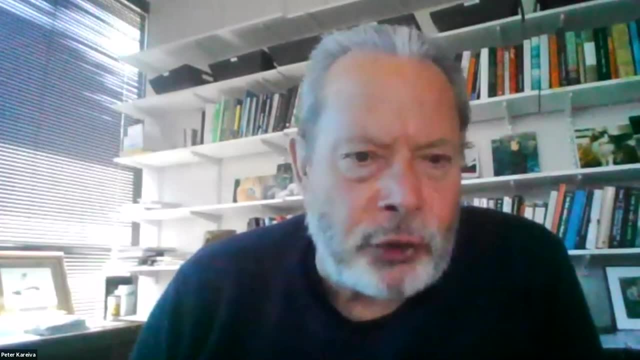 there would be some way of deciding whether it was worth it, whether the risk of getting it, you know, whether, whether we really needed to get things right fast, it was important enough that we give it the fast treatment, or we just let uh science take its course, or the national academy. 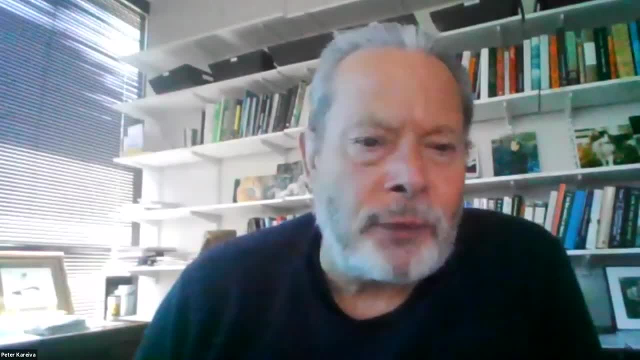 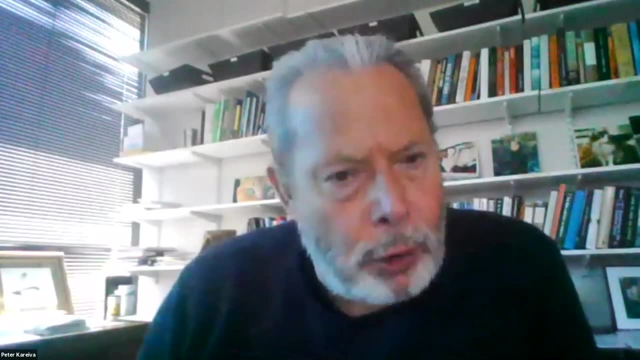 time, so you couldn't, you couldn't take everything through the fast process. um, i think in in you know there have been certain gmo issues that should have been taken through the fast process because they immediately affect the environment and the environment, and the environment and the environment. 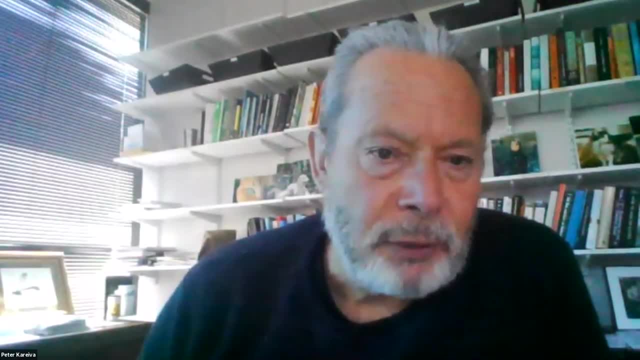 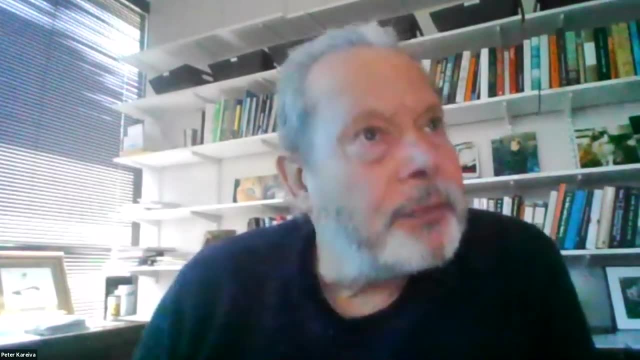 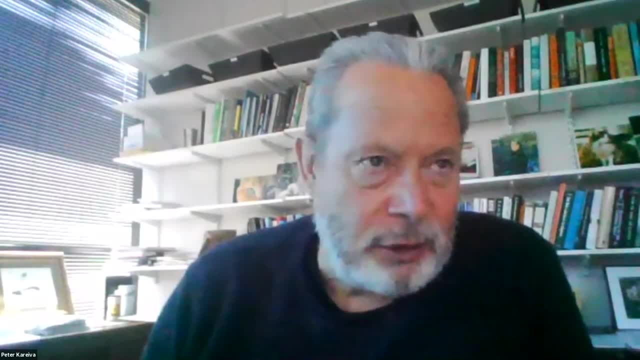 could have been taken through a fast process and you, you would get better at it. ota: i used to do contracts for ota. they put some things through pretty good processes. uh, i forgot what. who killed that, but it was. it was a kind of an in-between. 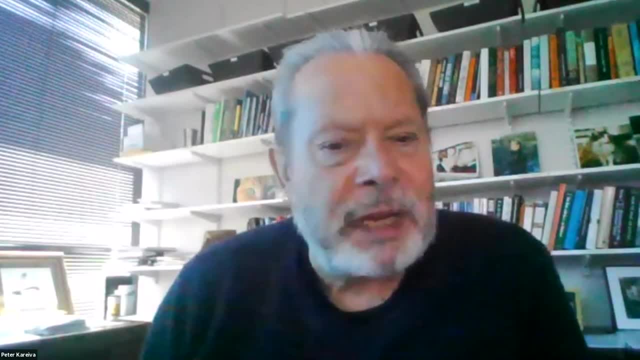 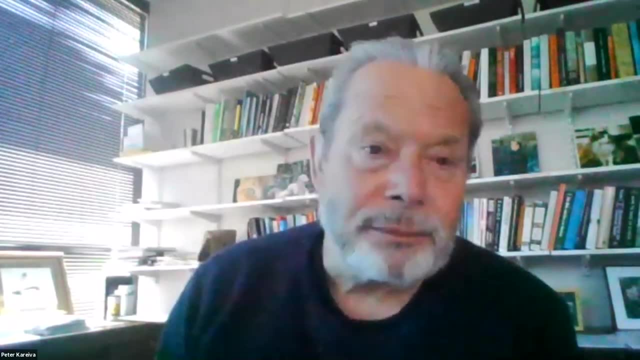 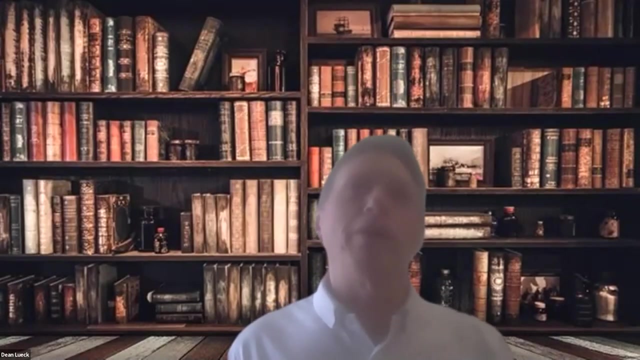 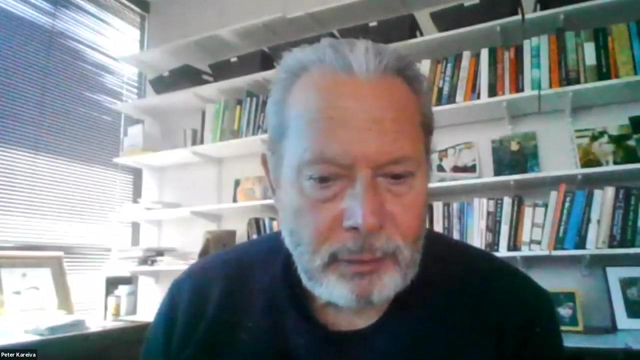 you um institution office of technology assessment, which is a branch of congress. um, it wasn't bad. no, reports are good. no, so we, we have some. we're kind of talking a little bit about institutions that might generate better outcomes, i think, overall here, which is useful. i'm going to go to, i'm going to read you now, peter zing's question. uh, thank you for this. so, 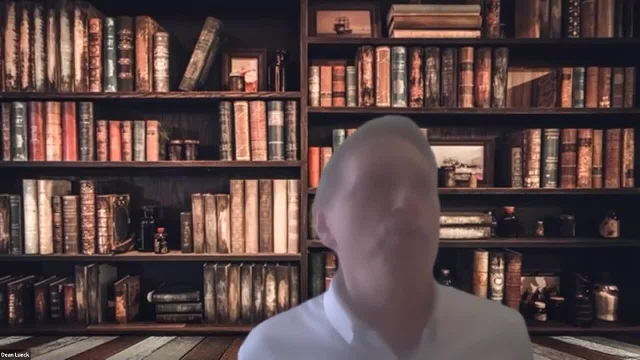 peter, how do you perceive japan's decision on dumping the us economy in the future, dumping fukushima nuclear wastewater into into the pacific, given the gap between public mistrust or trust and the science-based appraisals of low risk? how do we facilitate a better policy? 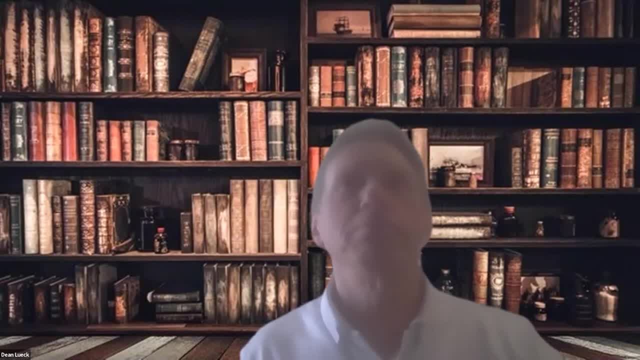 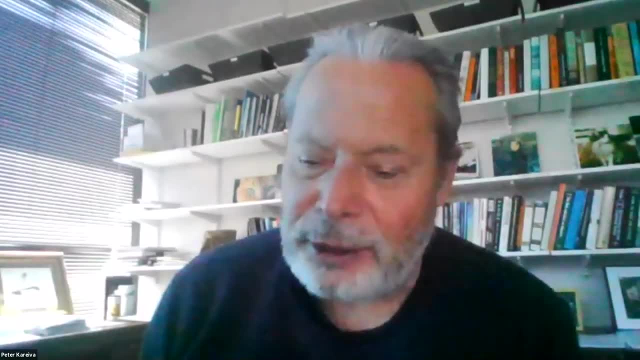 implementation facing public resistance. you know, i just don't know enough about that to comment. i, i, i just don't. one of the things i used to hate when i worked for the federal government is all these letters signed by all these scientists who i knew didn't know anything about it. but we're 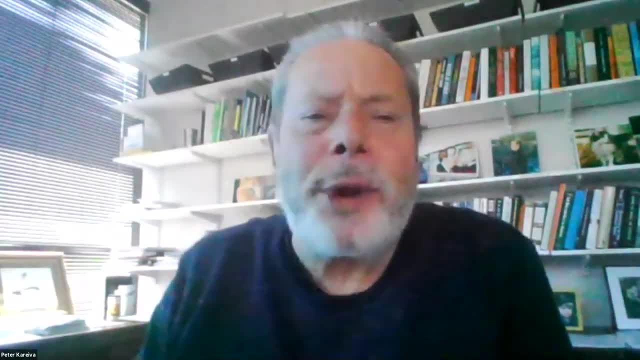 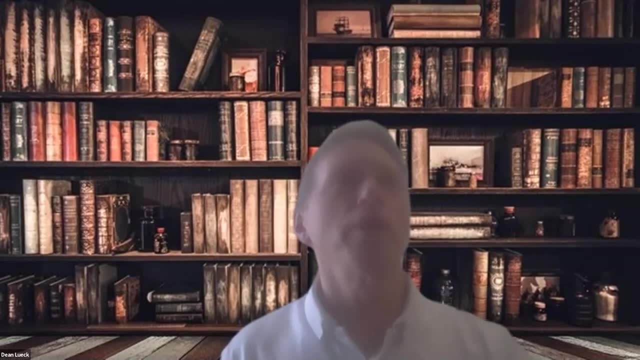 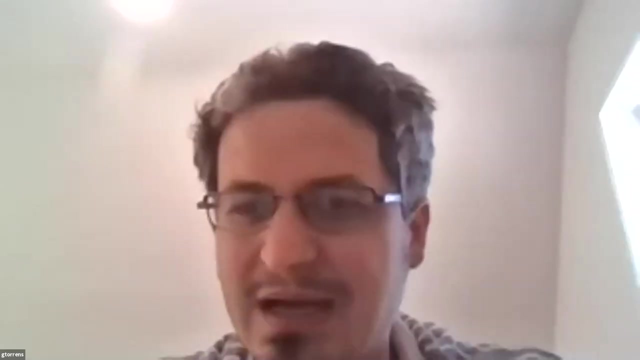 signing the letters. so i, i don't, i don't know enough. i just don't know enough about that. uh, okay, gustavo, do you have a question quickly, before i know you're getting ready to leave, but go, go for it. oh sorry, yes, i like my question because i i have to leave, but um so, um well. 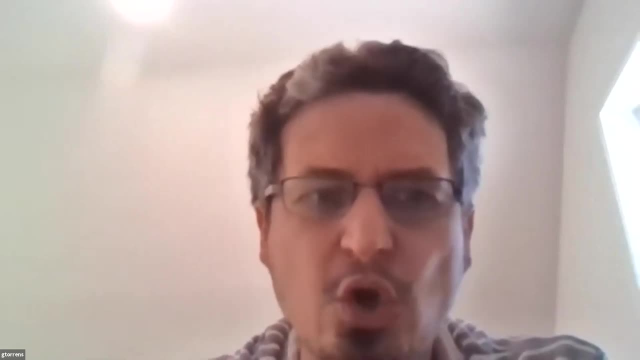 very, very fascinating discussion. my question is: so it seems to me that covid um climate change very different problems. so for covid you really need the fast policy decision, but climate change is more like a slow, slow cooking problem. no, so um, why? so if you're talking about 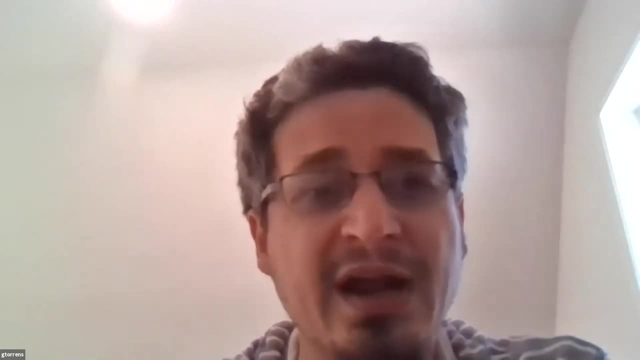 climate change or environmental issues. why don't we go for more gradual policy changes and then we wait for good science to win the battle against bad science among scientists and also, you know, win the heart of the people? uh, in order to get public support? no, so, essentially, 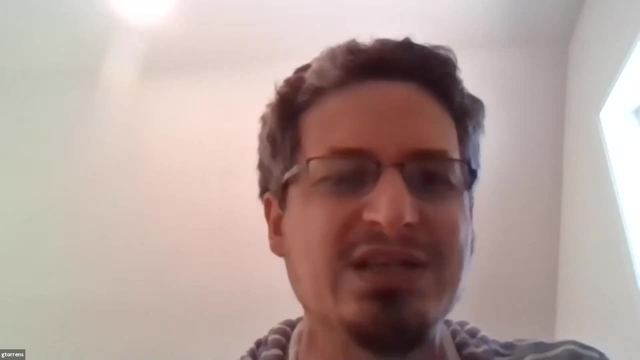 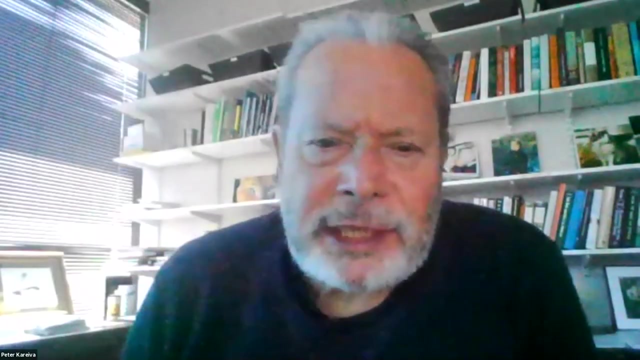 maybe we need to push for more gradual changes and that's kind of the solution. institutional solution, no. so i i would agree that covet is a special case, with its speed for sure. so covet is a special case, i'm not so sure, uh, but my main. 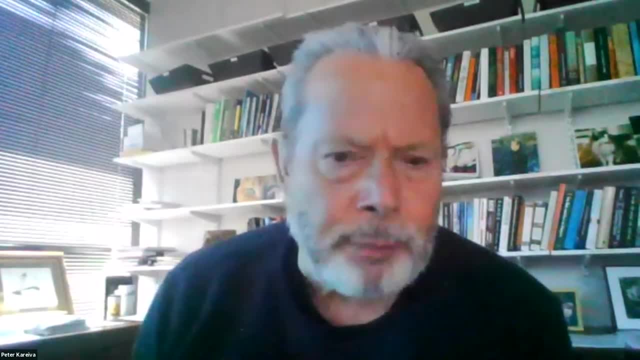 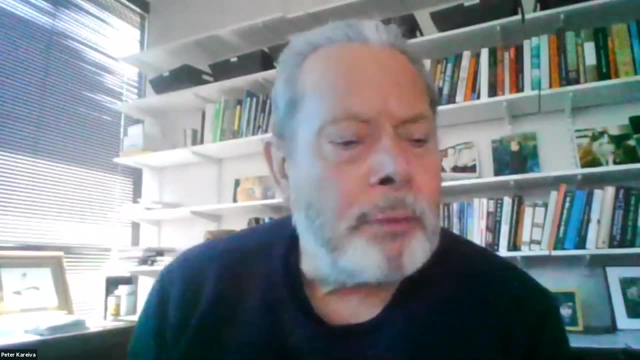 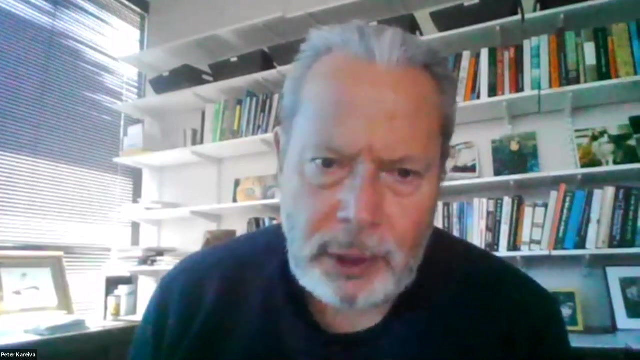 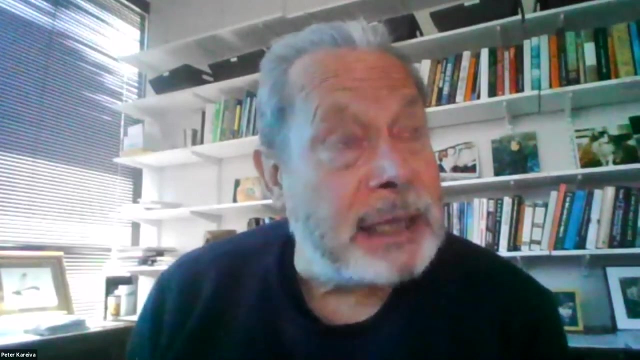 problem with, with the, with the climate science, was the missing the point about the fast, uh, positive feedback loops and the importance of these short lifespan. but even so, what, um? the policy cycle in california could be pretty rapid, so give you an example. right now, noah, um, noah has a federal policy to encourage aquaculture. and they've created what they are called um aquaculture opportunity zones and those and they've designated southern california coast as an opportunity zone for economic development and aquaculture. california is going to make a decision on that as a state on a time frame of a year. 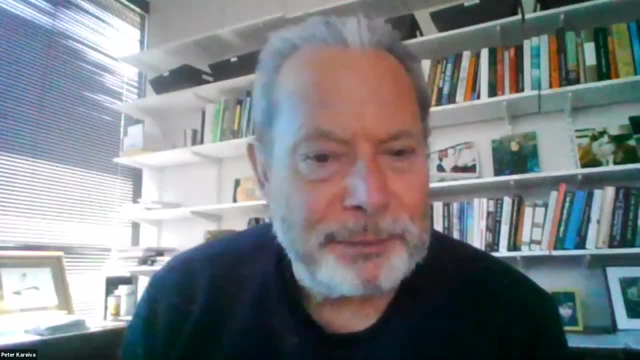 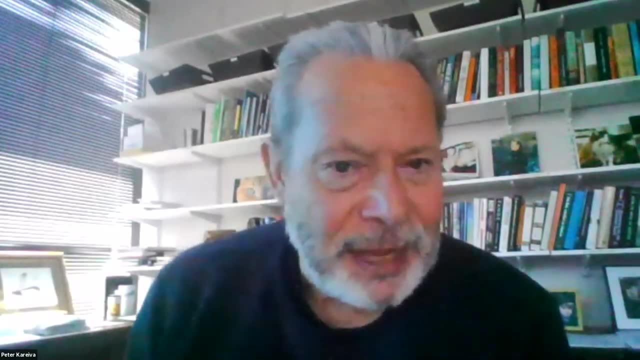 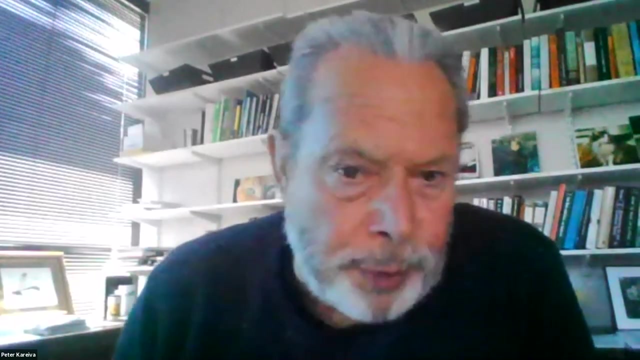 there is a fair bit of science that applies to that. there's a fair bit of science, there's a lot of activism on both sides and that's an example of an intermediate. so the arguments in favor of aquaculture are lower emissions for food production and reduces pressure on wild stocks. the arguments against it are nutrient. 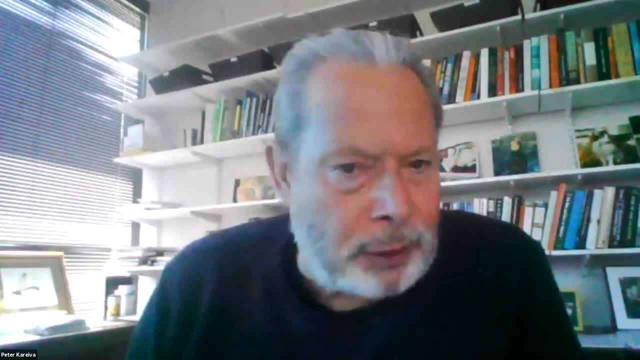 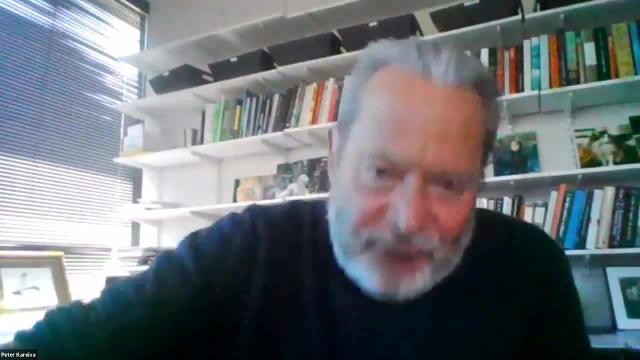 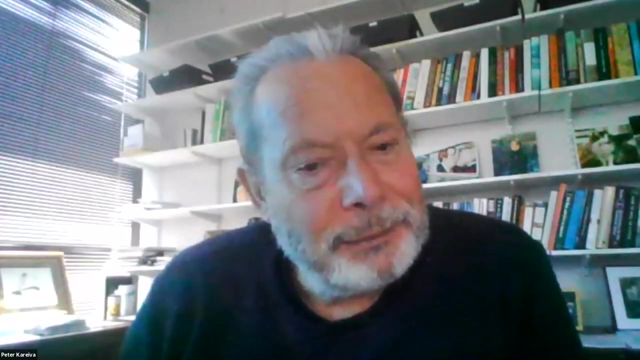 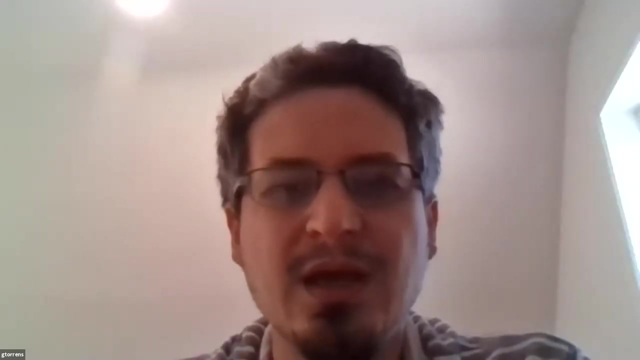 and habitat following. there's lots of papers, there's, you know, um. so it's a. it's a case where a state is responding to a federal and has to make a decision. that is pretty significant and that would be an intermediate time, just quick follow-up, could it be sure? but now we're talking about the question of science. 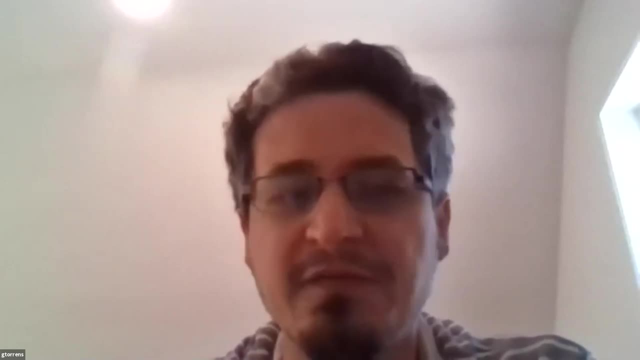 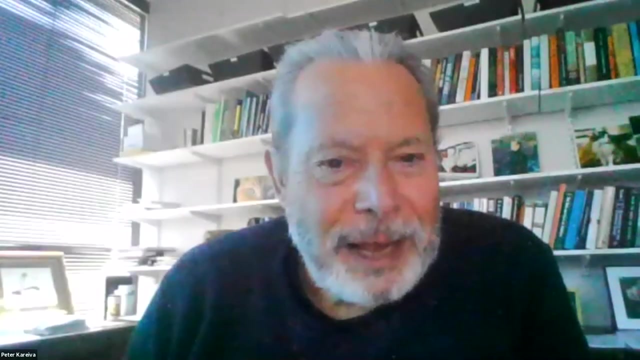 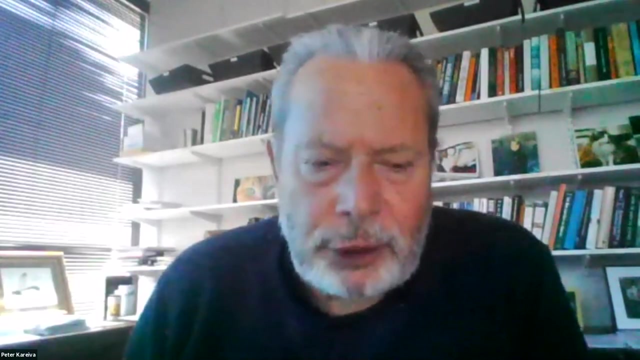 essentially we don't know, or it's a question of just conflict of interest. so different groups, they want to push in different directions, but they already know everything though. yeah, i mean, um, that is it, but the, the papers that are in this, in this aquaculture literature. 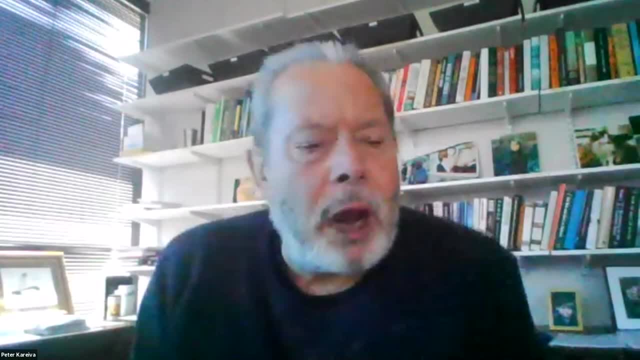 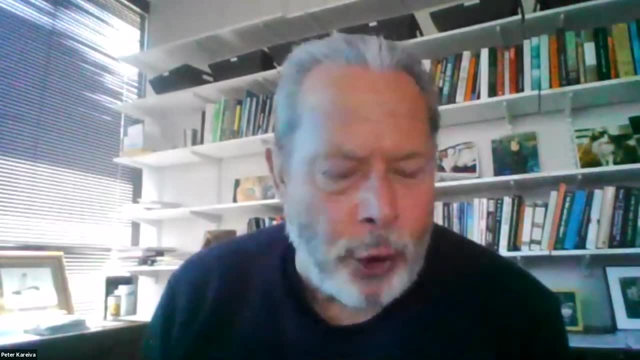 um, you know the papers are are, i suppose, like anything. they have some bias, but it's it's. it's not like the case where you have maybe the oil industry funding science to get some results. It's not like that. It's much more people genuinely 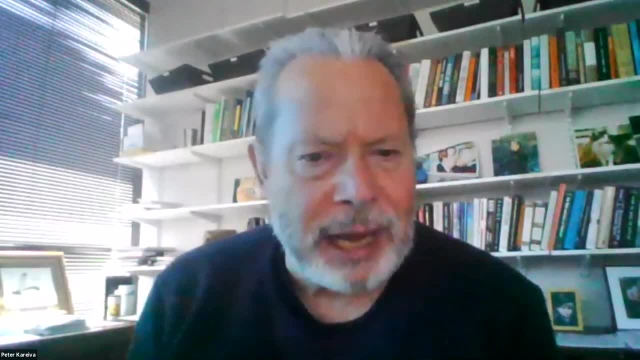 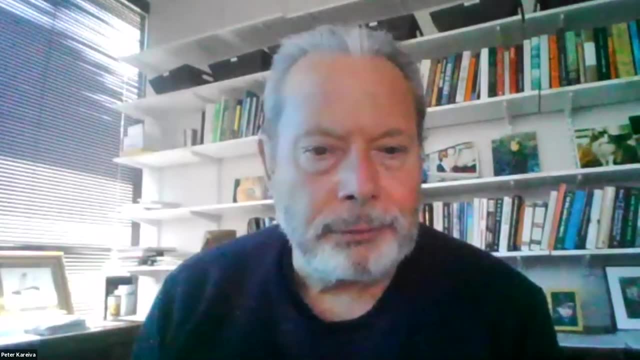 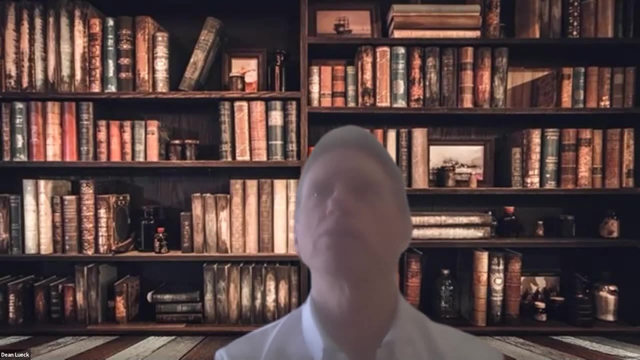 curious about aquaculture's impact. What you described could certainly be the case with like energy trade. energy We have. thanks, we have just a little bit of time left. I know Tom Kuntz has a question. Can you ask it, Tom, or do I need to ask it for you? It was really more of a. 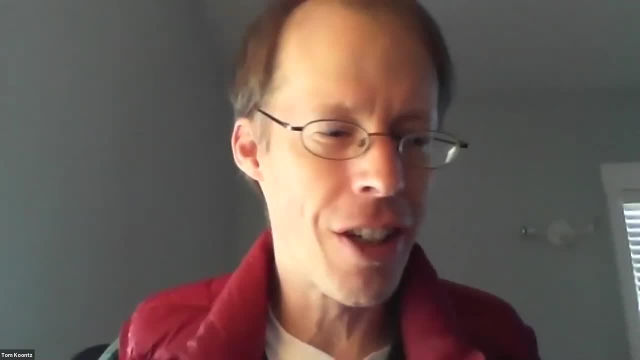 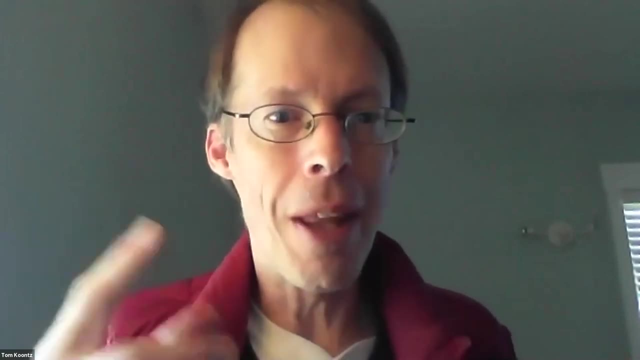 comment. I'm thinking about the Knowledge Commons, the collective action challenge of getting people to do the work. You could imagine maybe asking all the scientists to do one more peer review every month, but then it's just going to come out of our own time- versus funding something like the OTA. 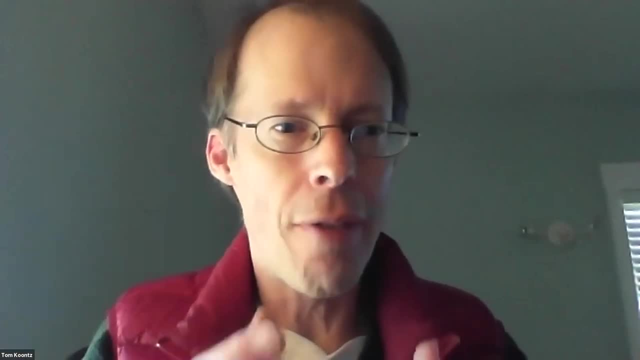 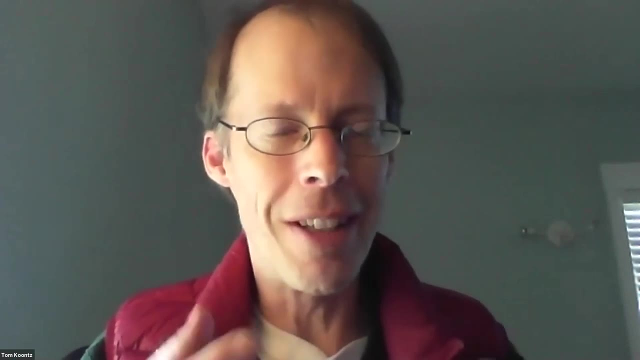 Why is it not funded? Maybe no congressperson saw enough bang for their buck, even though it would help everybody. So I think this sort of leads into questions about the Knowledge Commons and providing. this thing is hard to do. So that's just an observation. I was wondering if that 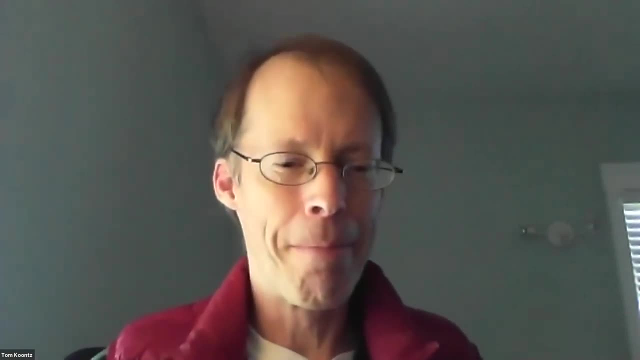 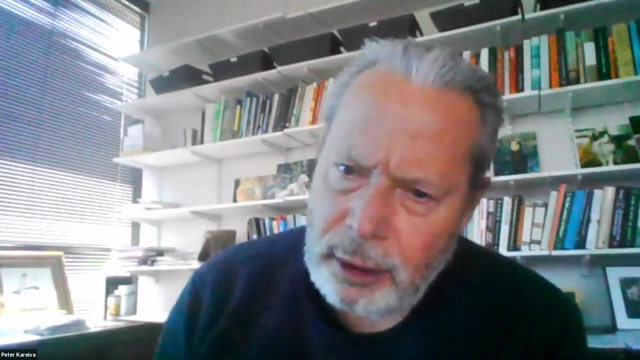 connection might be seen there, but not a specific question. I guess You know, I think you know people do people normally sign up for National Academy, which is a ton of work Because especially with- you know, cultural change, most scientists feel a. 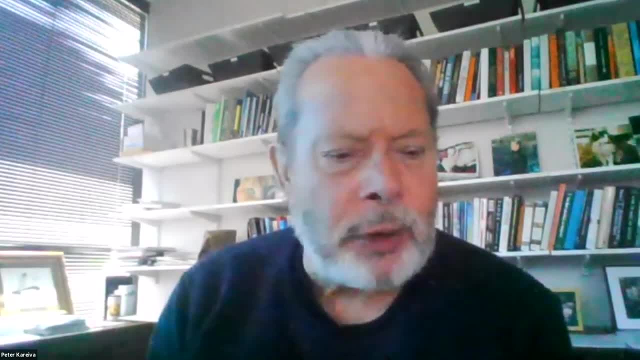 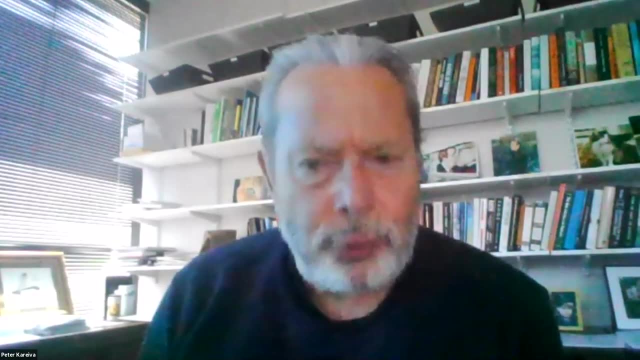 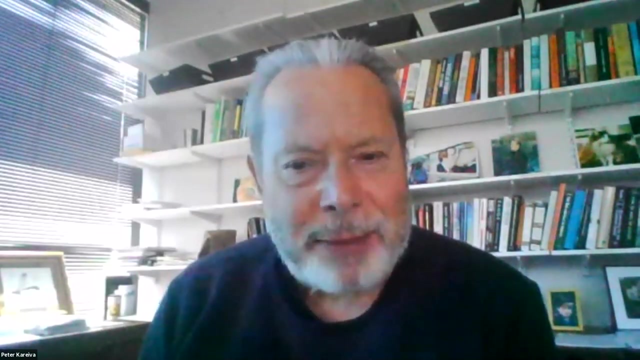 social responsibility. I think if there were an adequate filter so that you weren't asking for that extra effort to review a paper but to deal with an issue where a decision was to be made, I actually think the community would, would would behave well. Maybe I'm naively optimistic, but 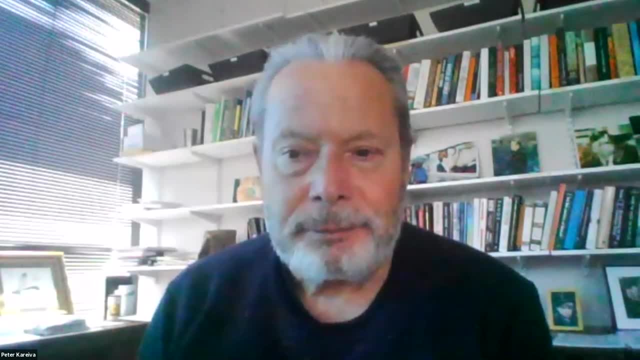 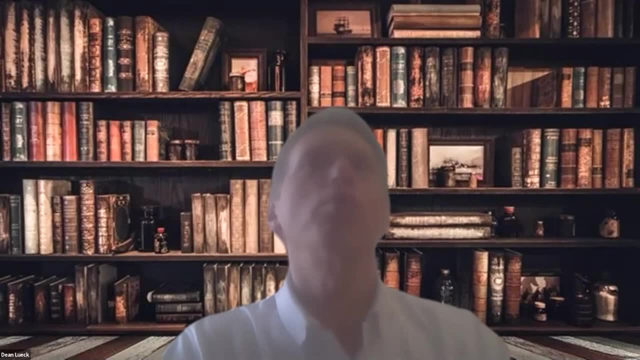 I've seen it behave well for the National Academy. Let's see we got a couple more left. Let me see I'll go back to chat. John Eldon, you have something, Herbert, excuse me? Yes, we'll get. if John ready, then we'll go to Herbert. 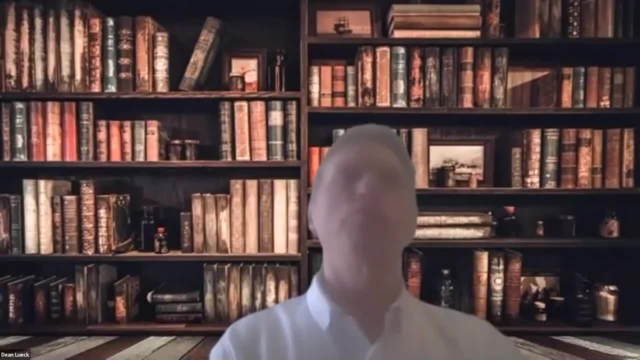 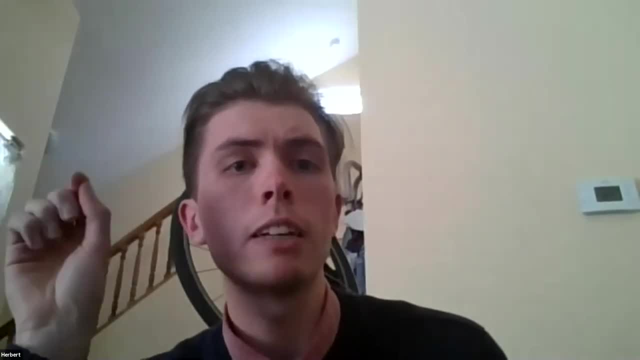 Oh, I'll pass it off to people raising their hands. Okay, Herbert, go for it. I'm sorry about that. So you, we've been saying public in the like this: in general sense, is it really the public we need to target, or is it specific actors in the? 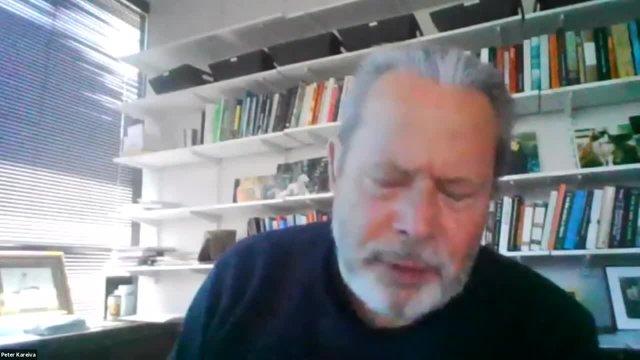 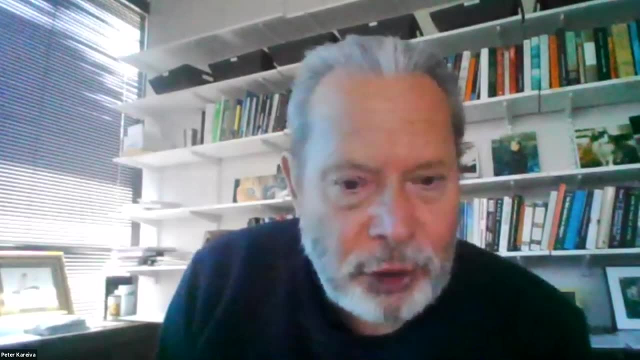 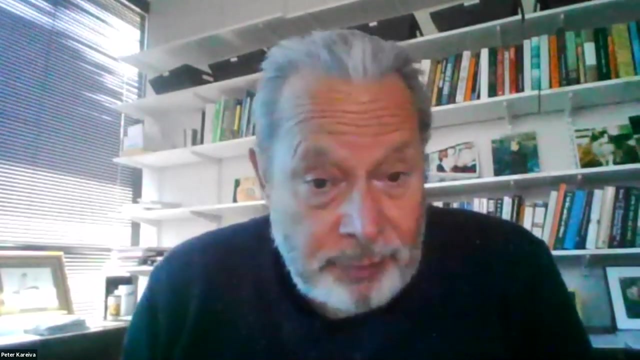 public. It would you know. I think it would be specific actors. I mean, sometimes it is the general public, but in some cases, like in this aquaculture thing in California, it's the assembly. you know it's not a single person, but you know what the body is going to be and what. 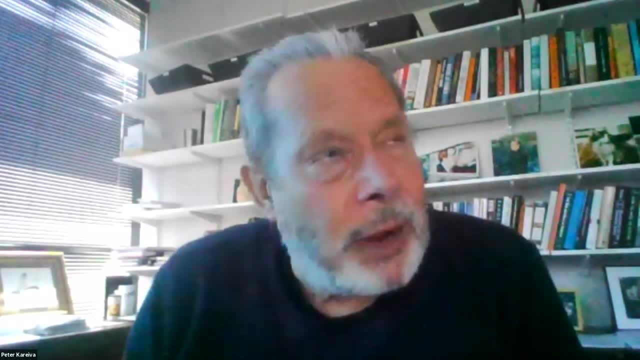 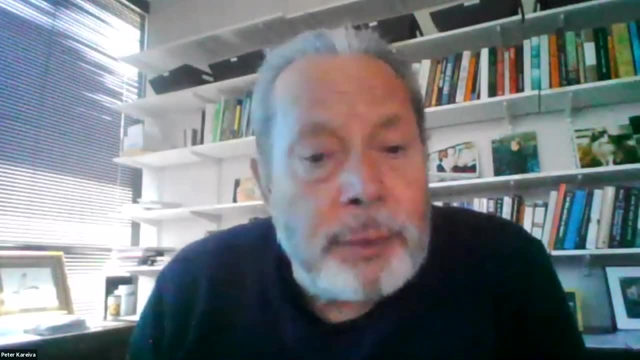 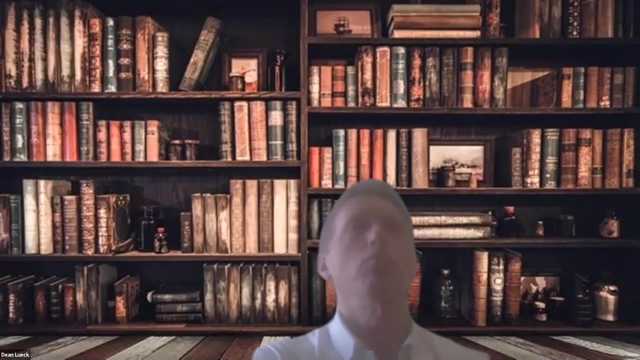 they're responsive to. So it's not a- you know, it's not a single bureaucrat or a head of an agency, but it is the assembly or something. In other cases, for GMOs it probably is the public. For a lot of the GMOs it is the public, But couldn't you also say that it's just the? 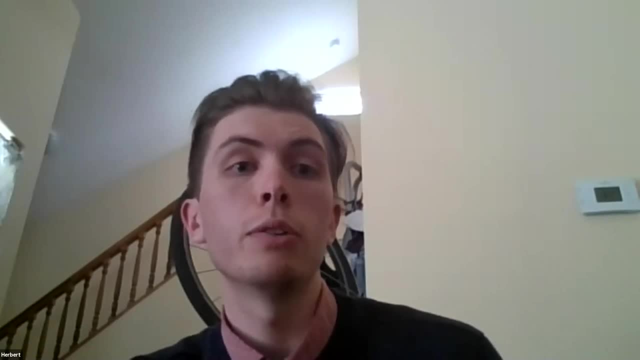 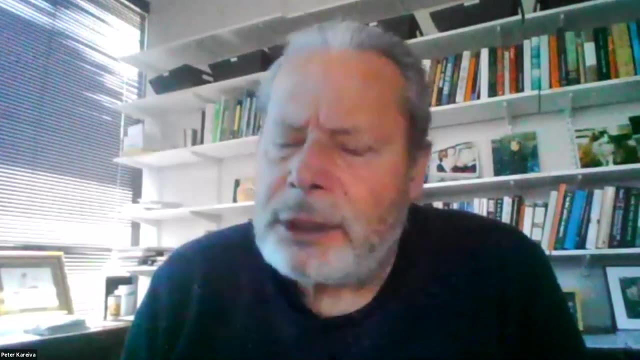 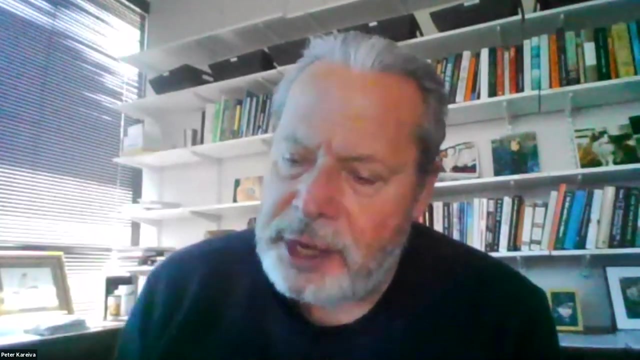 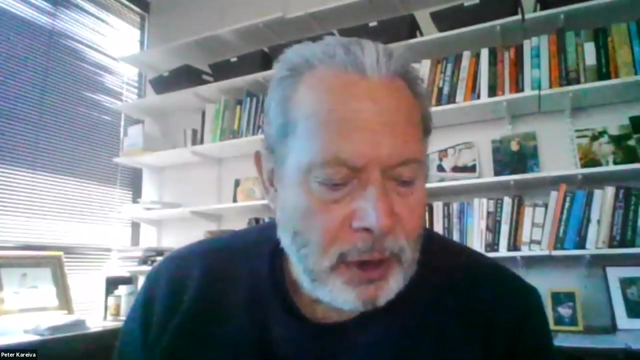 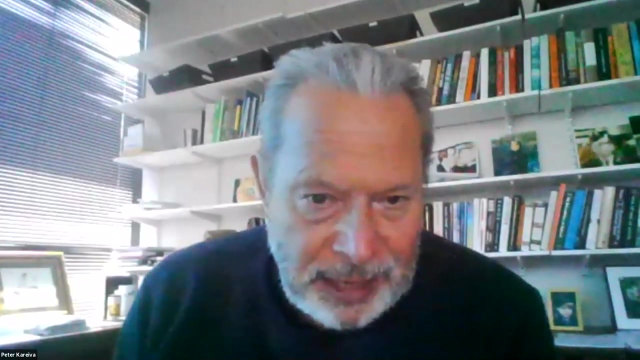 like policymakers, or it's the like USDA regulators. You know, even when we did that nationally. I don't think you could say that for GMOs, because the food industry will label things and market things on their own, independent of the regulatory agency, in a way that has implications for how the public responds. 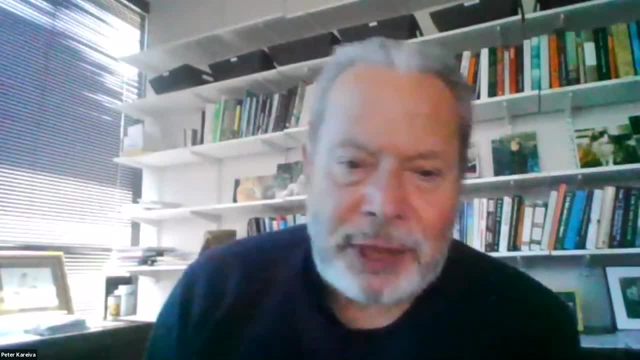 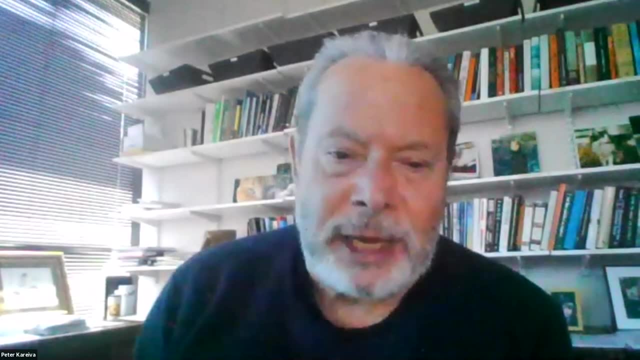 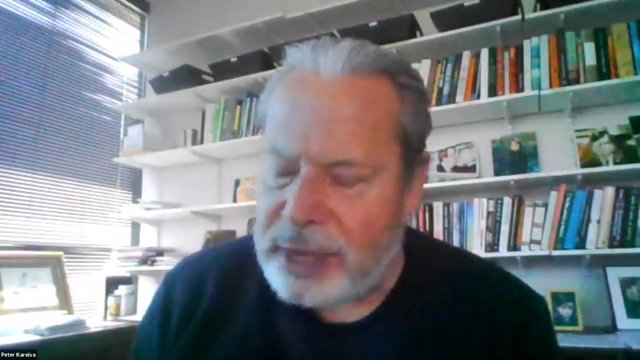 So the USDA could say we have to label something right, And that would be a big decision. But alternatively you could have labeling as a marketing strategy and you could really drive sort of what happens with food systems just through, frankly, marketing and labeling. 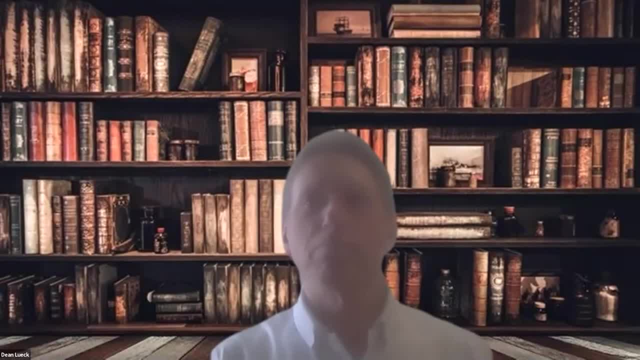 Yeah, and then we have. I want to try to move to the last. we have three questions left. We'll try to go through those quickly. I think we'll stop with those three and then we can hang around after. So we're going to go with. 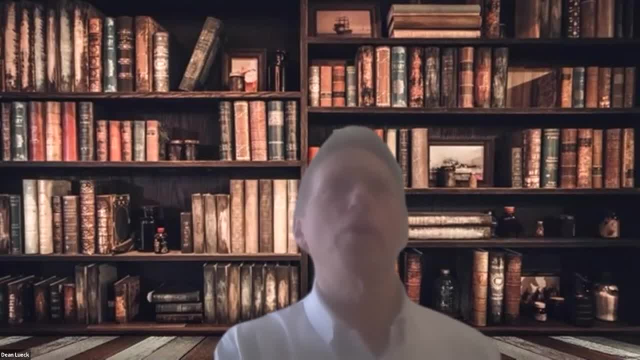 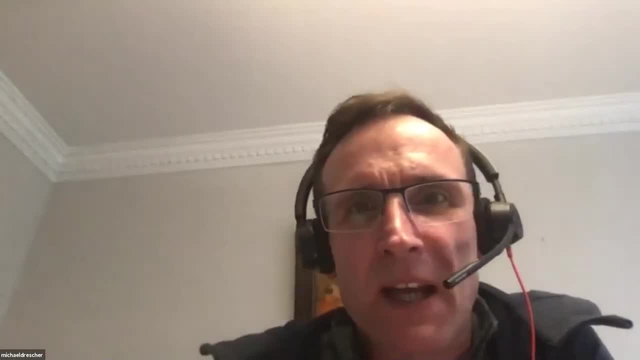 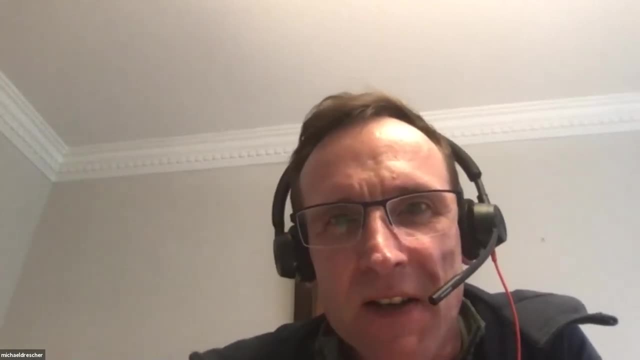 Michael Drescher, Macy Brammer and Vicky Maretsky, in that order. So, Michael, Hi, Peter, Good afternoon. I'm really struck with all these bad science problems, And I mean you brought up this example of, of course, the 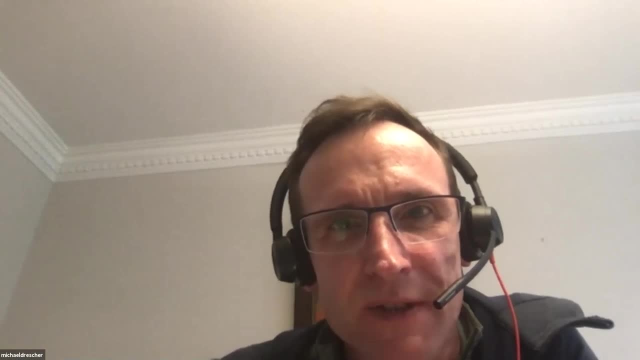 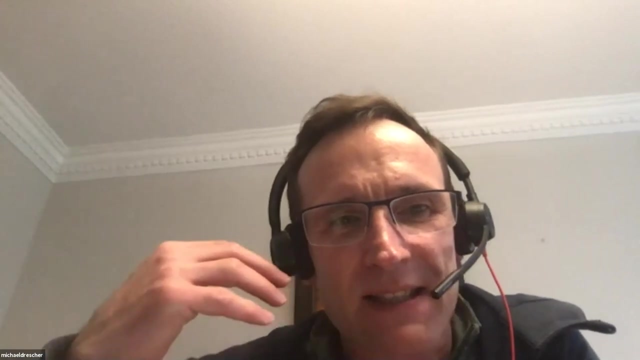 the vaccination story and and autism, and how difficult that is to to rein that in, And I- I compare the two- kind of a genie, The genie is out of the, out of the bottle, And how do you ever get that back. And so is that not then becoming more than a science or a natural? 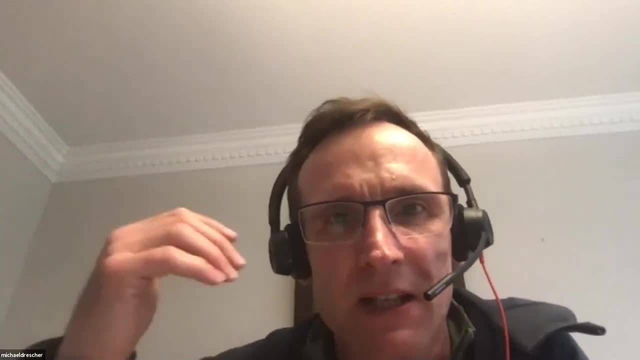 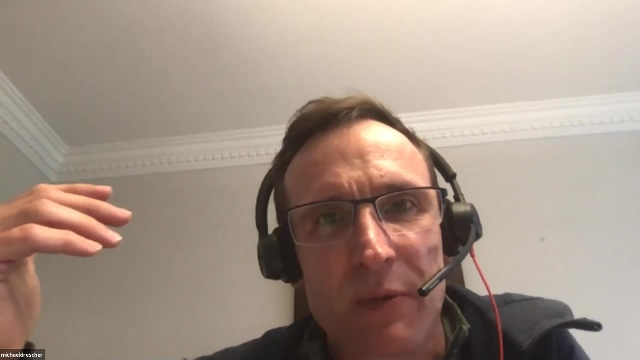 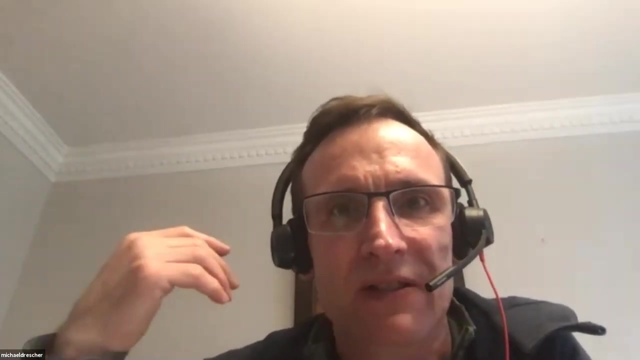 science problem or, in that case, health science problem, But it really asks for a much closer um cooperation between natural scientists and social scientists to really understand these problems as um social problems. How, how, how, how these stories are formed and then taking on. 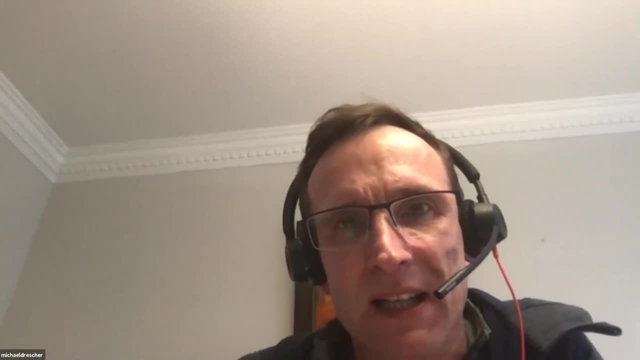 a life of their own in the public, And- and we as natural scientists, we're not trained to do deal with that. But there's different, different skill sets, expertise and knowledge um that we require to um to deal with these situations. 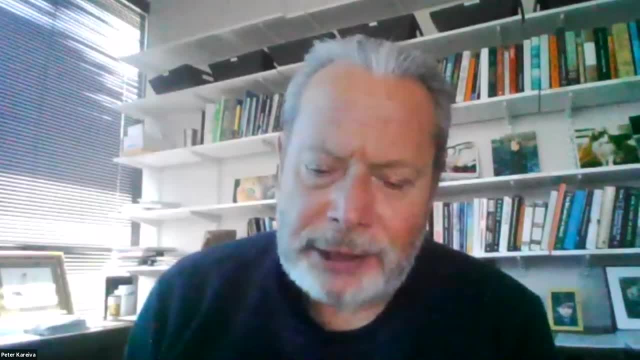 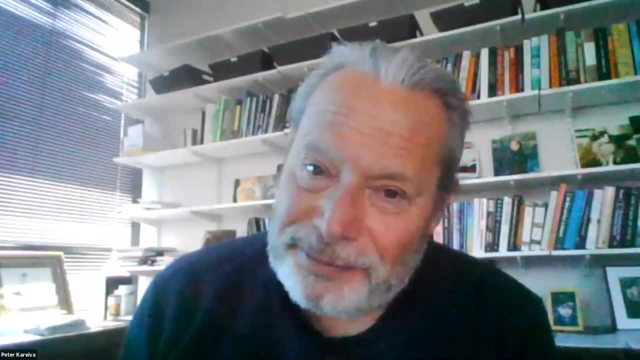 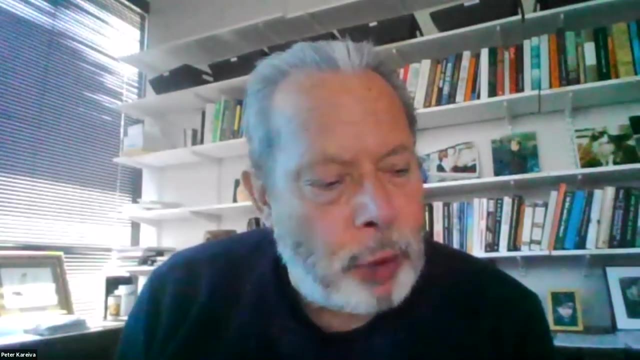 You know, I, I, I agree There is a real social science, because I think, um, social science could have anticipated some of these things. thought about it, And I think social science, uh, insight, would help a lot in terms of anticipating. 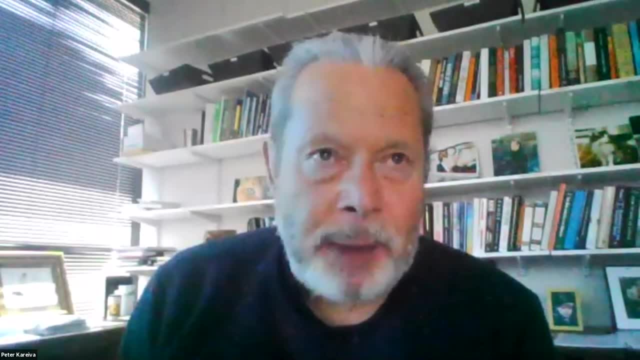 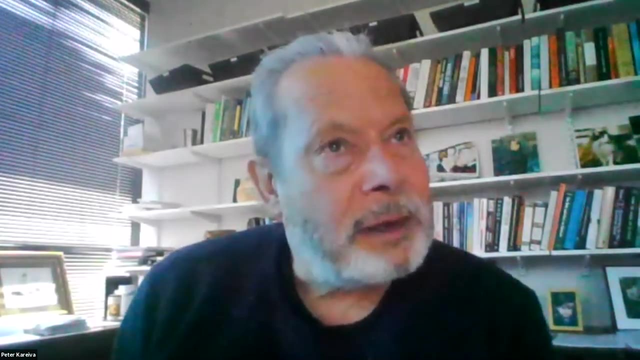 what's going to happen with these and responding faster in terms of of um, like it's, it's, it's very um. scientists form panels of experts. That's not the way you want to address some of these genies out of the bottle. 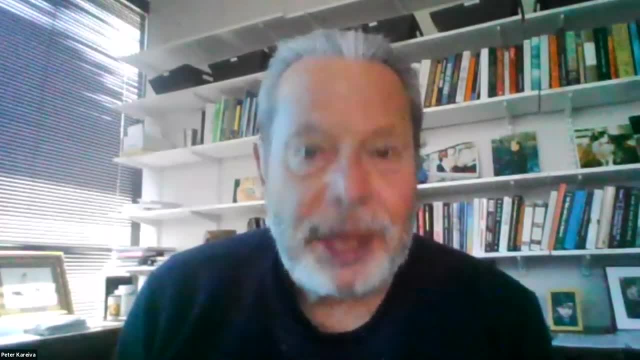 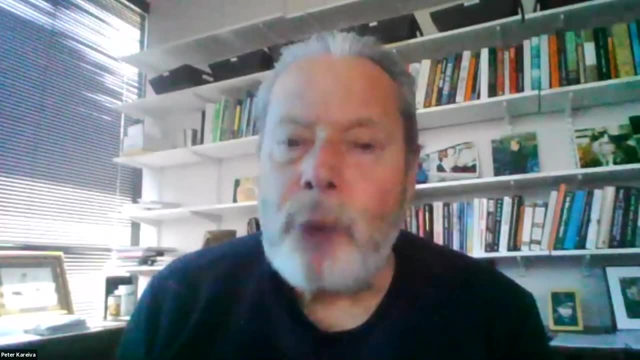 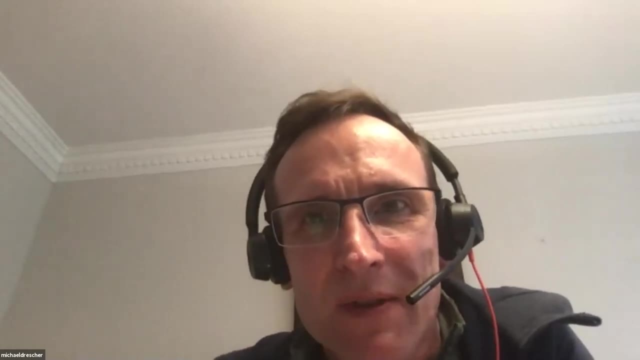 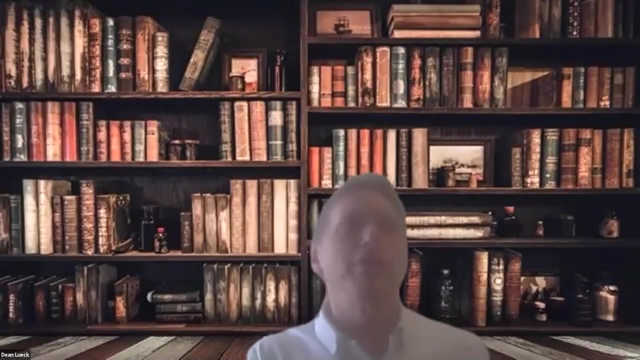 You don't just form a panel of experts. A social scientist would know that and and be able to uh set up a process that wasn't just panels. But uh, Michael, it strikes me Sorry, can I just, Michael, because we're over and we've got two. Okay, sorry, Sorry, Thank you. Hang around after and hopefully connect Macy Brammer and then Vicki Maretsky. 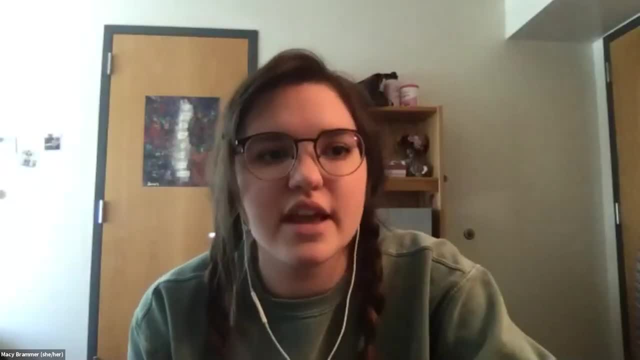 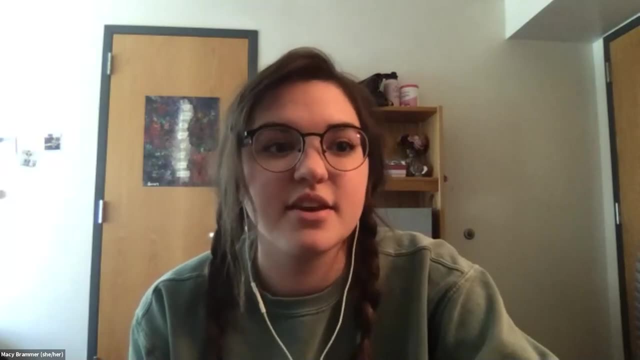 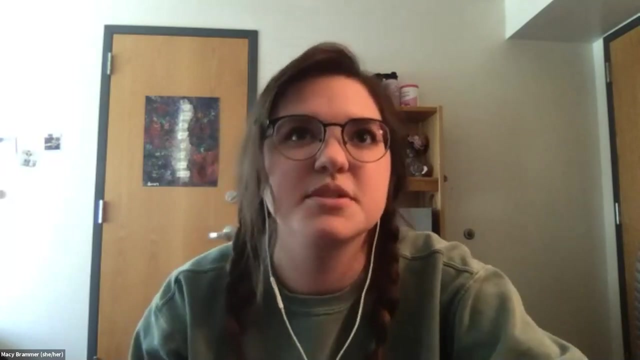 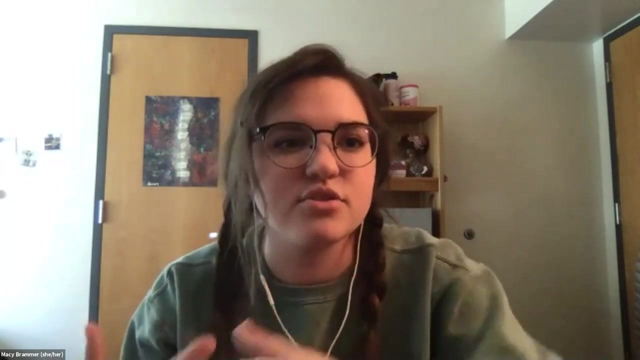 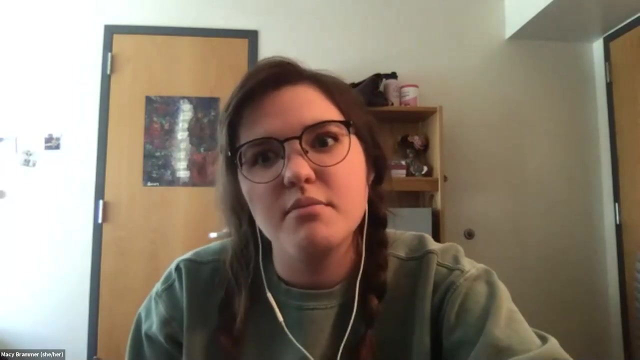 Hi. so I was wondering. you mentioned that little anecdote about a time that, like a group of lobbyists, were saying, oh well, we just said that because it would help us raise the most money. So, when it comes to political actors specifically and specifically, like individual politicians, like congresspeople, what would you say we should like, as constituents, expect from them in terms of, like trying to get the best results for maintaining that balance of environmental quality and, you know, positive economic outcomes? 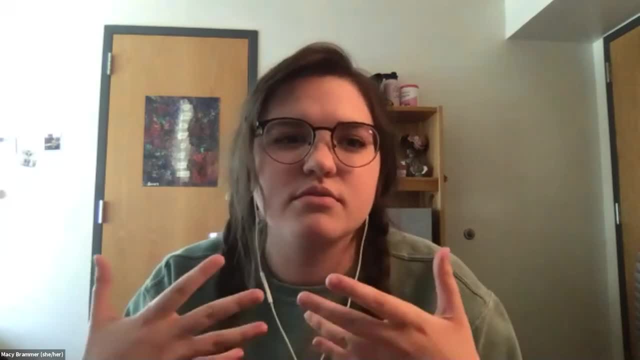 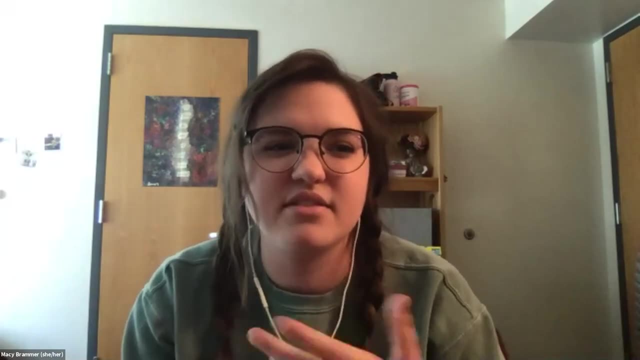 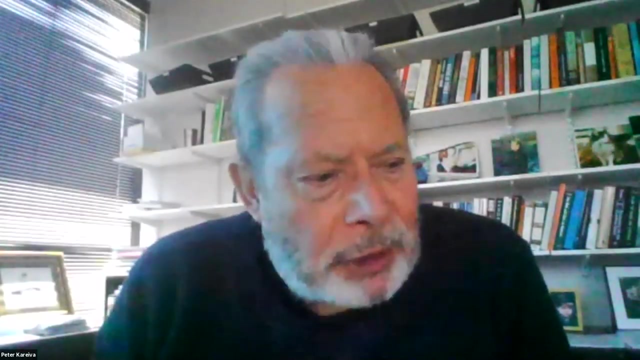 If that makes sense, Like, what do we want them to really have? How, where we want them to get their information from, How? how should they act to, like, best make the right choices that are informed by science, Right? Well, you know the, you know Congress and senators. they get their information from their staff. So it's really through their staff and it'll get it directly. 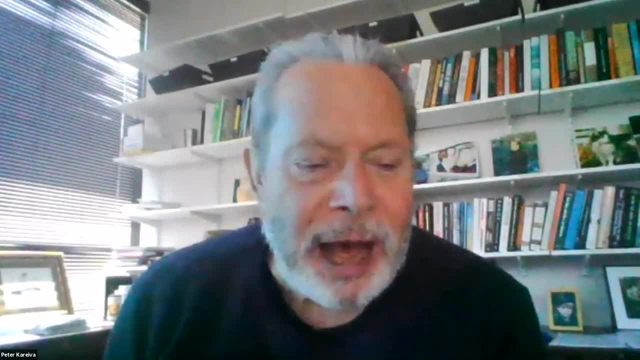 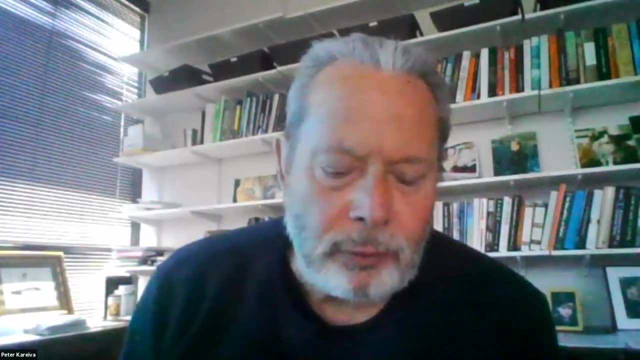 And it's, and it's by the interactions with staff. I wanted to that exact anecdote. I told you I want to represent it, Okay, Really accurately, because I think it's insightful. This was about taking out dams. The it was a single, it was a biologist who I respect, is a very good biologist. 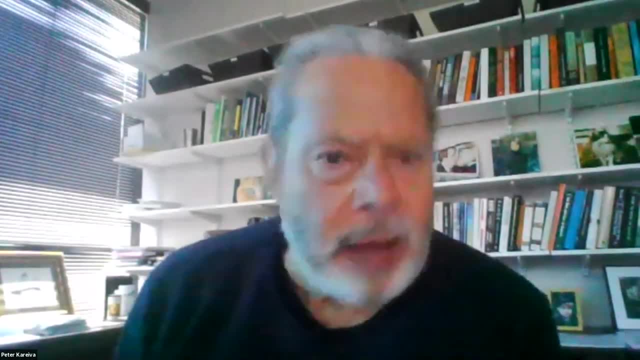 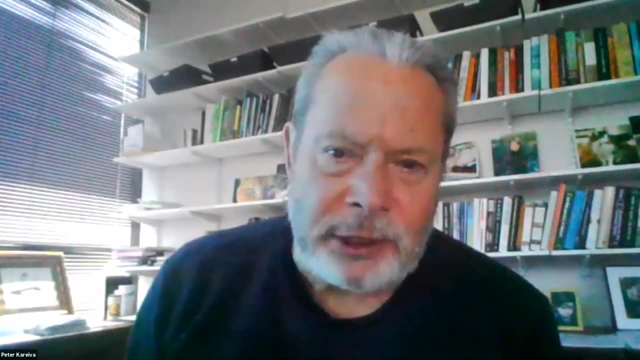 And the mission of his NGO is to get rid of dams because they want free running rivers. The only lever to do that is through the Endangered Species Act and a federally listed salmon. So the objective is to have free running rivers. the lever 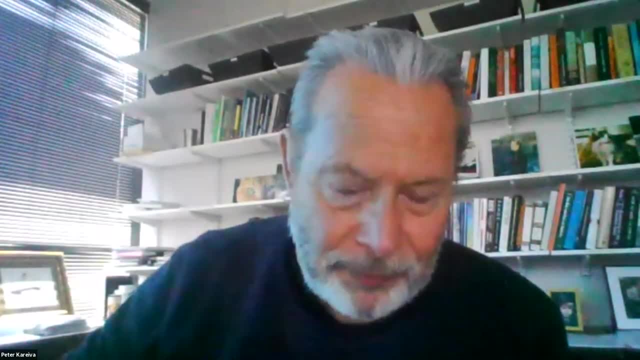 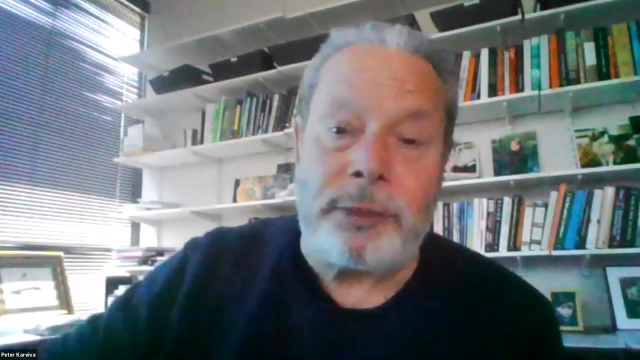 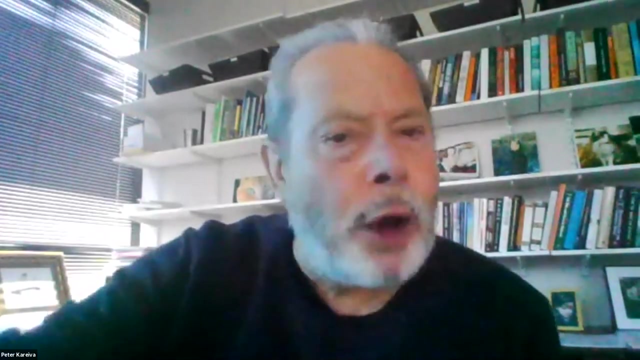 So the objective is to have free running rivers. the lever is Endangered Species Protection, The data concerned pit tags and what happens to salmon. He was just being honest And you know I was saying: you know, you guys know what's happening with salmon. 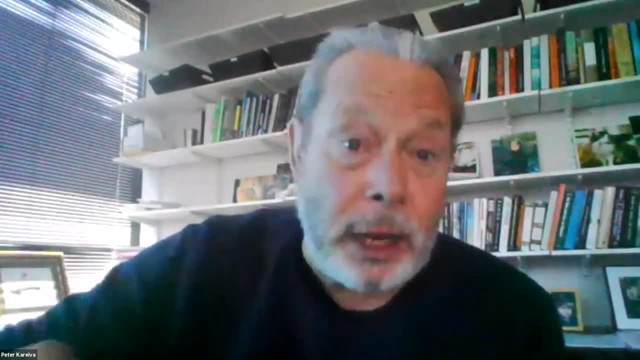 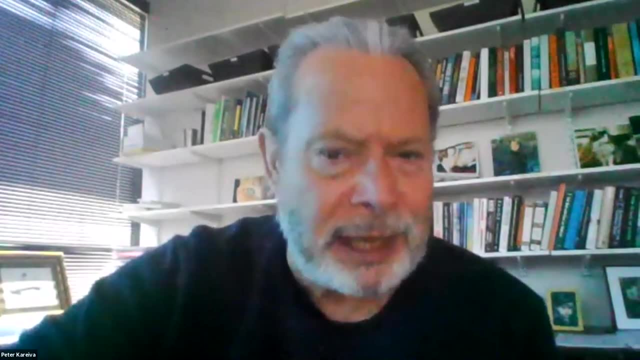 And he was just actually being honest and smiling and saying, yeah, he does know that, But to him it's not about salmon, It's about the river. It's just at the point of entry. He was the Endangered Species Act. 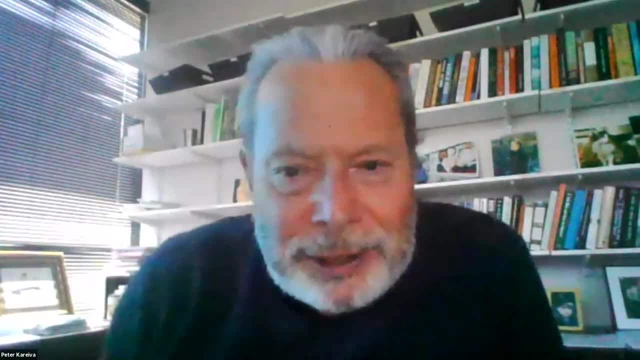 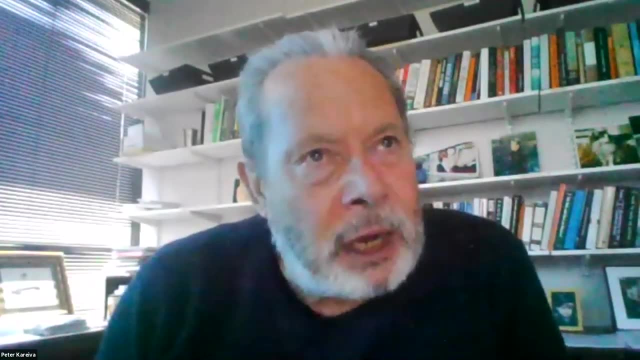 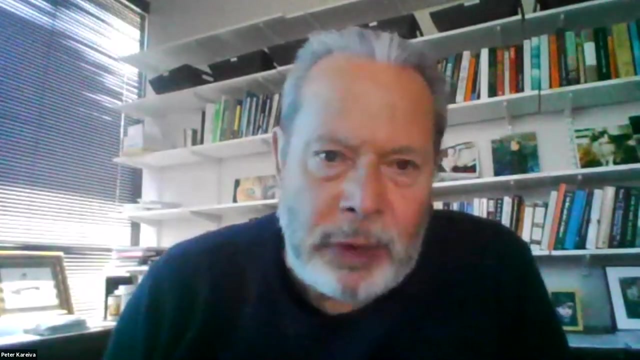 That gives a little richness to the story. I mean, that's actually and I respect this. I'm still friends with him, But I thought it is insightful because many times, the laws and the regulations that are being used are written for one purpose. 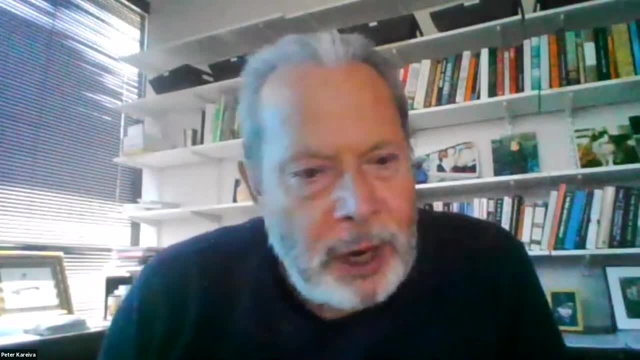 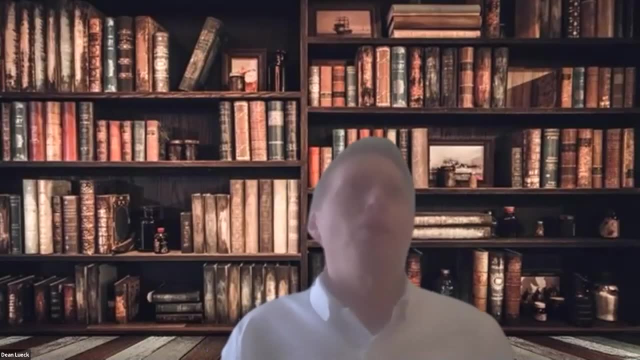 And the objectives of whatever the activist group are totally different. Yeah, Yeah, And I don't think that's uncommon. Yeah, No, that's a great anecdote, Thanks, We'll let Vicki Mretzky have the last question. 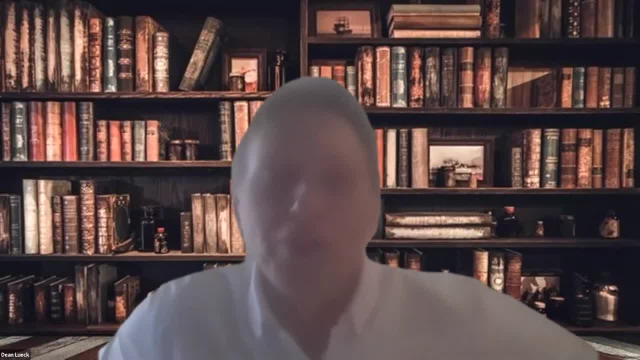 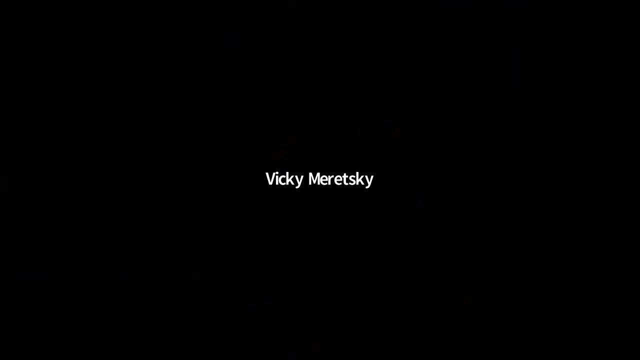 And then, when that's done, feel free to. we'll give Peter his due applause. Then we can hang out and visit informally Vicki. Thanks, Dean. I'm going to yield my turn to back to Michael because he was headed in the direction that I was interested in going. 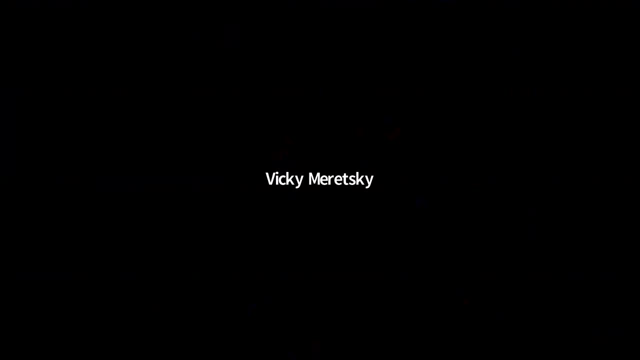 I'm really concerned that, as scientists, we are not the right people to be spearheaded, And I think that the work that you have done is fascinating Work designed to try to bring the public back to something that we think is the right place for the public to be going. 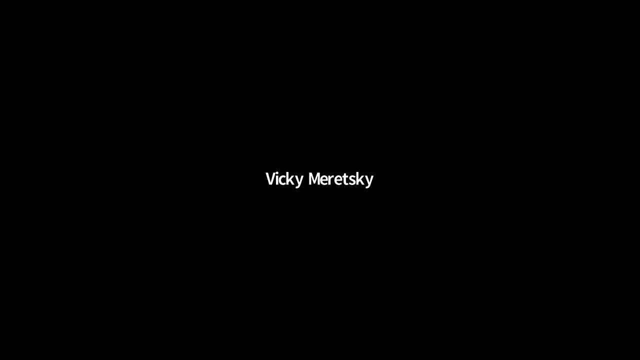 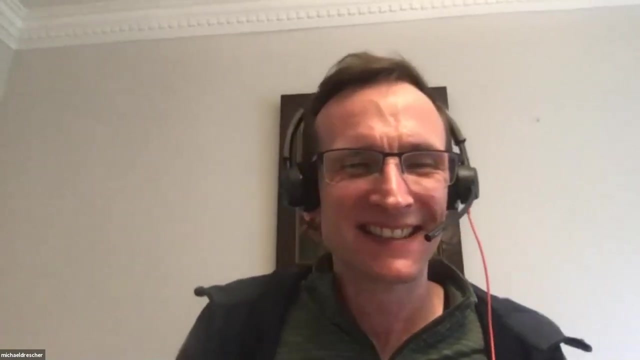 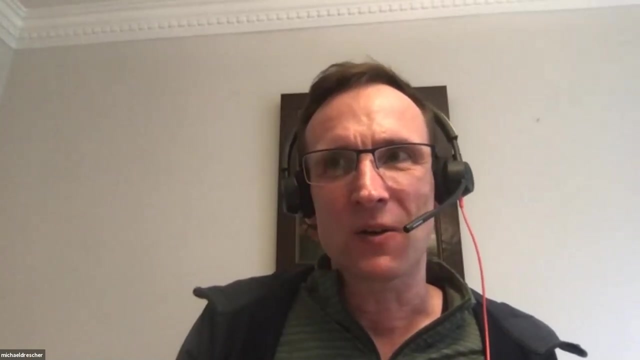 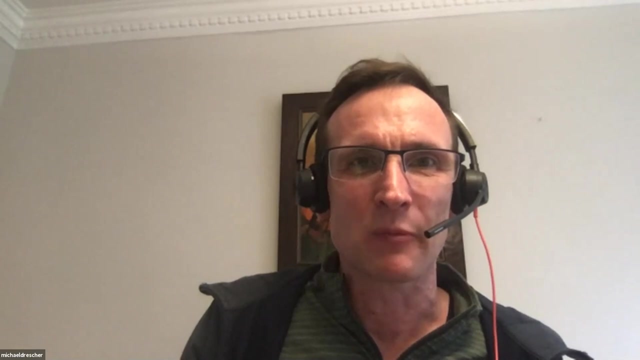 And I'm interested in terms of what supporting collaborations and what supporting skill sets might be there. But, Michael, if you want to craft the wording on that better. Thank you, Vicki, But I mean, what would I say? I mean, what I wanted to say is that I continue to be perplexed how, on an ongoing basis, how bad communication is also of governments with the public. 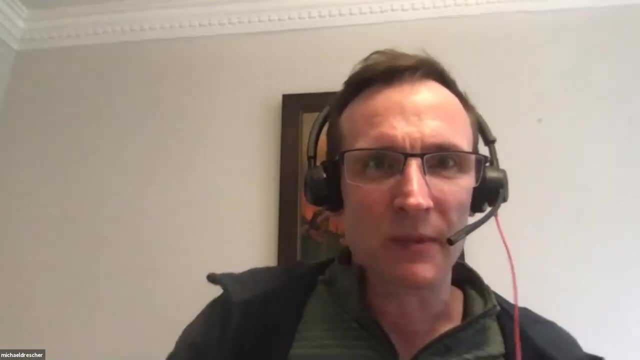 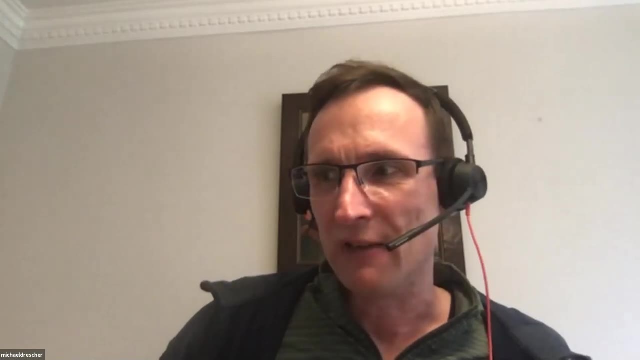 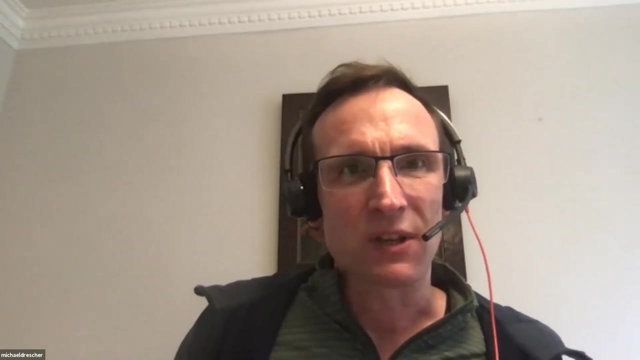 And the COVID example was brought up a couple of times, And that's a great example from us here in Canada, where we have, of course, as in other areas, vaccine hesitancy, And then part of that is that there's mistrust in science and mistrust in the government. 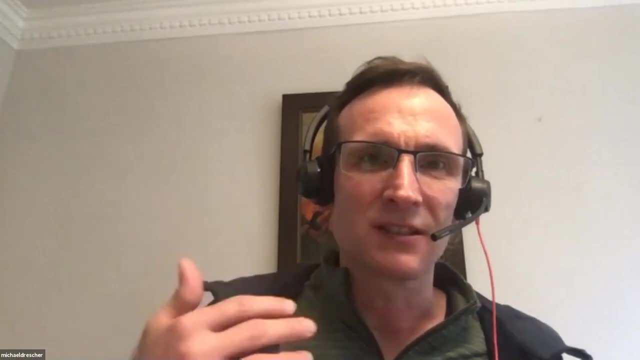 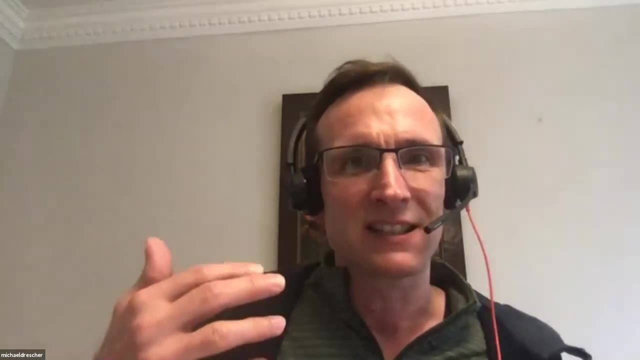 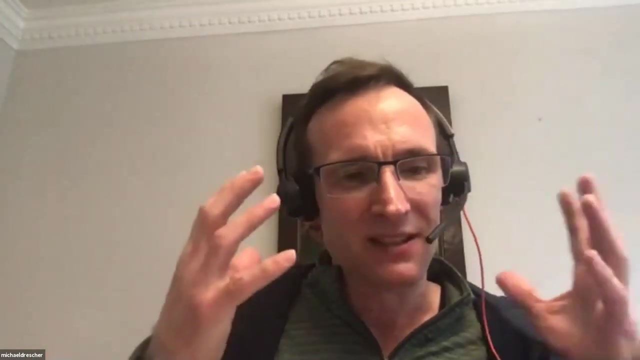 And then the government messaging to counter that is trust us, we know what we are doing. Well, if there's mistrust in government, then the government saying trust us is not going to help And there seems to be this amazing misunderstanding of what the problem is. 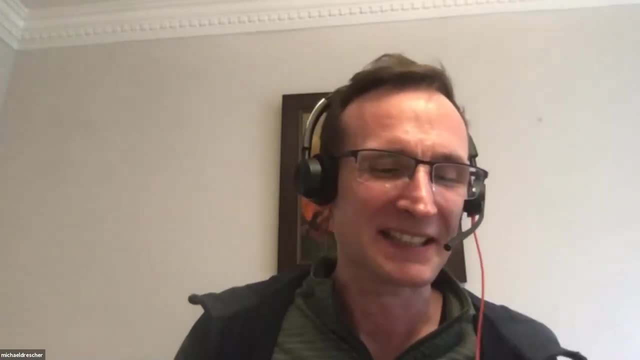 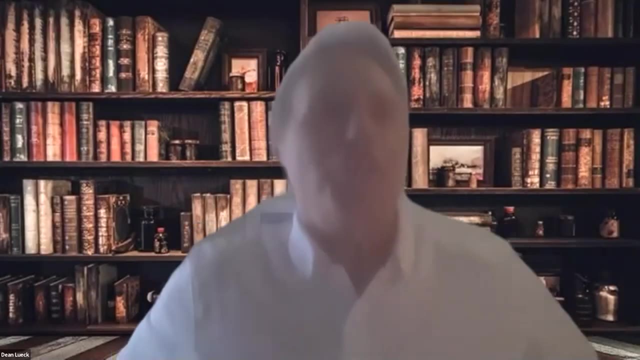 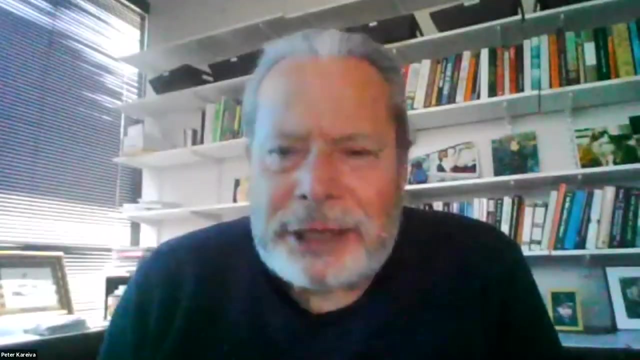 And I find it really, really it's mind boggling. Sorry, that's what I have, Peter. why don't you finish however you like and we'll just find Michael and Vicky, or however? So I mean, you know it's interesting. you say that, Michael, because that was the GMO problem. 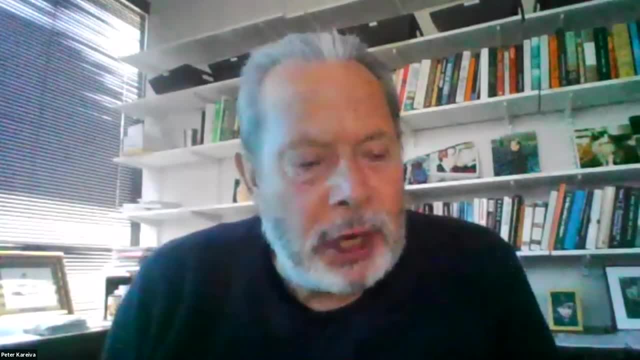 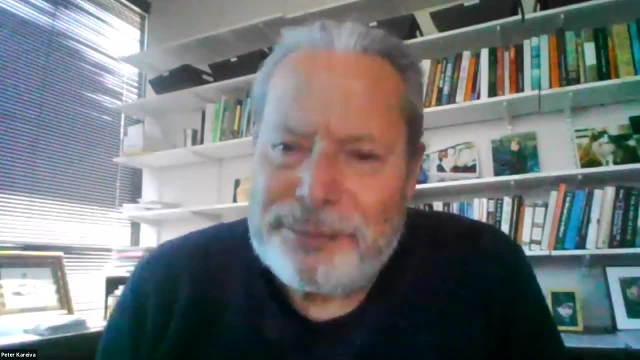 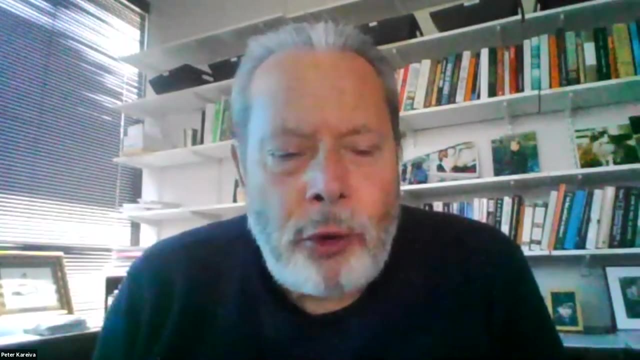 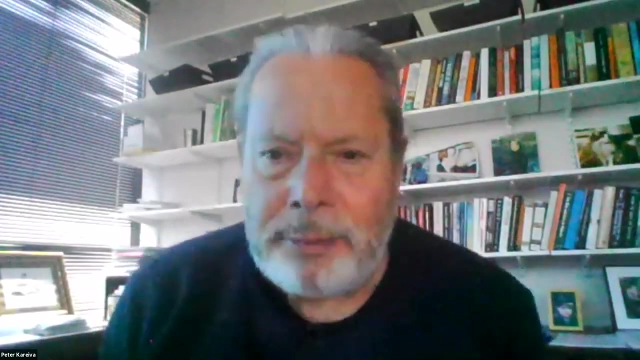 It was the molecular biologists, just absolutely ridiculed. I mean you know the patronizing problem. Remarks were pretty bad. I even made a. I shouldn't have done this. I took a quote from the president of the Anthropological Society of America about how DDT was nothing short of a miracle and magic.